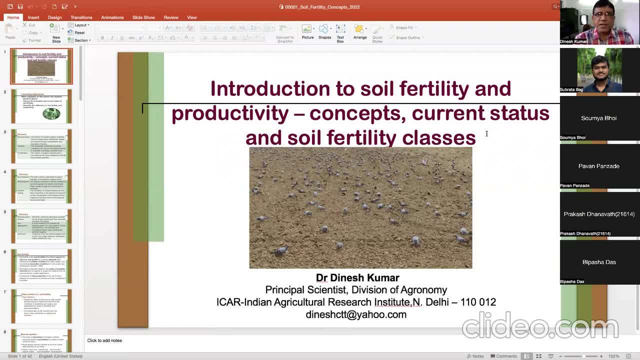 Anyone can come. There is no question of shame. Even if you are not correct, you are not right. I am there to correct you, But you should make attempt. This is the time to overcome your shyness. Come forward, Sir. soil fertility is the inherent ability of the soil to enhance plant growth by supplying nutrients. 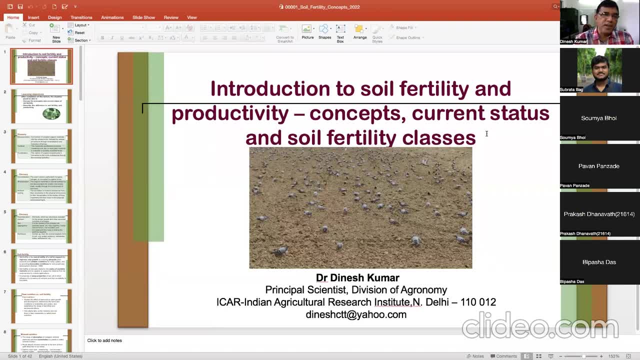 Very good. So see, very interestingly, she has not said just that soil fertility is the status of nutrients, of supplying the status of nutrients in soil, But she has also added, very interestingly, to improve the plant, to help the plant. 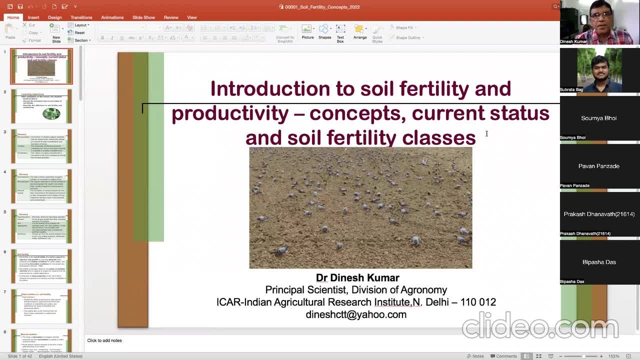 So this is quite interesting remarks by her. Any other definition of soil fertility, Because mostly people say it is the inherent capacity or ability of soil to supply nutrients in balanced and adequate amounts. But she has added another dimension, That is, to get the better plant growth. 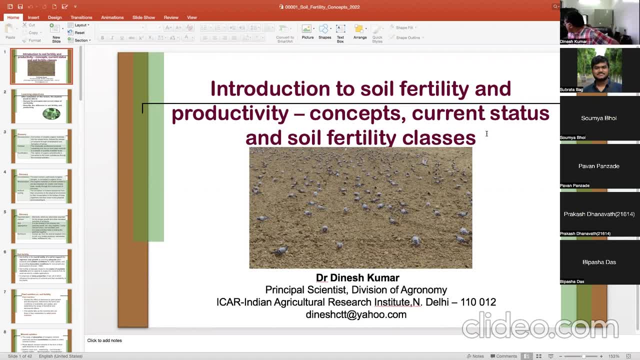 So any other definition of soil fertility, Hello sir? Yes, please. So the soil fertility can be defined as the ability of the soil to sustain the plant growth and development by providing the essential nutrients, like favorable chemical, physical and biological characteristics. Excellent, So actually, soil fertility is not just restricted to the status of nutrients. It includes something else also. 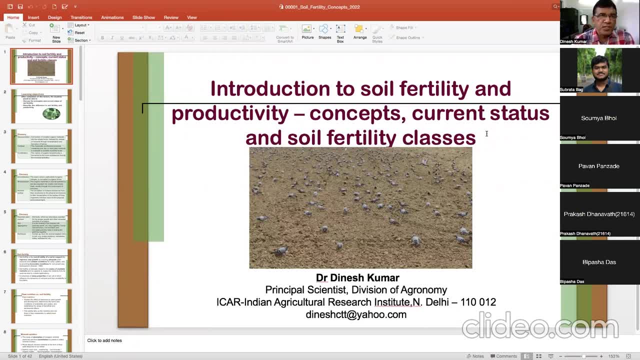 So I will show you definition of soil science: the Society of America in Swellfield. Next is your plant nutrition. What is plant nutrition and how we separate soil fertility from plant nutrition. Any idea, Come fast. Time is very limited, Hello sir. 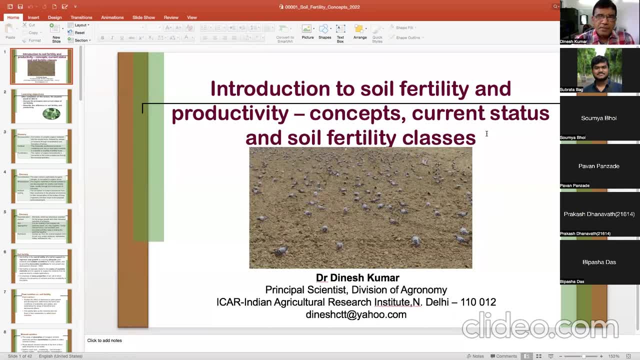 Yeah, Sir. plant nutrition is a broader concept Which includes availability of nutrients, their uptake and their accumulation, And this key process includes the total plant nutrition. Just a minute, Hello. Tell me quickly. So he has very directly pointed out what suggested definition of plant nutrition. 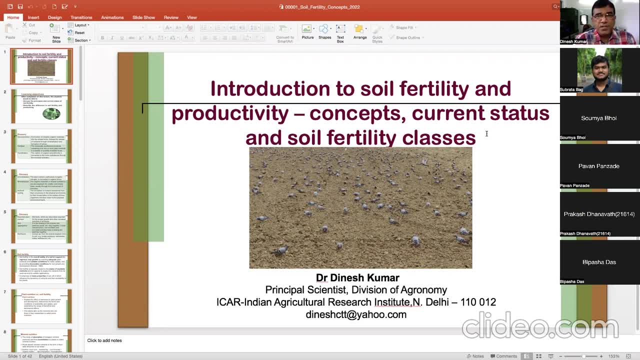 We will discuss it also. The next is mineral nutrition. So how plant nutrition is different from mineral nutrition, Because sometimes, you see, we write plant nutrition and sometimes we say mineral nutrition. Are they same or are they different? All right, Any difference in soil fertility and productivity? 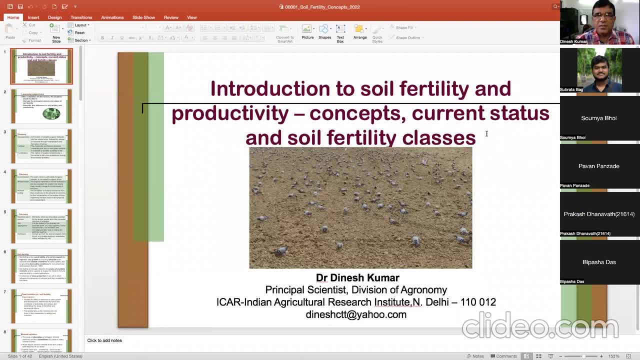 Yes, please. Any difference. Anybody knows the difference in soil fertility and productivity. Soil fertility is the capacity of the soil to supply nutrients for enhancing growth. Soil productivity is the ability of the soil to produce some crop in terms of hectare or in terms of yield. 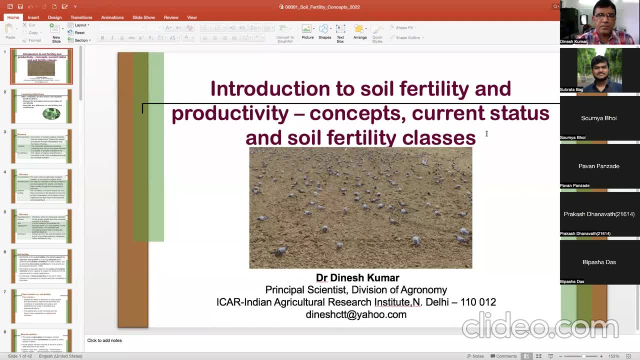 We can say that soil productivity is equal to soil fertility plus climate, plus management, Excellent, Excellent. So that is how we see differences And what should be the characteristics or ideal characteristics of a soil to be fertile, That, what are the things or what are the factors that will tell us that this particular soil is fertile and this particular soil is less fertile or low fertility. 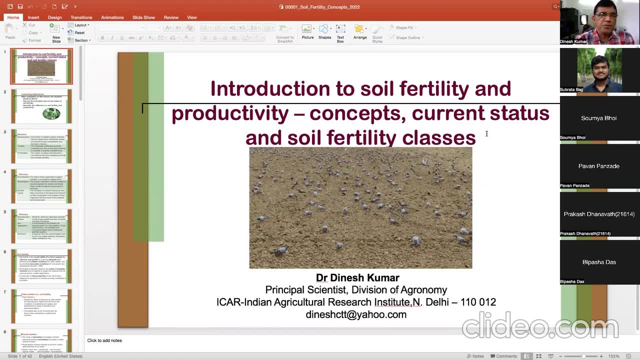 Having low fertility means how we can distinguish between soils of high fertility and low fertility. Just guess: By testing the soil nutrient contents like nitrogen, phosphorus and potassium. So it is just by seeing the nutrient status of the soil. But what about pH? What about CEC? What about soil structure? What about biological activities? 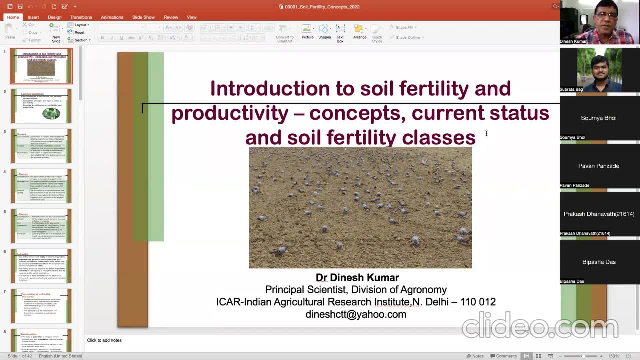 So it will also include, besides the chemical property like nutrient status, it will include many other factors Like soil depth and toxic things, soil pollution. You can find good status of nutrient in the soil, But if it is polluted by heavy metals, polluted by pesticides, 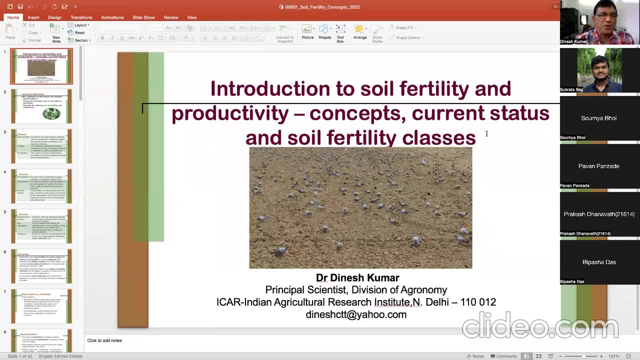 So you cannot call it fertile soil. So we need to look into other aspects also. We need to see the components of soil fertility. Next is: what are the principles of soil fertility? Anybody knows principles of soil fertility. So there are three principles of soil fertility. 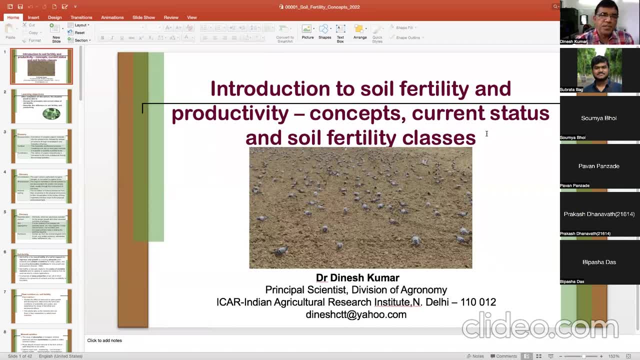 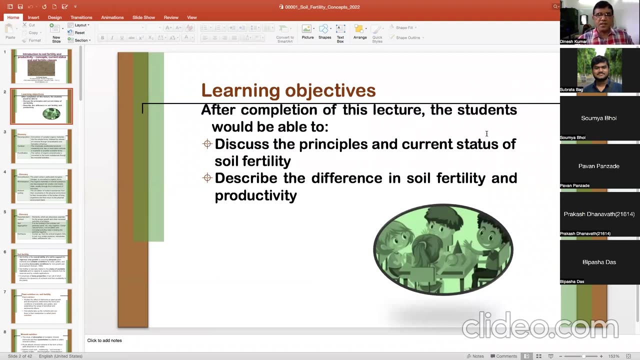 One is law of minimum, Other is principle of synchrony And third one is nutrient recycling or cycling. So these are three principles that we are going to discuss. So learning objectives are to discuss the principles and current status of fertility And describe the difference in fertility and productivity. 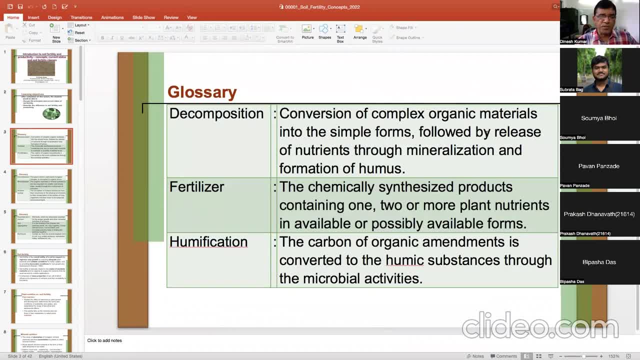 Some terminology. I think most of you know it, Just refreshing your memories: Decomposition- Conversion of complex organic materials into the simple forms, Followed by release of nutrients through mineralization and formation of humans- Means decomposition of organic matter. This is with respect to organic matter. 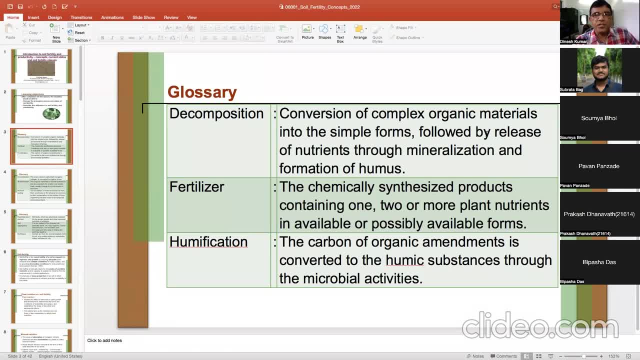 Means that something is made up of certain nutrients, Certain constituents, Certain compounds, Certain chemicals could make something, For example, organic matter. It will be made up of proteins, It will be made up of fats and lignin, Or proteins, carbohydrates, etc. 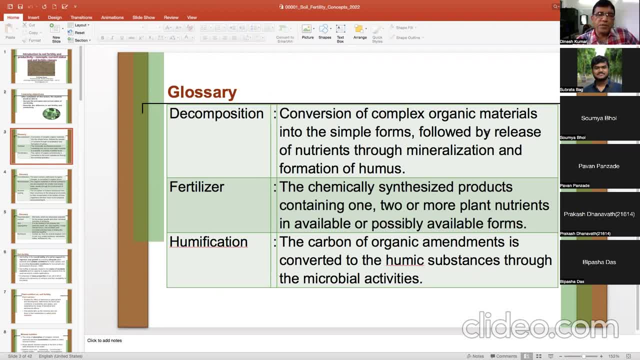 So this is the composition. And then, when you disintegrate it, When you degrade it, When you break it into different, similar compounds, That becomes your decomposition. Fertilizer is chemically synthesized products Containing one, two or more plant materials. 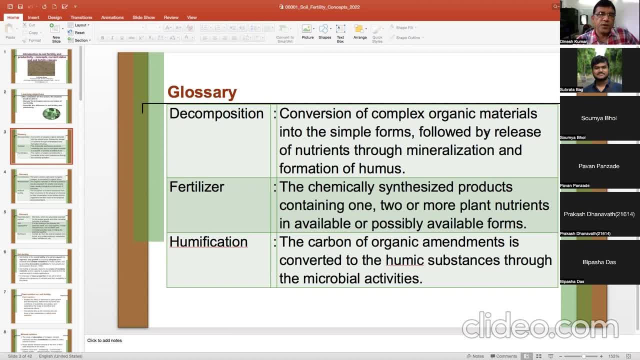 Humification is simply formation of humans Or production of humans after decomposition of organic matter And when organic matter decomposes. There are two major pathways which are happening in organic matter decomposition. One is humification, Other is mineralization. They go hand in hand. 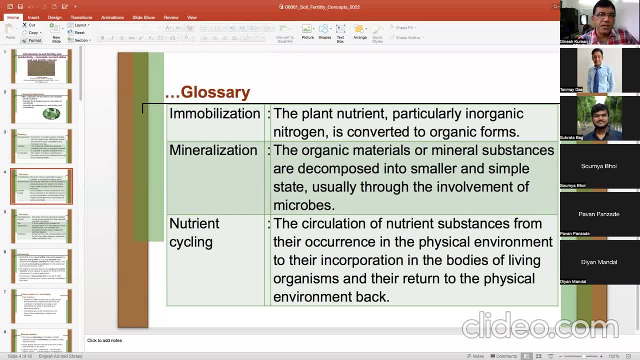 Next term is immobilization, When organic matter decompose, Particularly when you have higher CN ratio, And that time microbes consume the available nitrogen From the soil- Mainly nitrogen- And then there is shortage of nitrogen at that time. So this conversion of available nitrogen into unavailable nitrogen- 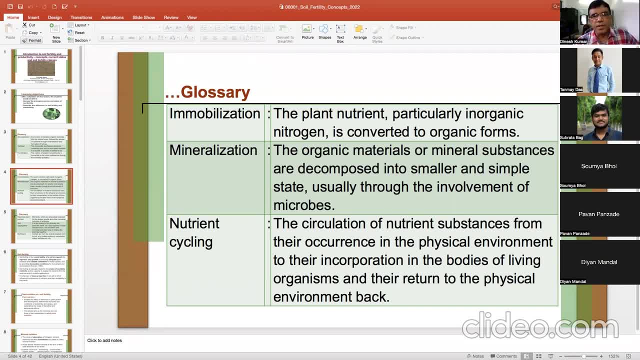 In the form of Nitrogen is taken up by microbes, Is your immobilization. It is also called as microbial immobilization, Mineralization, when you have organic matter And when it played down into different pieces. So there are two pathways. One is humification. 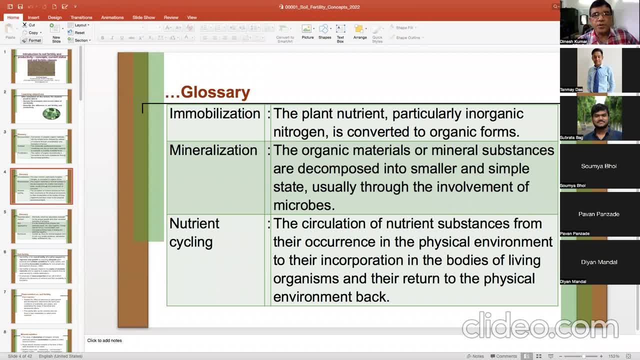 Other is mineralization. So mineralization, Decomposition of organic matter, Results in production of certain minerals. Or you can say: when you have organic matter, If you burn it. If you burn it It will be oxidized And carbon. 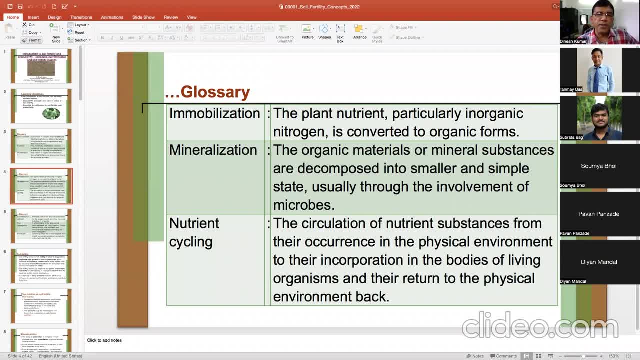 And hydrogen And oxygen will be liberated. They will go away, And what left is your ash. And ash contains all the minerals. Ash contains all the minerals, Of course, during burning, Some of the nitrogen And some of the sulfur And some of the phosphorus. 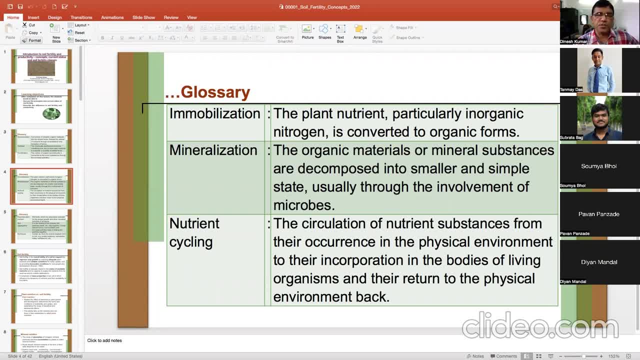 They also get away. They are also lost partly. So whatever is left in the ash Are your minerals, And that is done by fire. Similarly, it can be done by oxidation Involving microbes. So that is your mineralization, Part of decomposition. 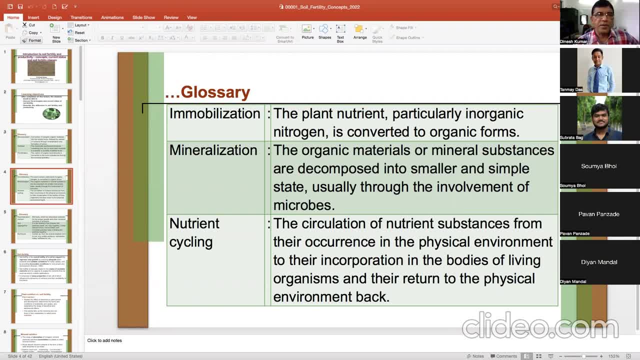 Where minerals are released. Nutrient cycling. Nutrient cycling is just circulation of minerals. Circulation of minerals Through the terrestrial system, Through the water system And so on. Nutrients: You can see it: The circulation of nutrient substances from their occurrence in the physical environment. 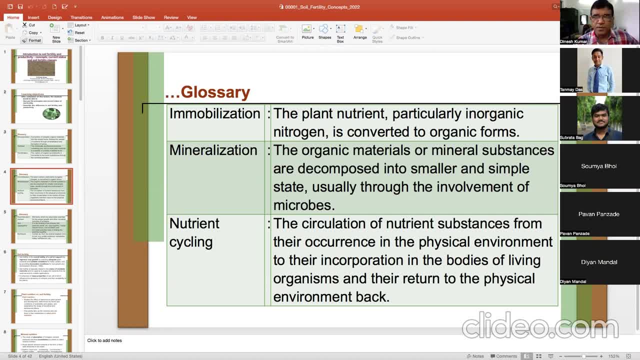 To their incorporation in the bodies of living organisms And their return to the physical environment there. When they recycle, When they change their materials, Change their are in X. tomorrow they will be in Y- Essential plant nutrients. you know it: Soil aggregation. 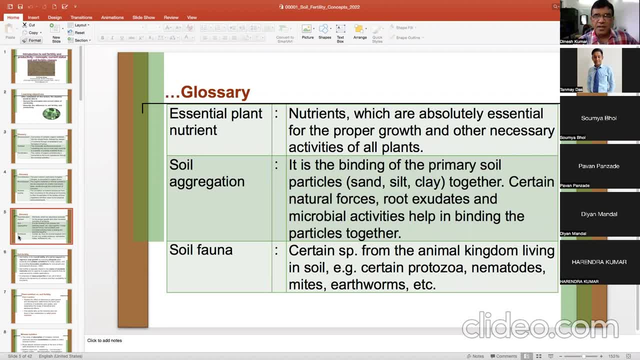 is binding of the primary soil particles. Aggregation means making small, small clots of sand-silk clay together. Certain natural forces and root exudates and microbial activity help in binding the particles together. This is important. Certain natural forces, or maybe? 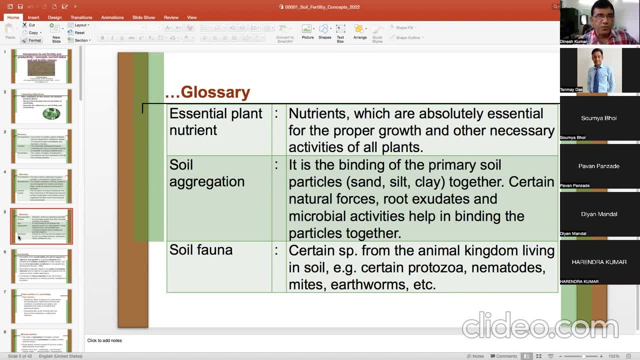 some attraction, chemical attraction, root exudates and microbial activities. Certain fungi release some material that can bind the particle together. Other microbes also release some organic materials that can bind the particle together. And other role is played by humus. Humus is very important in soil aggregation. It helps in binding the clay. 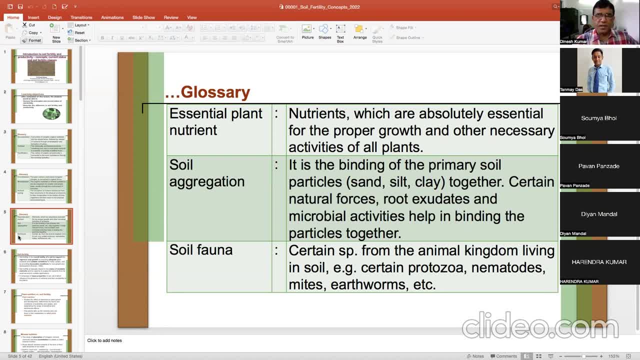 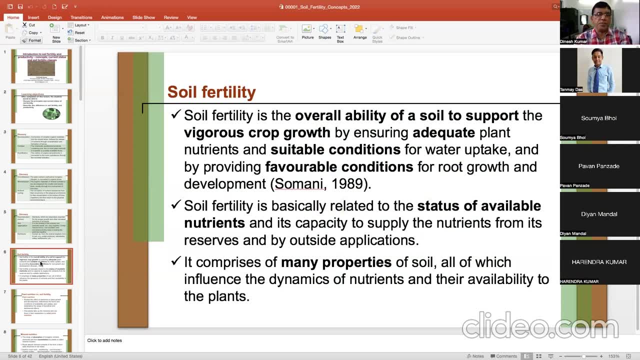 particles are certain species from the animal kingdom living in soil, certain protozoa, nematodes, mites, earthworms, etc. Now we come to the main topic, that is, soil fertility. So Somani in 1989 gave this definition: Soil fertility is the overall ability of the soil to support 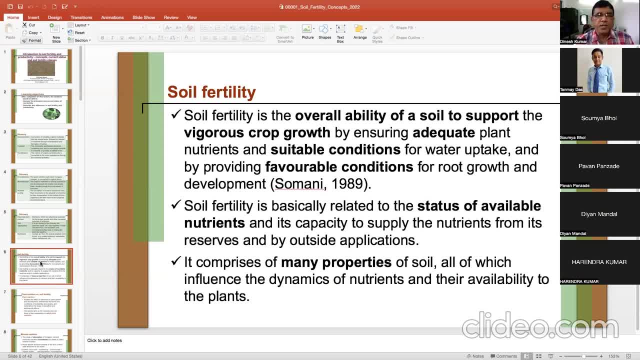 the vigorous crop growth, as pointed out by you. So here growth is also important that it should in. in theory, it should support the vigorous crop growth by ensuring adequate plant nutrients and suitable conditions for water uptake Without, because without water availability and uptake, the nutrients cannot be taken up. So this the soil should be able. 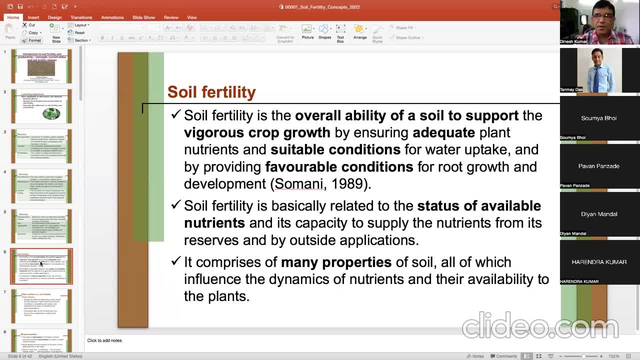 to supply the nutrients. But it is possible when you have required water and water uptake conditions are good, and by providing favorable conditions for root growth, Because without root also your nutrients cannot be taken up by plants and developed. so this is perhaps very good definition. soil fertility is the overall ability of the soil to support the 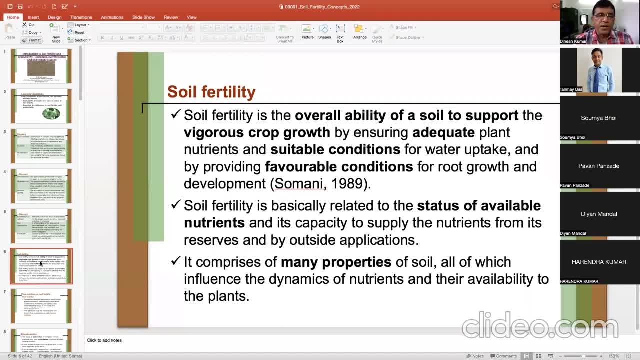 vigorous growth growth by ensuring adequate plant nutrients and suitable conditions for water uptake and by providing favorable conditions for root growth and development. so this is complete definition of fertility. however, other definitions, like soil fertility, is basically related to the status of available nutrients and its capacity to supply the nutrients. 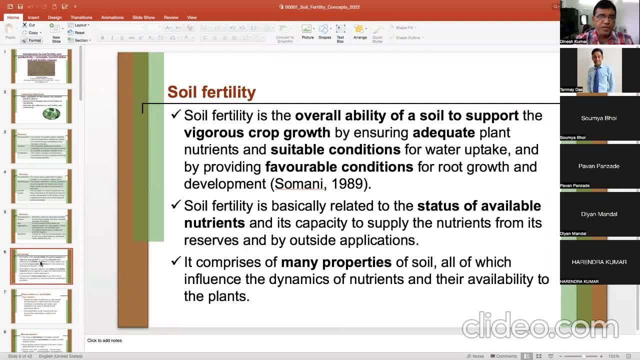 status and capacities to supply the nutrients from in reserves and by outside application. so nutrients can come through the reserve and through the outside applications. that is soil fertility. so this definition is brief and and it can be remembered easily. also, though it is not complete, other is comprises of many properties of soil. so here you can see soil fertility has been broken into. 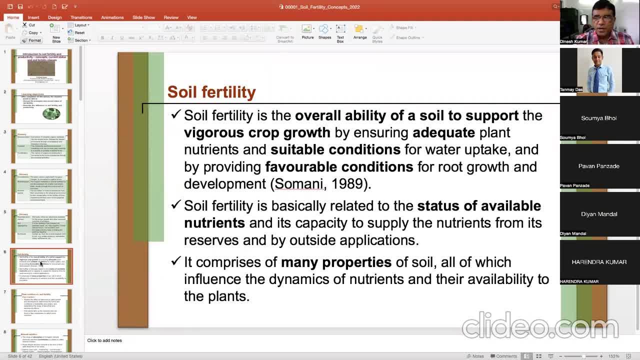 properties. so it comprises of many properties of soil, all of which influence the dynamics of nutrients, dynamics of nutrients and their availability to the plant. so you can see, in this definition, it is not just a status of nutrients which is called less fertility. you can see, in this case there are many other things, many other things. 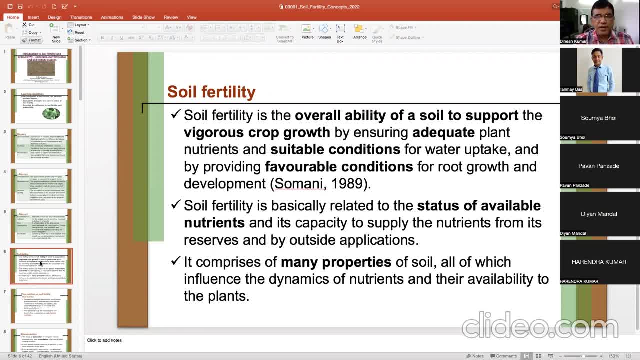 many more things other than the nutrients which are part of hydrology and that can influence the availability of the nutrients. for example, aeration will surely affect the availability of the nutrients, similarly water content, similarly soil structure and faces, soil fatigue. there are many other things which are component of soil fertility we need to discuss. 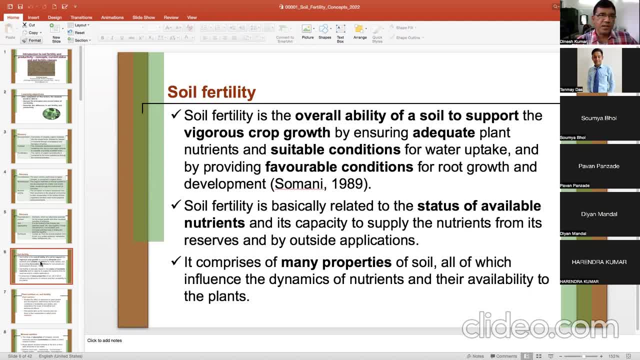 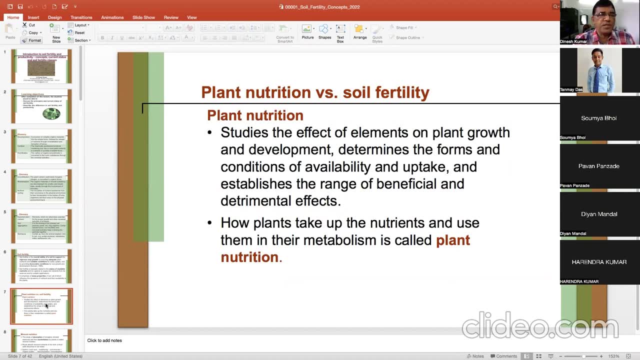 so if you are not able to understand anything what i discussed, You can stop me there, right there, and we can clarify it. So it should be two way interaction Now: plant nutrition versus soil fertility. So, soil fertility, you have just now seen. 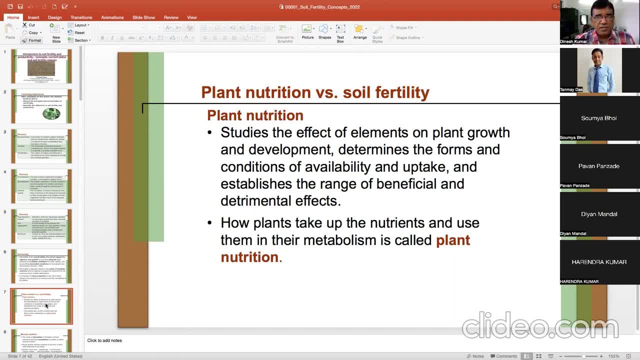 And plant nutrition is the subject. it starts where the fertility ends. You have seen that in soil fertility, the status of nutrients and supplying capacity of the soil, supplying capacity of the nutrients of the soil to the plants. So that is soil fertility. 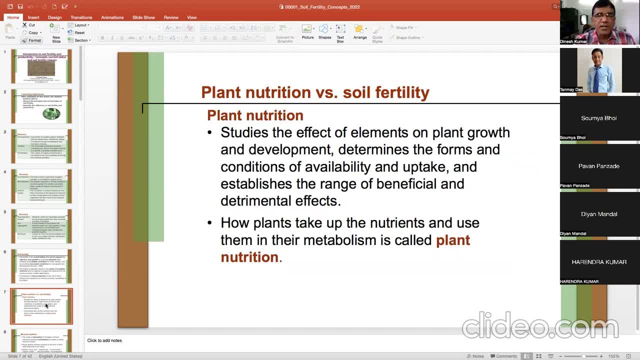 And then comes your uptake. soil fertility can make the nutrients available. Then after that plant will take up the nutrient. it is part of plant nutrition means uptake of nutrient, then translocation of nutrients in the plant system, then further synthesis of the nutrient. 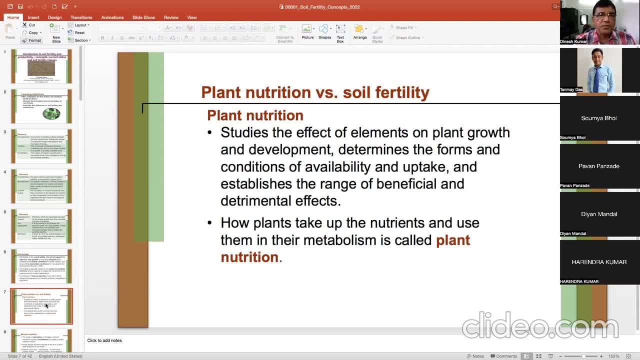 And it will be playing a number of roles. So we need to study uptake, translocation, assimilation and then role of the nutrient in the plant, And then deficiency symptoms or toxicity symptoms. All these subjects are part of plant nutrition. I think they are complementing each other. 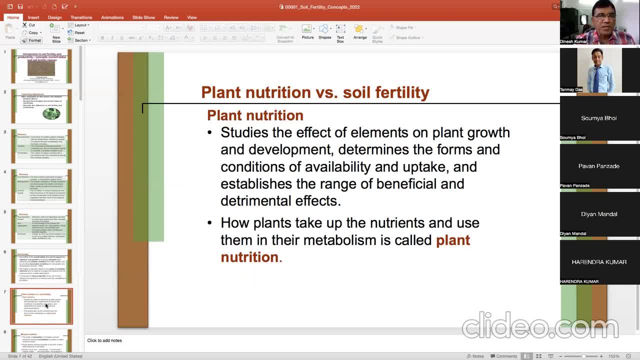 So first, soil fertility, it will supply the nutrients, and then comes your plant nutrition, which will help in taking care of the nutrients. Okay, So it will be taking care of the nutrients from the soil and then translocation, assimilation, and then, if they are deficient, what are the symptoms? what are the roles of nutrients? 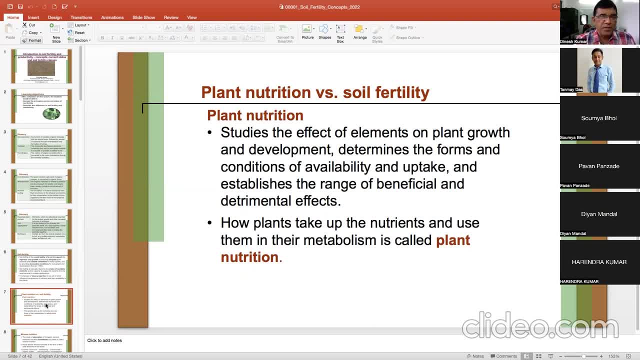 So that makes part of your plant nutrition. So it studies the effect of elements on plant growth and development, determines the forms and condition of availability and uptake and establishes the range of beneficial and detrimental effects. So this is plant growth and development, Plant nutrition. 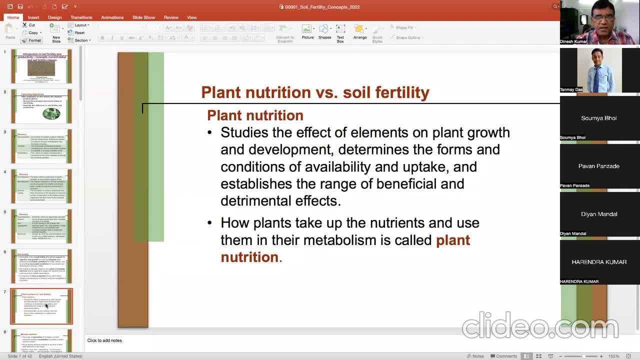 In simpler words, how plants take up the nutrients and use them in their metabolism is called as plant nutrition. So you can have a variety of definitions, but you can remember very easily that after soil fertility the subject of plant nutrition starts: uptake, translocation, assimilation. 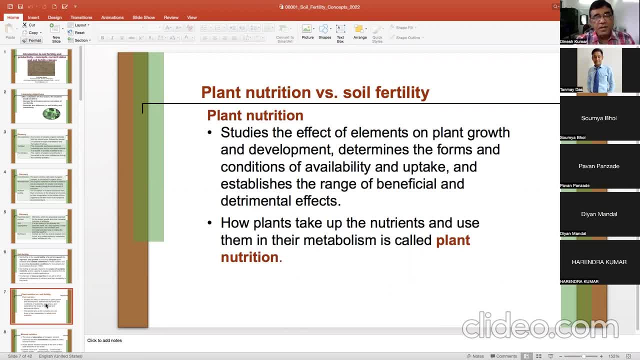 and different roles and deficiency symptoms. Next comes the mineral nutrition. So plant nutrition includes all the. So how many elements are essential for plant growth? How many elements are essential for plant growth? 70.. How many 70.. 70.. 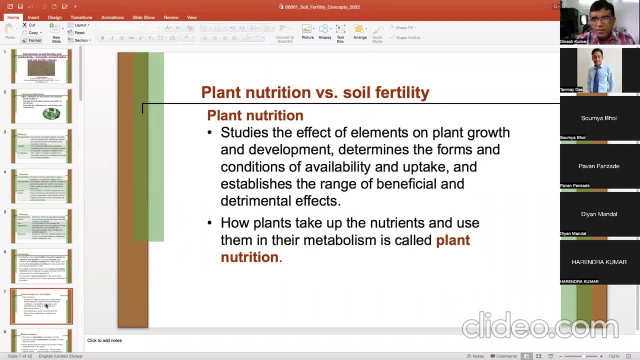 Yeah, So in 17,. carbon, hydrogen and oxygen: these three important nutrients are considered as framework element. That make the major framework element Okay. So what is the major framework of plants? Because carbon can be 40 to 45%, oxygen can be 40 to 45% and hydrogen can be 5 to 8%. 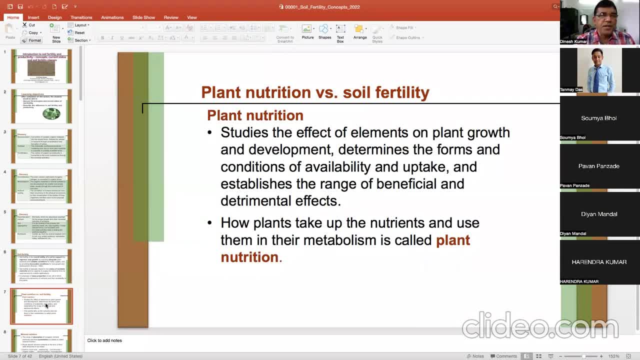 So you can see about 94,, 94,- 95% plant is carbon hydrogen and oxygen. But we do not normally talk about carbon hydrogen and oxygen nutrition to the plant because these elements plants are getting from the nature in the natural form. 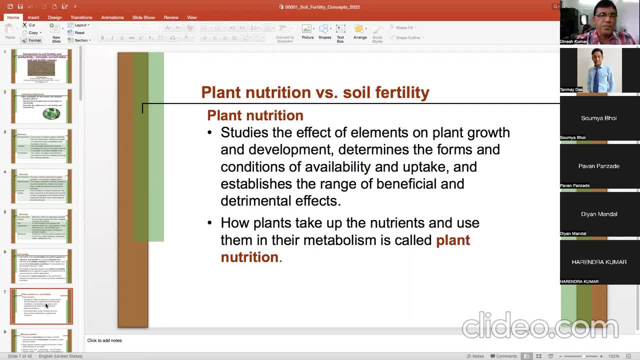 So human being is not feeding plants. hydrogen: Human being is not feeding plants. oxygen, And so is the case of carbon. Carbon is coming as CO2, hydrogen from water and oxygen from water and carbon dioxide, So there is no need for any nutrition. 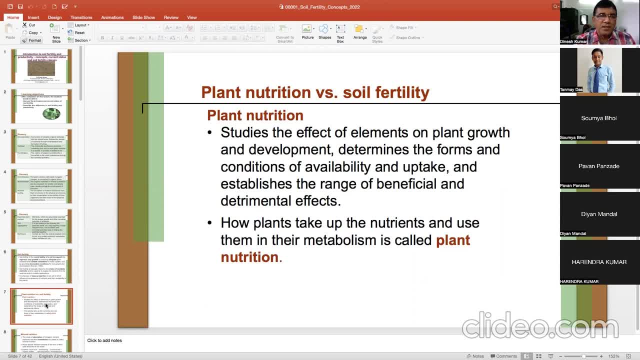 So plant nutrition includes all the 17 elements. Okay, So there are 17 essential nutrients, including carbon, hydrogen and oxygen. However, mineral nutrition includes your 17, minus carbon hydrogen and oxygen. where mineral nutrition is studied, These nutrients are taken up in ionic form by the plants. 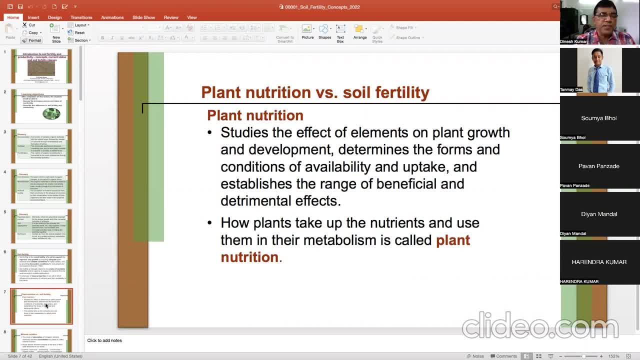 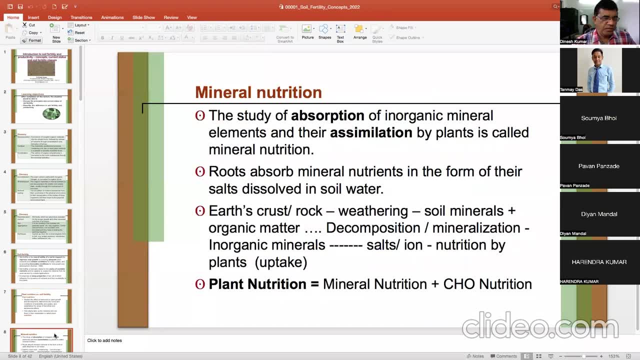 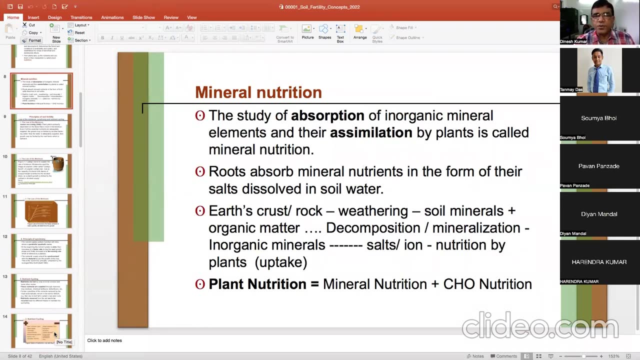 Those kinds of studies are the subject of mineral nutrition, which exclude carbon hydrogen and oxygen. Okay, Okay Now the study, mineral nutrition, is the study of absorption of inorganic mineral elements. inorganic mineral elements and their assimilation by plants is your mineral nutrition. 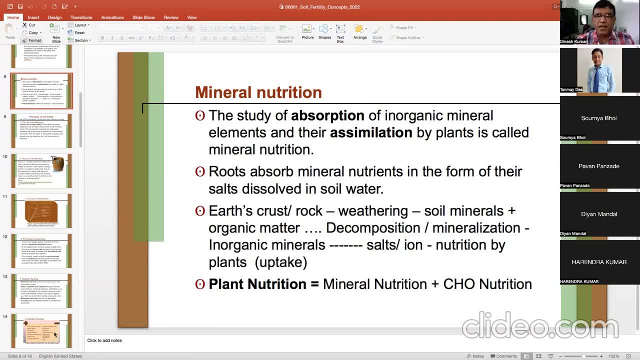 Roots absorb mineral nutrients in the form of their salts dissolved in soil water. That is another reason that it is called as mineral nutrients, because nutrients are removed as ions, But they are kind of soluble Earth's crust. and another thing: how these minerals come. 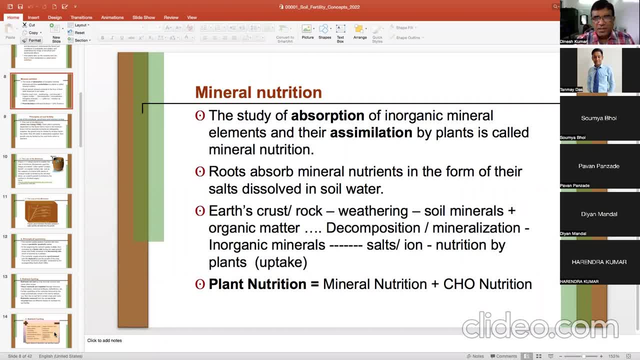 Earth's crust or rope. you know the weathering process. you understand Physical, chemical, biological weathering is there, from which the rope material is converted into soil, And then soil minerals are released. after the weathering, They are held by organic matter to make soil. 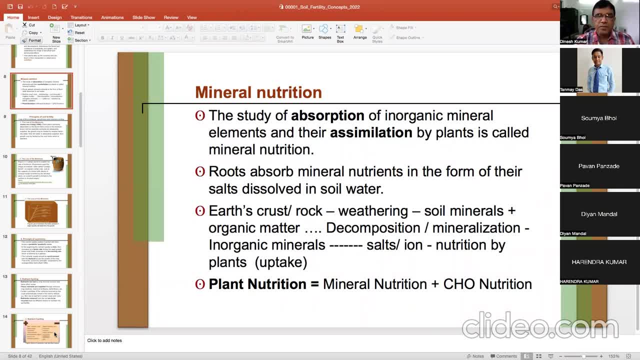 Decomposition can happen. Decomposition and mineralization can happen for this organic matter or even for mineral. Minerals can be further mineralized into simpler forms like your ionic forms, And these are taken up by plants. So you can see, plant nutrition is called mineral nutrition, plus CHO, carbon, hydrogen oxygen. 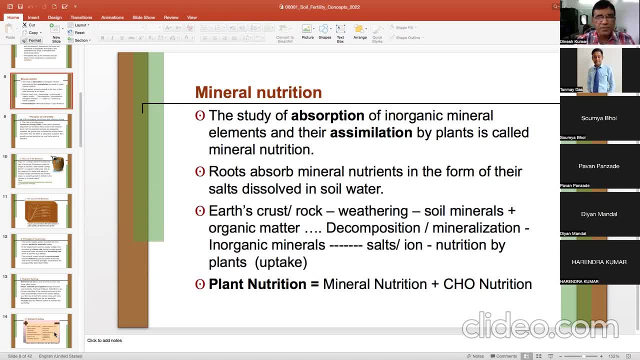 nutrition. Any question, any doubt up to now? Okay, Any point of discussion? Pawan, Sir, I think there are three components of mineral nutrition, like absorption, transcription and assimilation. Yeah, That is right, Sir. Yeah, 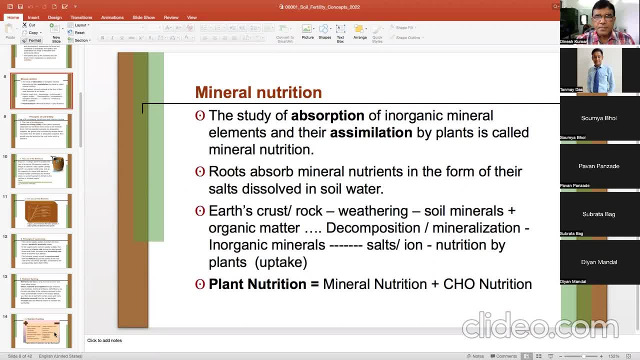 Yes, yes, Speak Tanmay Sir. that's all, sir. Three components of mineral nutrition. Yeah, That is right. Yeah, Yes, yes, Speak Tanmay Sir. that's all, sir. Three components of mineral nutrition. 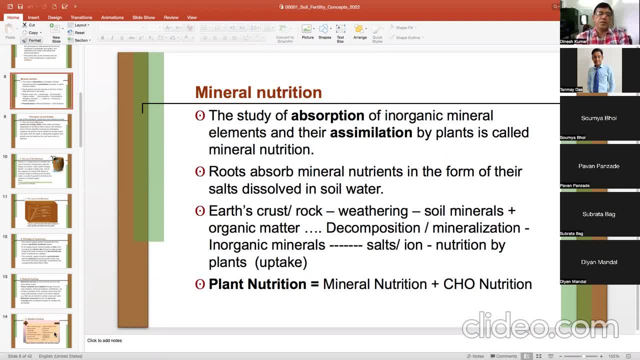 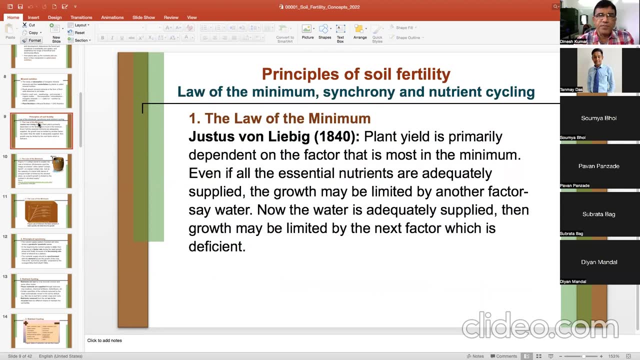 Yeah, Yeah, This is true. This is true. Mineral nutrition or plant nutrition? in this case it is absorption, transcription and assimilation. Fine, Now we go to principles of soil fertility. What are the fundamental principles of soil fertility maintenance? 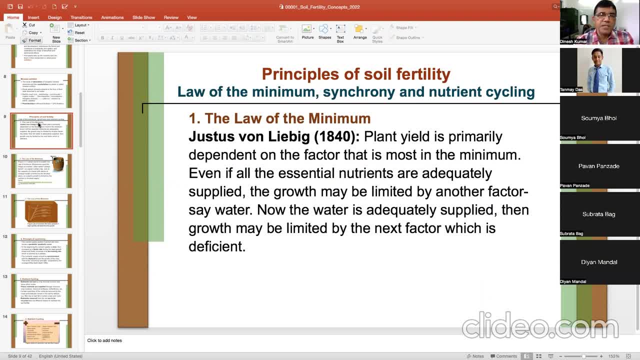 What should be considered as basic principles of soil fertility. First is law of the minimums, Other is law of synchrony and law of nutrient cycle. These are basic or fundamental things to soil fertility maintenance. Law of minimums: it says that all the nutrients should be present in balanced amount or at 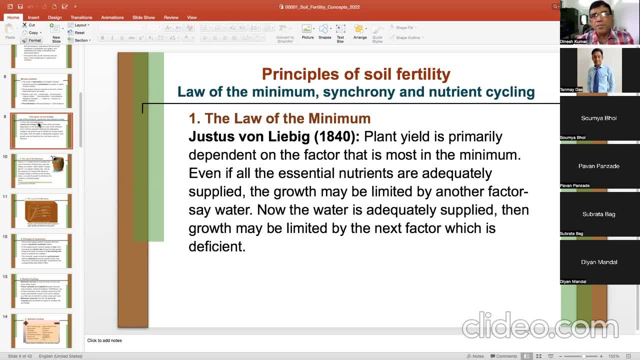 least some minimum quantity or lowest quantity of a nutrient should be present in the soil. That is good also for maintenance of soil fertility. if one element is missing or is not present in the soil or is in less concentration, it can affect the uptake of other nutrients. so therefore, first, 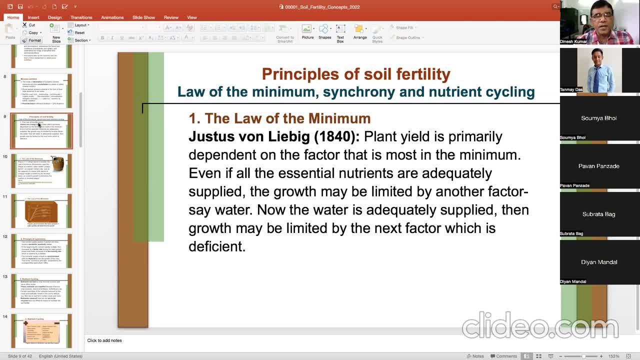 principle is that all the nutrients should be there in the balanced ratios in the soil and right amount. so love, minimum help in knowing that. so that is why it is principle of self-reliance. another is principle of synchrony. whatever nutrients are there in the soil, suppose at 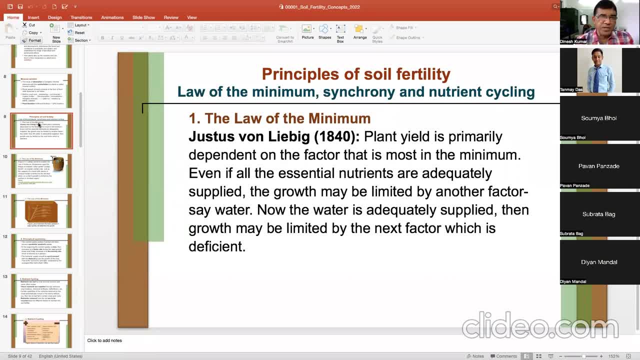 the time of sowing, there are large number of nutrients, large amount of nutrients. but at that time, because plant is in seedling stage, it cannot take up the amount of nutrients that is available in soil. so what will happen then? some of the nutrients will be lost and plant will not use it. 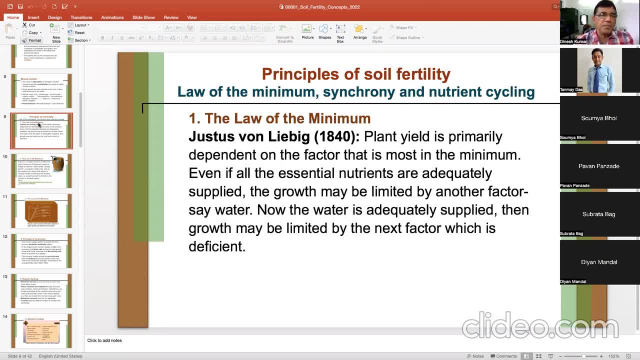 but what happens? that in the beginning, suppose we don't apply nitrogen in the beginning, that is fine and we can apply it later, later, later, later, later, later. and requirement of requirement of nitrogen is small in rice, we can apply it with a tilling, we can apply it with a panicle, initiation stage. so we must synchronize the availability or supply of 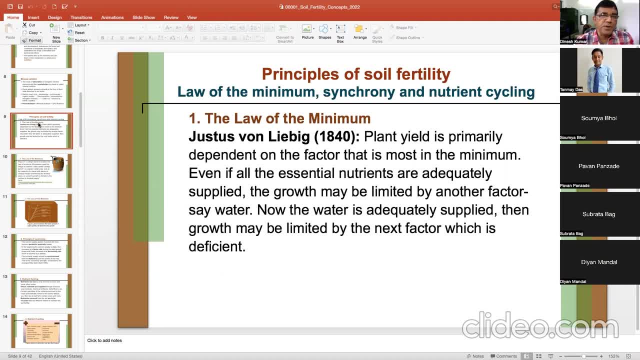 the nutrient to the requirement requirement. when requirement is more, our soil should have more nutrients and otherwise, when requirement is less, there should be less status of nutrient. and that can be manipulated by external application of fertilizers or manure. and that can be manipulated by external application of fertilizers or manure. 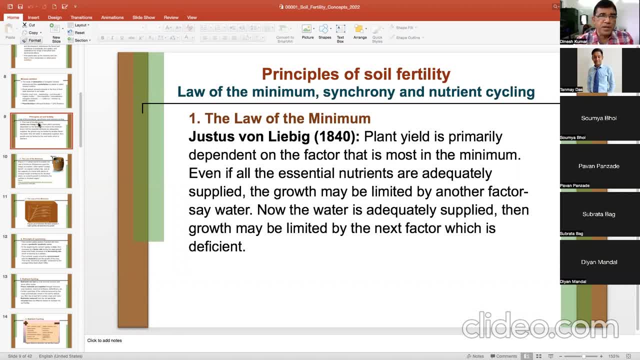 and that can be manipulated by external application of fertilizers or manure. so, but this is, this becomes important. principle of soil fertility, principle of synchrony. so, but this is, this becomes important. principle of soil fertility, principle of synchrony. so, but this is, this becomes important. principle of soil fertility, principle of synchrony, and then principles of nutrient cycling. 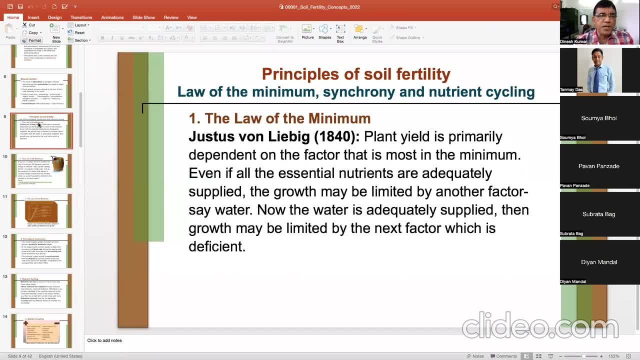 and then principles of nutrient cycling, and then principles of nutrient cycling. it is not, as always, desirable that whatever it is not, as always, desirable that whatever. it is not, as always, desirable that whatever nutrients have been removed from the soil, nutrients have been removed from the soil, nutrients have been removed from the soil, and all should be supplied through fertilizers. 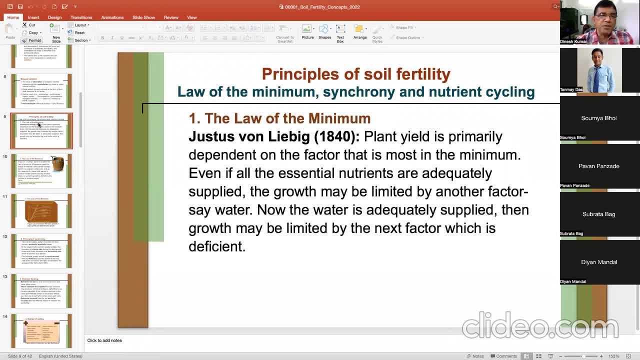 and all should be supplied through fertilizers and all should be supplied through fertilizers. that is never necessary, because some of the that is never necessary, because some of the that is never necessary, because some of the nutrients which have been removed from the nutrients which have been removed from the 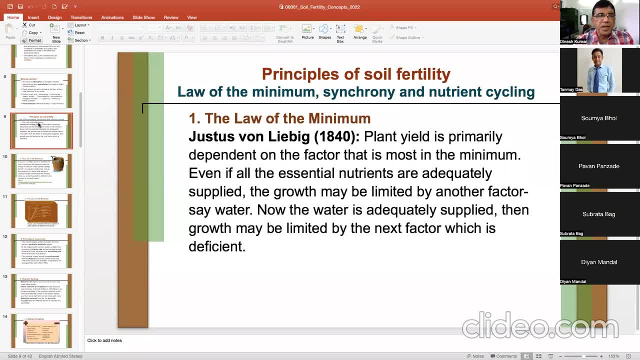 nutrients which have been removed from the soil into the plant parts. some of them should soil into the plant parts. some of them should soil into the plant parts. some of them should be returned to the soil. be returned to the soil. be returned to the soil just to supplement the fertilizers. so 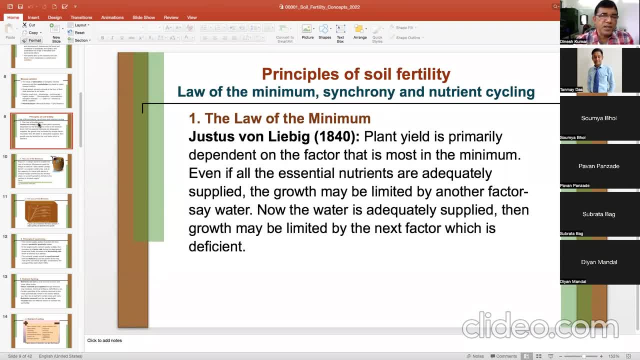 just to supplement the fertilizers, so just to supplement the fertilizers. so therefore cycling is very, very important. therefore, cycling is very, very important. therefore cycling is very, very important. at least insta can be cycled, at least if. at least insta can be cycled, at least if. 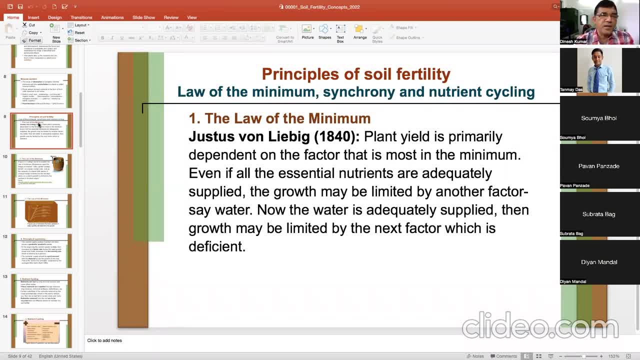 at least insta can be cycled at least. if you feed fodder to the animals, you feed fodder to the animals, you feed fodder to the animals, and then their tongue can make your, and then their tongue can make your, and then their tongue can make your compost or farm yard manure, that should. 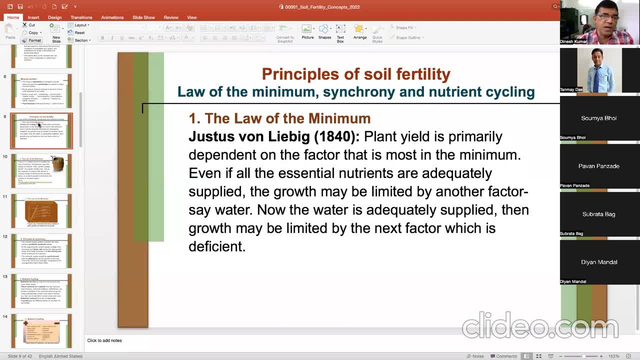 compost or farm yard manure that should compost, or farm yard manure that should be returned back to the soil, so nutrient be returned back to the soil. so nutrient be returned back to the soil, so nutrient cycling should happen. that is also a. cycling should happen. that is also a. 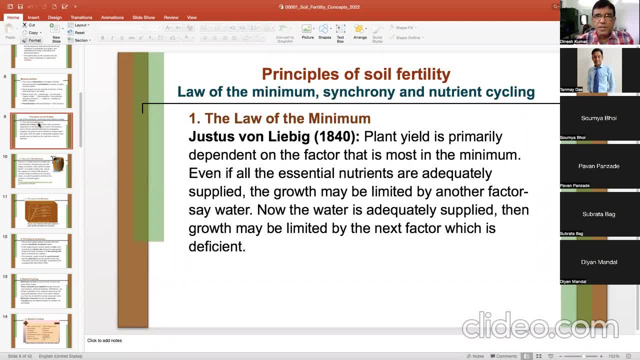 cycling should happen. that is also a principle of soil filter. if we principle of soil filter, if we principle of soil filter, if we adopt these three principles, then we can adopt these three principles, then we can adopt these three principles, then we can sustain about sustain, about sustain, about fertility and productivity. so, law of 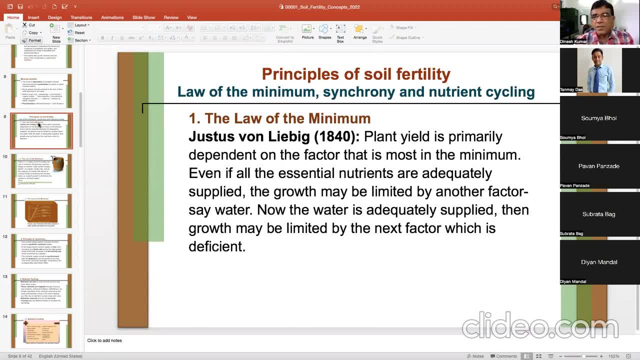 fertility and productivity. so law of fertility and productivity, so law of minimum law of synchronicity and nutrient minimum law of synchronicity and nutrient minimum law of synchronicity and nutrient cycle cycle cycle are the three laws of soil fertility, are the three laws of soil fertility, are the three laws of soil fertility, and you will not find these laws in any. 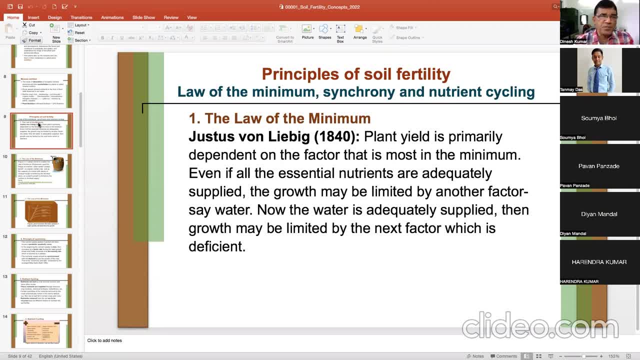 and you will not find these laws in any, and you will not find these laws in any book, book, book. if any student come across, if any student come across, if any student come across that he has found these principles of that. he has found these principles of that, he has found these principles of soil fertility. 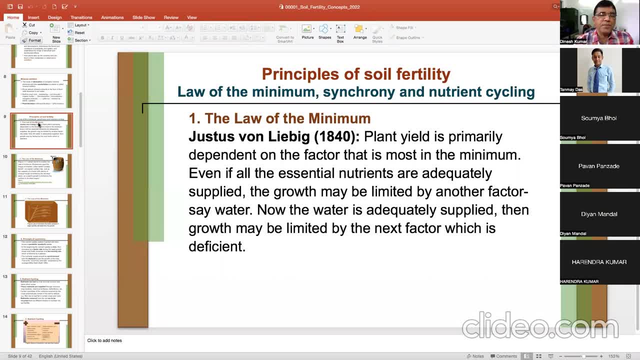 soil fertility, soil fertility. written in any book, written in any book, written in any book. you will not find, you will not find, you will not find. but you can find only in one book, but you can find only in one book, but you can find only in one book. i will share, uh, that chapter. 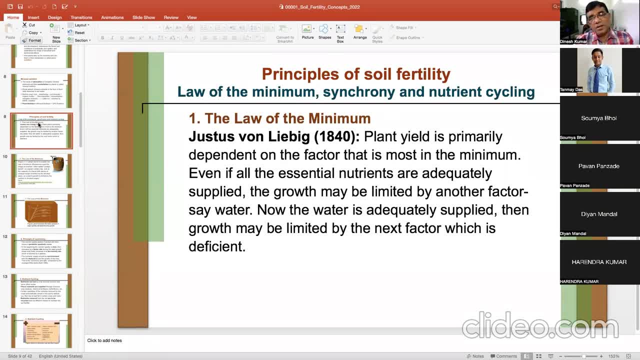 i will share uh that chapter. i will share uh that chapter with you. principles of soil fertility, with you, principles of soil fertility, with you, principles of soil fertility. so so so uh references are not available, but uh references are not available. but uh references are not available. but separately you can find. 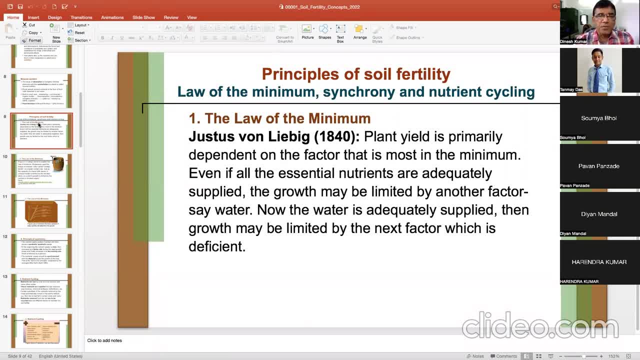 uh references are not available, but separately you can find uh references are not available, but separately you can find love minimum synchrony, love minimum synchrony, love minimum synchrony. so you can see the love minimum, so you can see the love minimum, so you can see the love minimum and many of you might be knowing that it 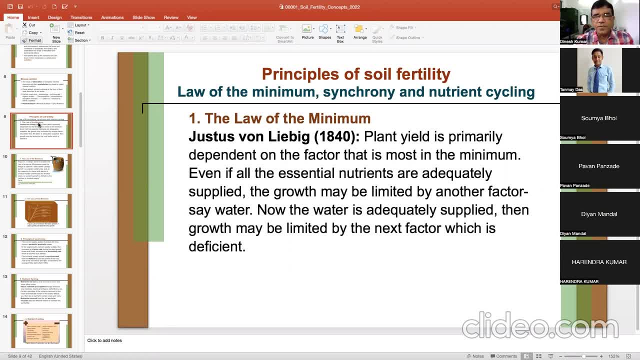 and many of you might be knowing that it, and many of you might be knowing that it was proposed by. was proposed by: was proposed by: justice born living 1840. justice born living 1840. justice born living 1840. what did he say? that plant yield is. 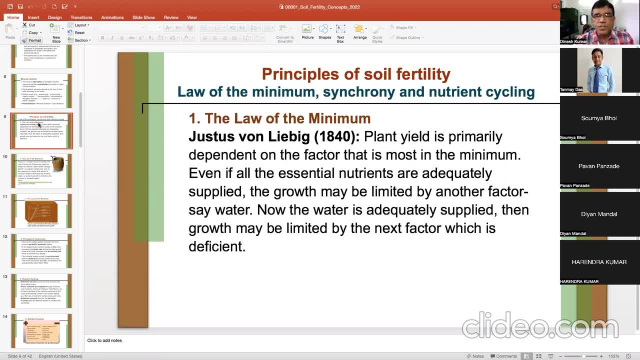 what did he say? that plant yield is. what did he say? that plant yield is primarily dependent on the factor, primarily dependent on the factor, primarily dependent on the factor that is most in the middle. that is most in the middle. that is most in the middle means most the lowest quantity of the 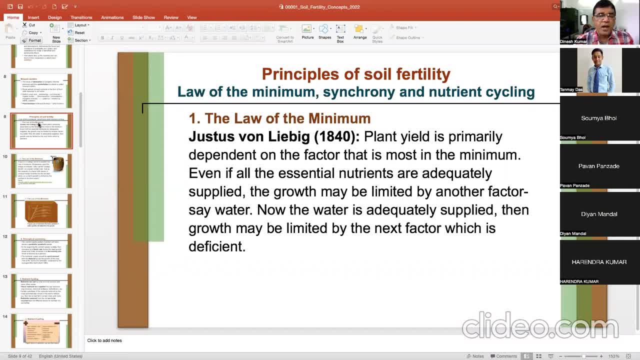 means most the lowest quantity of the means most the lowest quantity of the factor. even if all the essential factor, even if all the essential factor, even if all the essential nutrients are adequately supplied, the nutrients are adequately supplied. the nutrients are adequately supplied. the growth may be limited by another factor. 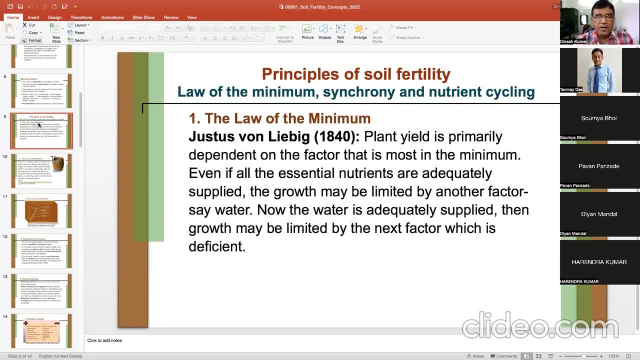 growth may be limited by another factor. growth may be limited by another factor. say water, say water, say water. now the water is adequately supplied. that now the water is adequately supplied, that now the water is adequately supplied, that growth may be limited by the next factor. growth may be limited by the next factor. 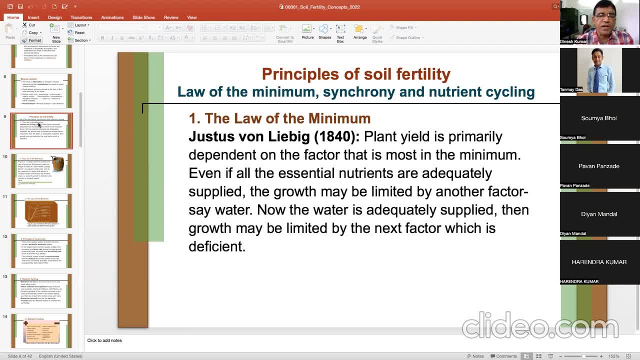 growth may be limited by the next factor: which is deficient, which is deficient, which is deficient. so the law of minimum can be defined in. so the law of minimum can be defined in. so the law of minimum can be defined in many ways, many ways, many ways. first, you can define it in factors. 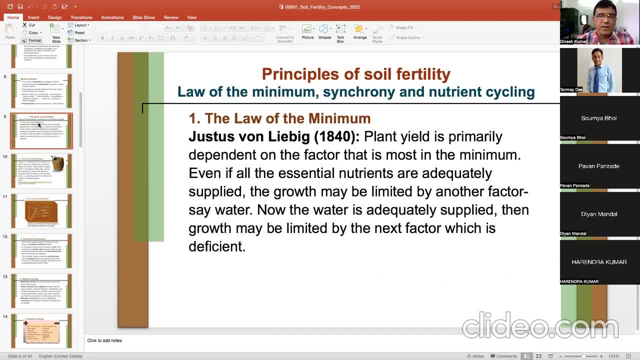 first you can define it in factors. first you can define it in factors affecting plant growth, in that sense affecting plant growth, in that sense affecting plant growth, in that sense also you can define it, and you can also, also, you can define it, and you can also also, you can define it and you can also, if you consider just new, different. 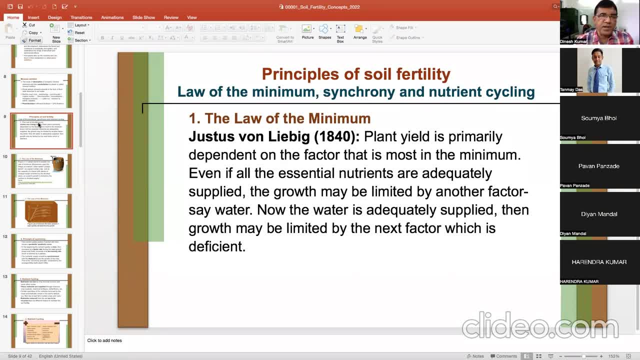 if you consider just new, different, if you consider just new, different nutrients, nutrients, nutrients as factors, different nutrients as factor as factors, different nutrients as factor as factors, different nutrients as factor of growth, then also you can define of growth, then also you can define of growth, then also you can define this law. but this is mostly restricted. 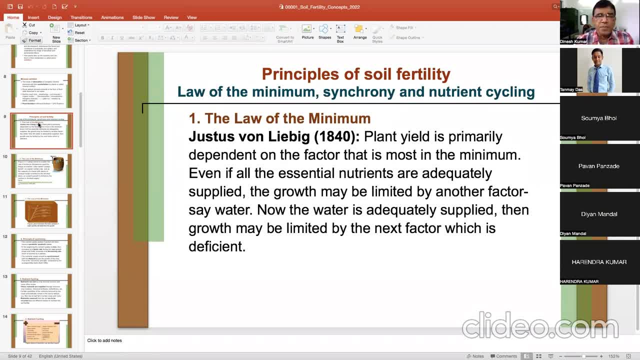 this law, but this is mostly restricted this law, but this is mostly restricted to the nutrients. there are 17 essential to the nutrients. there are 17 essential to the nutrients. there are 17 essential nutrients: nutrients, nutrients and carbon hydrogen oxygen. you need not and carbon hydrogen oxygen. you need not. 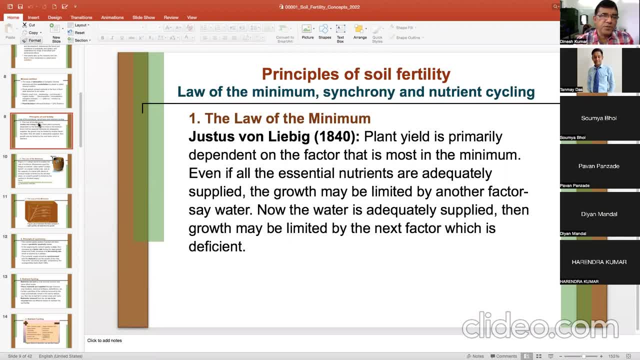 and carbon hydrogen oxygen, you need not to bother. and carbon hydrogen oxygen, you need not to bother. zinc is not there and you have all the zinc is not there and you have all. the zinc is not there and you have all. the other necessary nutrients primary. other necessary nutrients: primary. 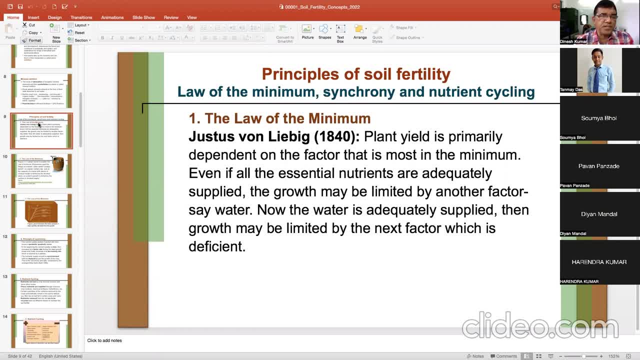 other necessary nutrients: primary nutrients, nutrients, nutrients, secondary nutrients and all other secondary nutrients and all other secondary nutrients and all other micronutrients, micronutrients, micronutrients. so zinc will decide the growth if the so zinc will decide the growth. if the so zinc will decide the growth if the quantity of zinc is below the minimum. 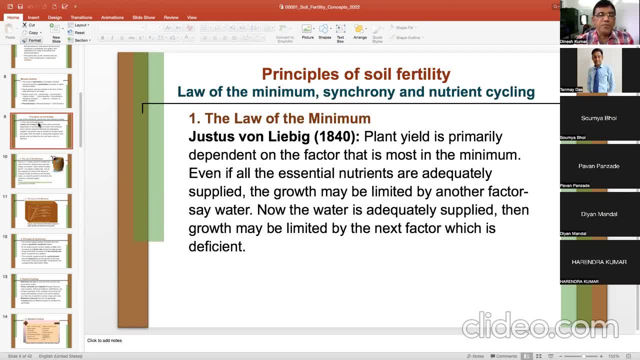 quantity of zinc is below the minimum. quantity of zinc is below the minimum, then plant will not, plants will not. then plant will not, plants will not, then plant will not. plants will not attain good growth. attain good growth. attain good growth if you add the quantity required. quantity: 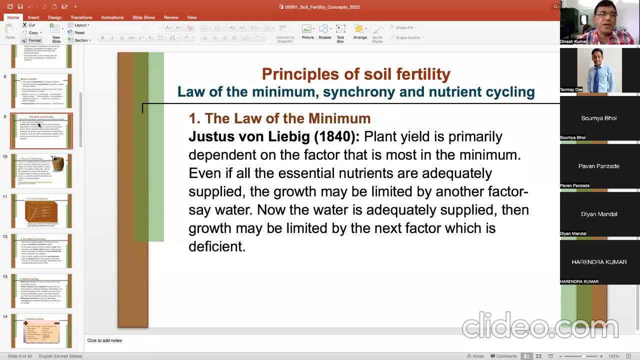 if you add the quantity required quantity, if you add the quantity required quantity of zinc into the soil of zinc, into the soil of zinc, into the soil, then another nutrient can become, then another nutrient can become, then another nutrient can become deficient. then that way you need to. 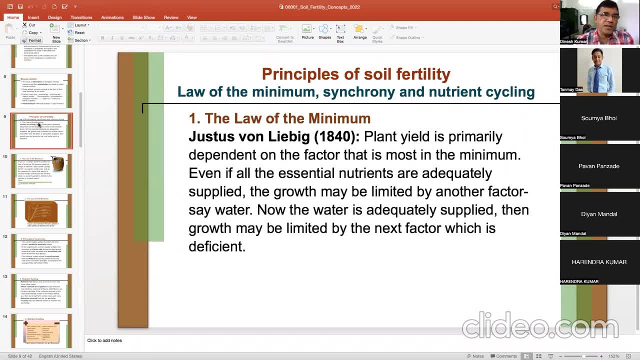 deficient, then that way you need to. deficient, then that way you need to increase the supply of that second. increase the supply of that second, increase the supply of that second. nutrient does, nutrient does. nutrient does. so therefore balance is necessary. one so therefore balance is necessary. one so therefore balance is necessary. one should not be in two axis and one should. 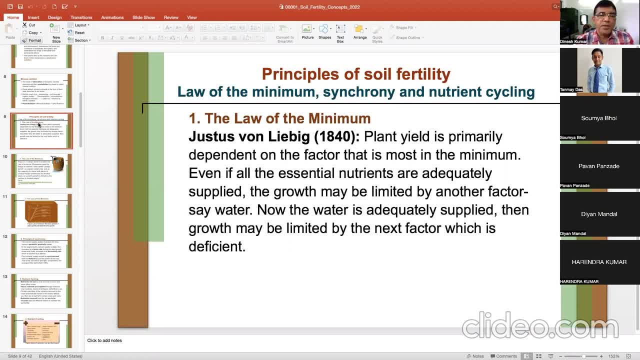 should not be in two axis, and one should should not be in two axis, and one should not be too low, not be too low, not be too low. so that is the law of minimum. if you want, so that is the law of minimum. if you want, so that is the law of minimum. if you want the best result. 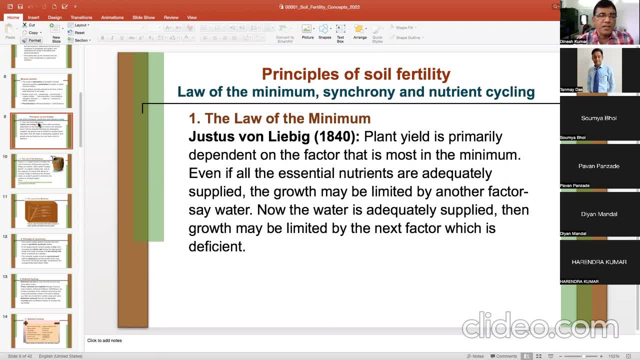 the best result. the best result, every nutrient, every nutrient should be every nutrient, every nutrient should be every nutrient, every nutrient should be present at least minimum quantities present, at least minimum quantities present, at least minimum quantities required for the growth, required for the growth, required for the growth. and this can be defined by, understood by: 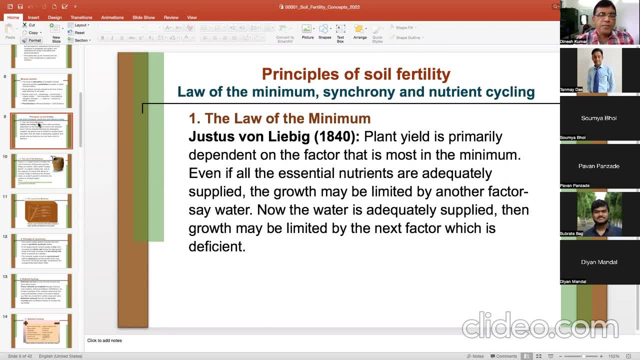 and this can be defined by understood by, and this can be defined by understood by many ways, many ways, many ways. suppose you have food, suppose you have food. suppose you have food before you. you have rice, you have before you, you have rice, you have before you. you have rice. you have chapati dal, everything is there. 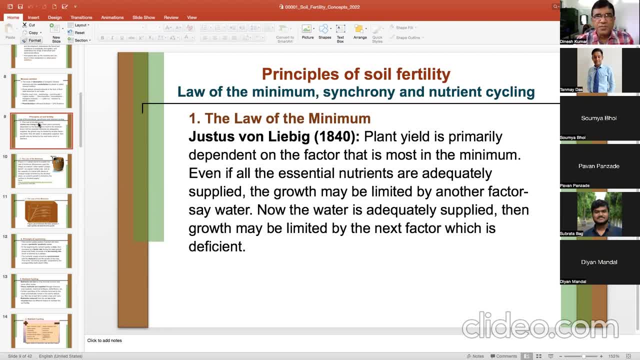 chapati dal: everything is there. chapati dal- everything is there, but you forgot to add the salt. but you forgot to add the salt. but you forgot to add the salt. will you add this food? eat this food. will you add this food? eat this food. will you add this food? eat this food. you will not like to eat this food. you. 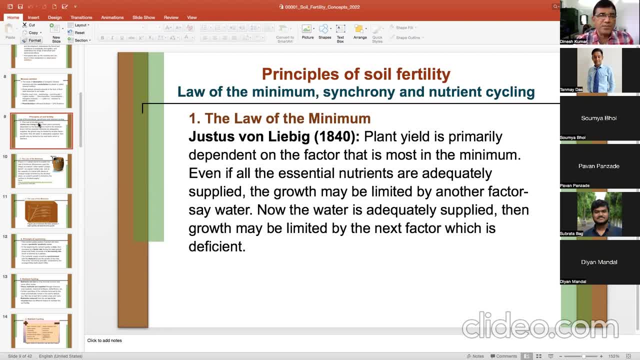 you will not like to eat this food. you, you will not like to eat this food. you will take one or two pieces, and then you will take one or two pieces, and then you will take one or two pieces, and then you will never eat this food without salt. 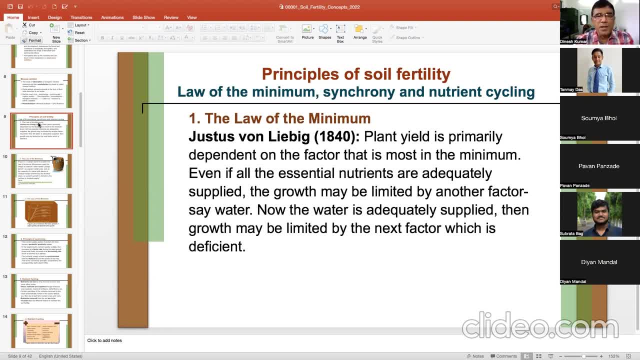 will never eat this food without salt, will never eat this food without salt. so if you add the salt, you will, you will. so if you add the salt, you will, you will. so if you add the salt, you will, you will eat the food. similarly, if you add the, 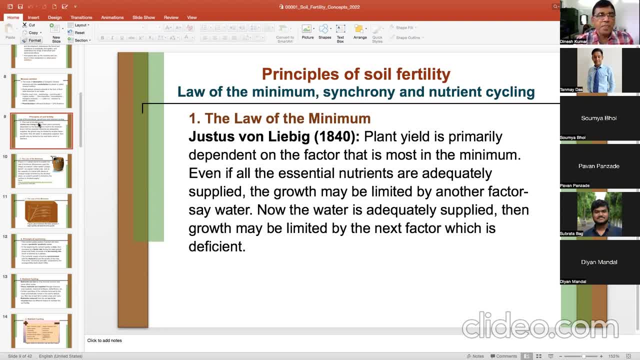 eat the food. similarly. if you add the, eat the food similarly. if you add the micronutrients, or micronutrients, or micronutrients, or any nutrient which is deficient, then any nutrient which is deficient, then any nutrient which is deficient, then then you can achieve better product. 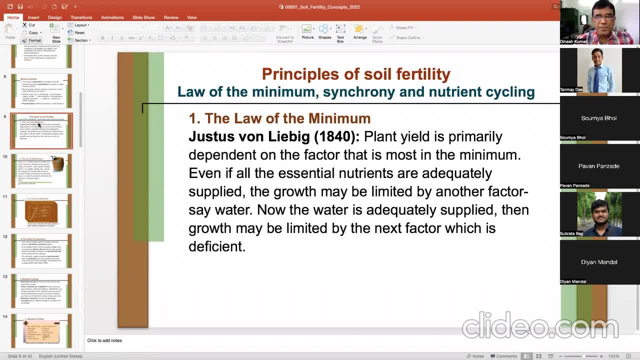 then you can achieve better product. then you can achieve better product. and it is also said that the strength of, and it is also said that the strength of, and it is also said that the strength of a chain, a chain, a chain, the strength of a chain, will be decided. 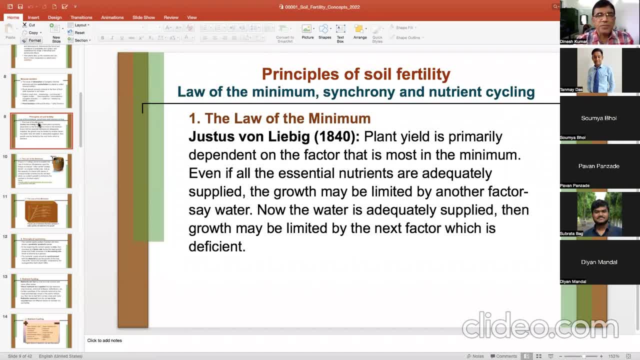 the strength of a chain will be decided. the strength of a chain will be decided by the link which is the weakest, by the link which is the weakest, by the link which is the weakest, so weakest link will decide the strength, so weakest link will decide the strength. 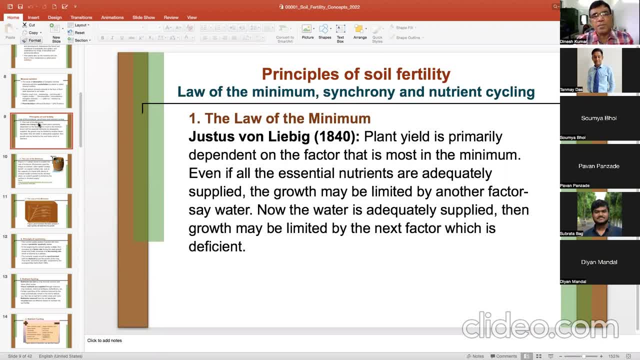 so weakest link will decide the strength of the chain, of the chain of the chain. similarly, if you are running on the, similarly, if you are running on the similarly, if you are running on the road, you are in delhi road, you are in delhi road, you are in delhi and having your vehicle. 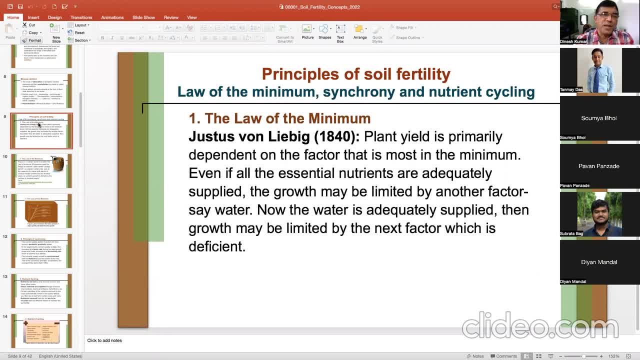 and having your vehicle, and having your vehicle, and, and there is no space to overtake and, and there is no space to overtake, and, and there is no space to overtake, so the vehicle which is running the, so the vehicle which is running the, so the vehicle which is running the slowest. 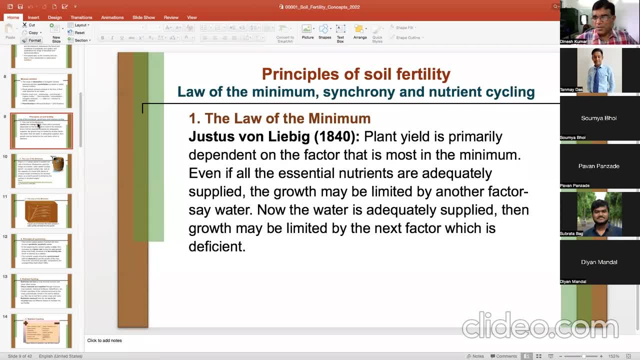 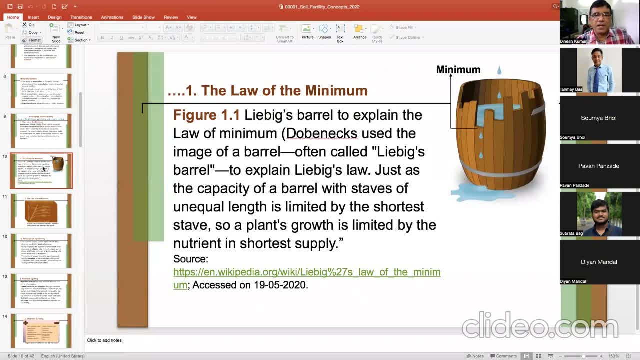 slowest. slowest will decide the speed of others who are, will decide the speed of others who are, will decide the speed of others who are following, following, following, so so. so, this is how you can define it. this is how you can define it. this is how you can define it. libix barrel to explain the law minimum. 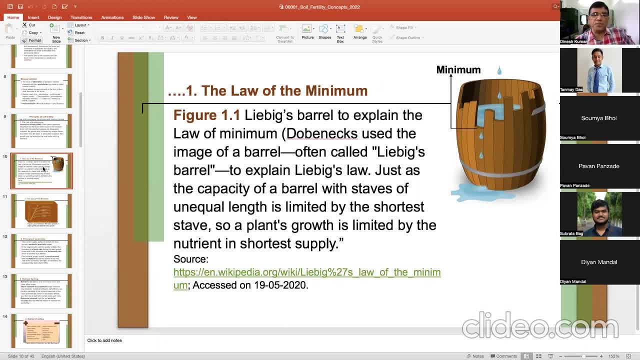 libix barrel to explain the law minimum. libix barrel to explain the law minimum and it was used by toban x. toban x used and it was used by toban x. toban x used and it was used by toban x. toban x used the image of barrel. 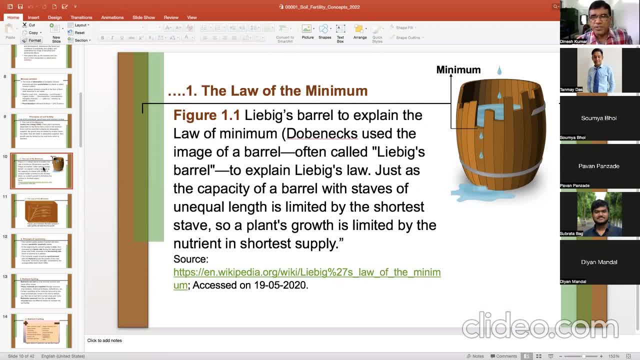 the image of barrel, the image of barrel, often called as libix barrel to explain, often called as libix barrel to explain, often called as libix barrel to explain the libix law, the libix law, the libix law, just as the capacity of a barrel with 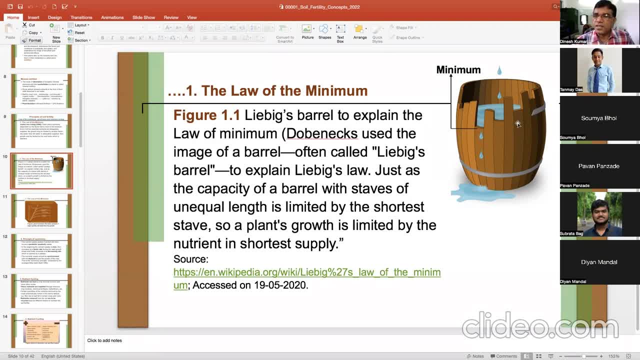 just as the capacity of a barrel with, just as the capacity of a barrel with the states, these structures wooden the states. these structures wooden the states. these structures wooden structures are states, structures are states, structures are states. the states of unequal length, they are of the states of unequal length, they are of. 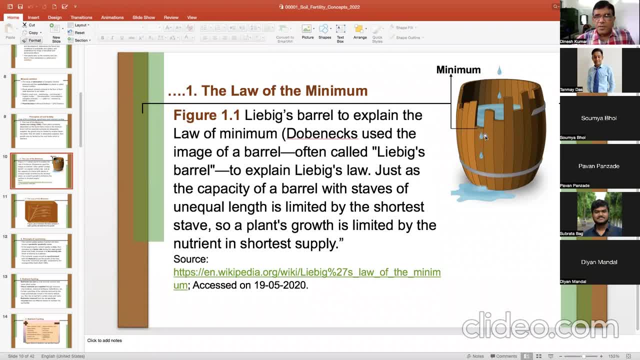 the states of unequal length. they are of unequal length, unequal length, unequal length. uh is limited by the shortest state, so uh is limited by the shortest state, so uh is limited by the shortest state. so total quantity of water that can be. total quantity of water that can be. 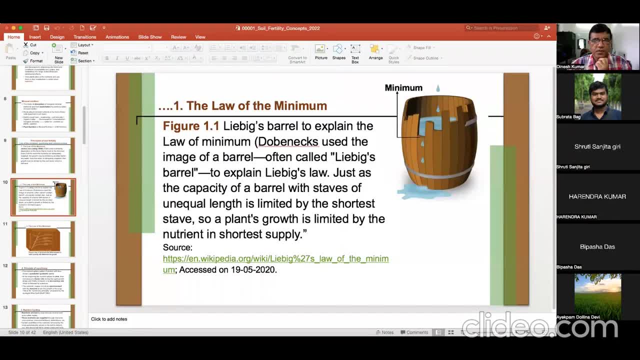 total quantity of water that can be retained. it can be treated as growth of retained. it can be treated as growth of retained. it can be treated as growth of the part, the part, the part. so we can see the, the quantity of growth. so we can see the, the quantity of growth. 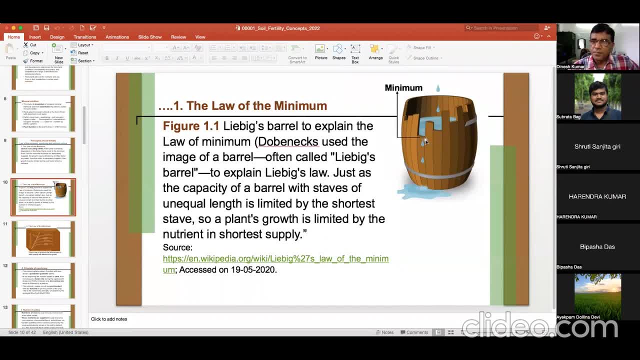 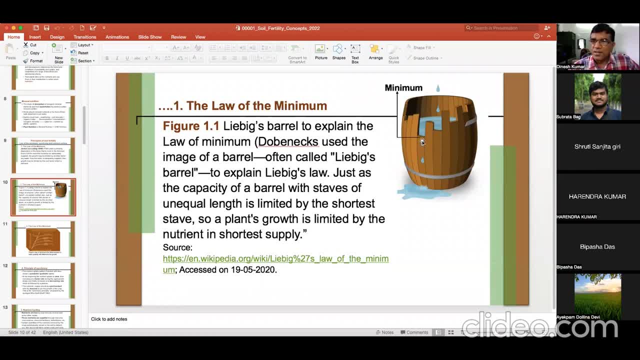 by the state which is at the shortest distance, which is the lowest length distance which is the lowest length distance which is the lowest length, lowest quantity or lowest length, so that lowest quantity or lowest length, so that lowest quantity or lowest length, so that will decide the will decide the. 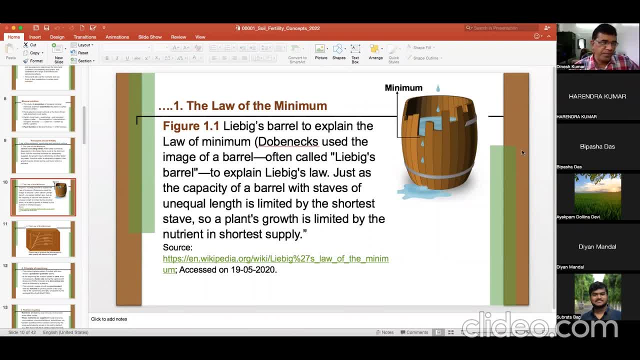 will decide the: the growth of quantity of water in the, the growth of quantity of water in the, the growth of quantity of water in the barrel, barrel, barrel. you'll see another thing here. you'll see another thing here. you'll see another thing here. this is from. 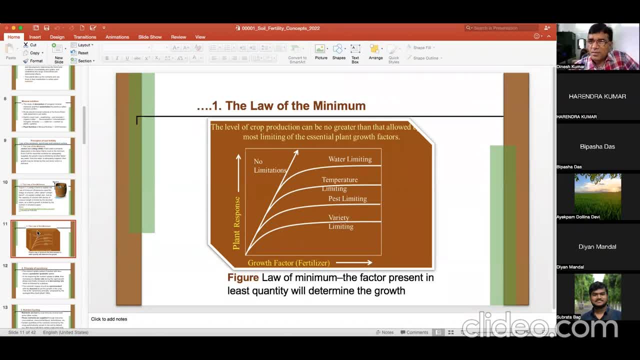 this is from. this is from book of tisdale, book of tisdale, book of tisdale: soil fertility and fertilizers. yeah, diane, do you have that book? yeah, diane, do you have that book? yeah, diane, do you have that book? yes, sir, you have. you have shared during. 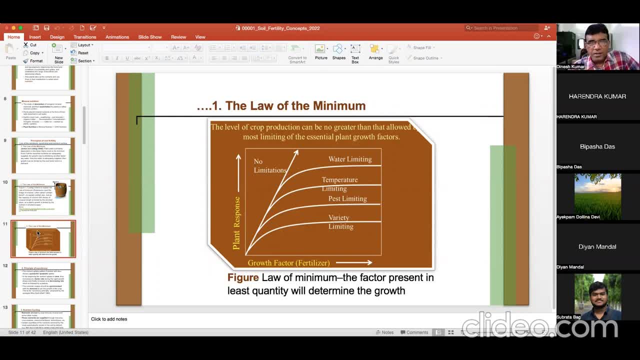 yes, sir, you have you have shared during. yes, sir, you have you have shared during. the first semester. good so the first semester. good so the first semester. good so, uh, you can study uh this, uh, you can study uh this. uh, you can study uh this law of minimum there are in that book. 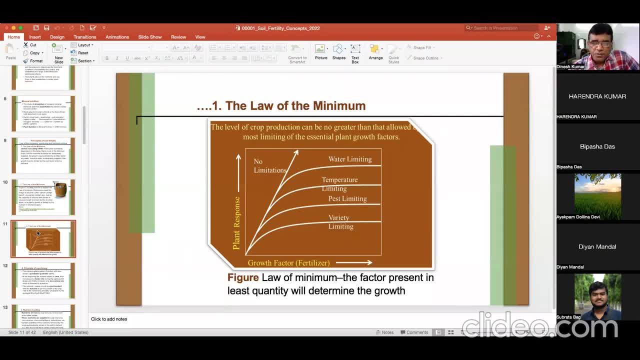 law of minimum. there are in that book, law of minimum. there are in that book some information is given. i just copied. some information is given. i just copied some information is given. i just copied from there, from there, from there, so you can see: law of minimum, the. 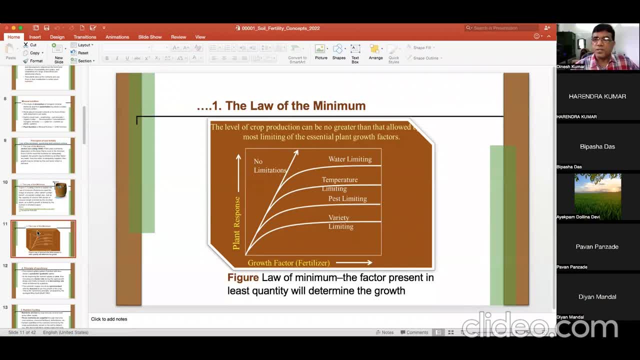 so you can see law of minimum, the. so you can see law of minimum the factor present in least quantity will factor present in least quantity. will factor present in least quantity will determine the growth. so, instead of taking, determine the growth. so, instead of taking, determine the growth. so, instead of taking different nutrients, he has explained it. 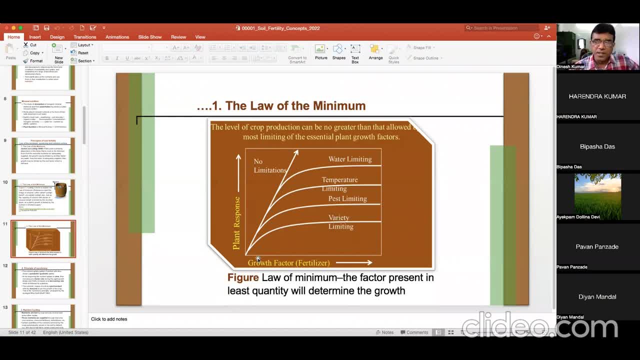 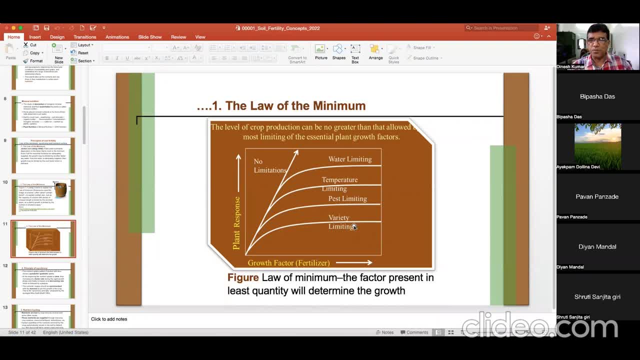 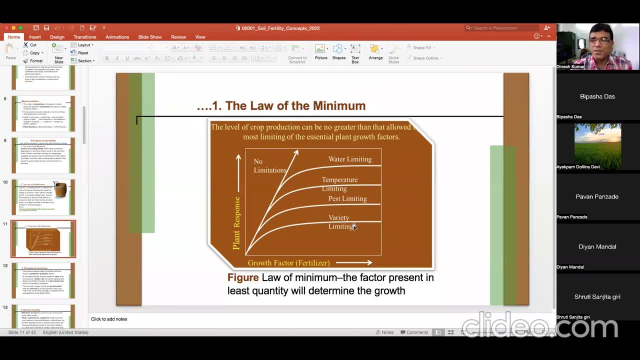 if variety is poor and you, whatever. if variety is poor and you, whatever quantity of water you apply, you give quantity of water, you apply. you give quantity of water you apply. you give ideal temperature, you control the pest. ideal temperature: you control the pest. ideal temperature, you control the pest. you do everything, but still it will not. 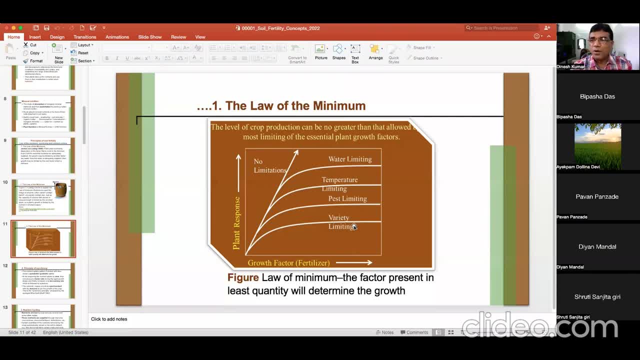 you do everything, but still it will not. you do everything, but still it will not yield good. because variety was a yield good, because variety was a yield good. because variety was a limitation, it was low yielding variety limitation, it was low yielding variety limitation, it was low yielding variety. suppose now you have changed the 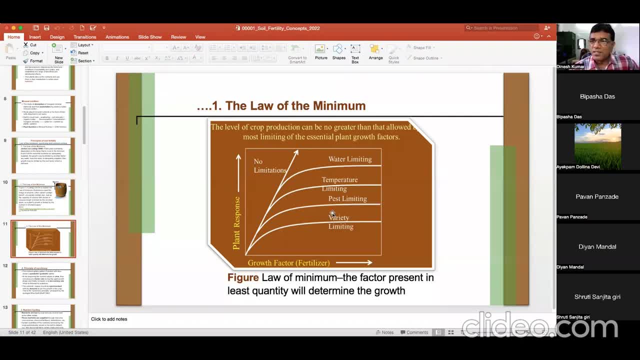 suppose: now you have changed the suppose, now you have changed the, you have changed the variety, you have changed the variety, you have changed the variety. now variety is giving good yield, but now variety is giving good yield. but now variety is giving good yield, but again it is infested by 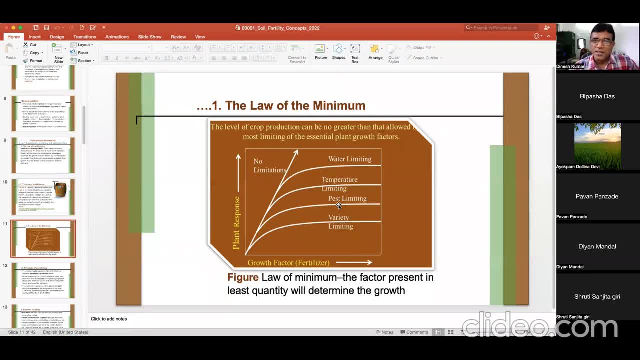 again it is infested by. again it is infested by. so pest can pest can decrease the yield. so pest can pest can decrease the yield. so pest can pest can decrease the yield, decrease the growth, decrease the growth, decrease the growth. and again you have controlled the pest. 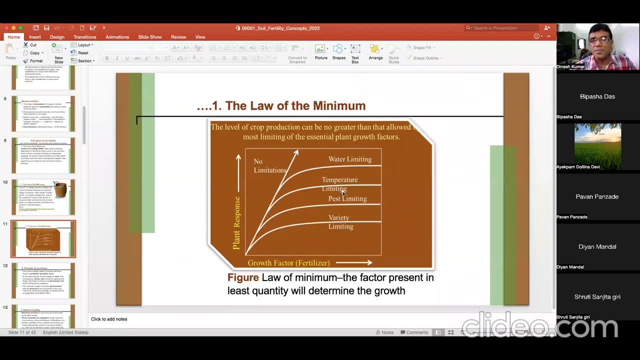 and again you have controlled the pest. and again you have controlled the pest. suppose you have good variety control. suppose you have good variety control, suppose you have good variety, control the pest. then next time temperature, can the pest, then next time temperature: can the pest. then next time temperature can become limited, you can have low. 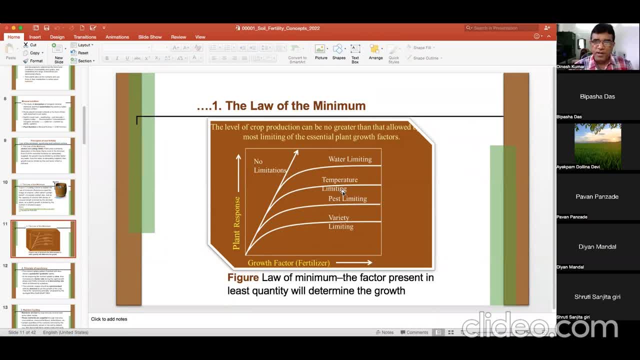 become limited. you can have low, become limited. you can have low temperature or high temperature means temperature, or high temperature means temperature or high temperature means another growth factor. can become another growth factor, can become another growth factor, can become limited, limited, limited. okay, i will overcome this factor also. 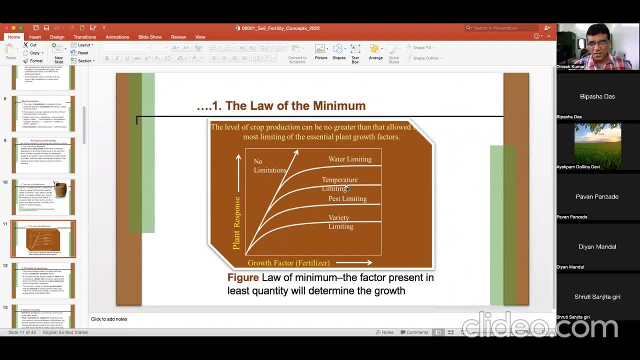 okay, i will overcome this factor also. okay, i will overcome this factor also. then water will become limited. so it is, then water will become limited. so it is like this in nature in, like this in nature in, like this in nature in in agriculture. all the factors are not. 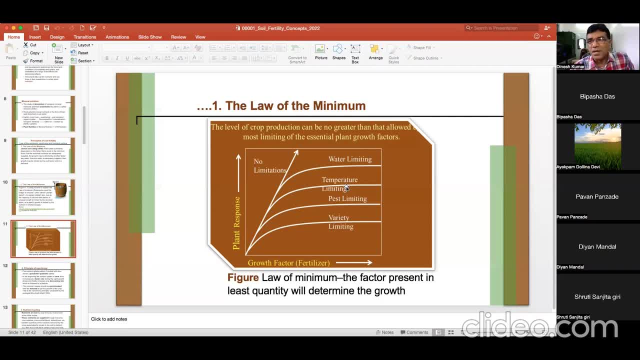 in agriculture, all the factors are not in agriculture, all the factors are not at their best. so sometimes one factor is at their best, so sometimes one factor is at their best. so sometimes one factor is limiting, sometimes other so this one limiting, sometimes other so this one limiting, sometimes other so this one limiting factor. 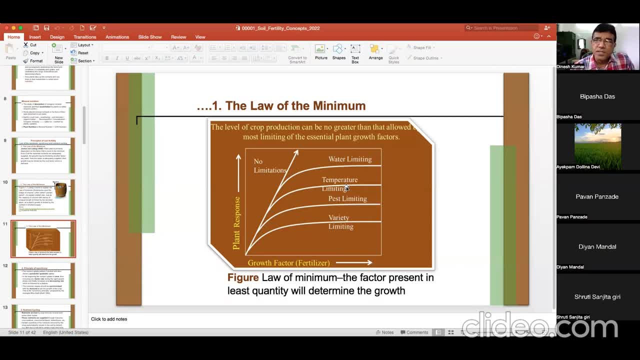 limiting factor. limiting factor will affect the growth. the growth will be will affect the growth. the growth will be will affect the growth. the growth will be affected much by the limiting factor, affected much by the limiting factor, affected much by the limiting factor. similar is the case of your nutrients. 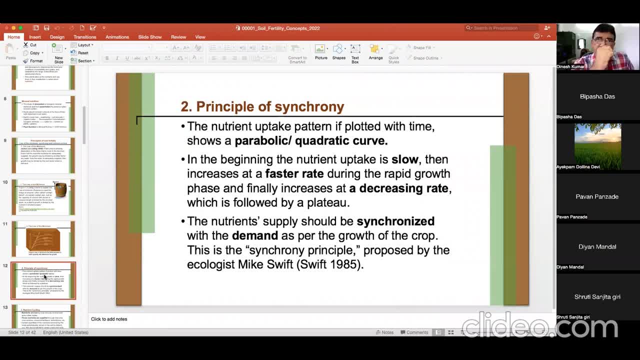 similar is the case of your nutrients. similar is the case of your nutrients. next is principle of synchronic- i already. next is principle of synchronic: i already. next is principle of synchronic. i already told you that you should told you that you should told you that you should um ensure that supply of the nutrient is. 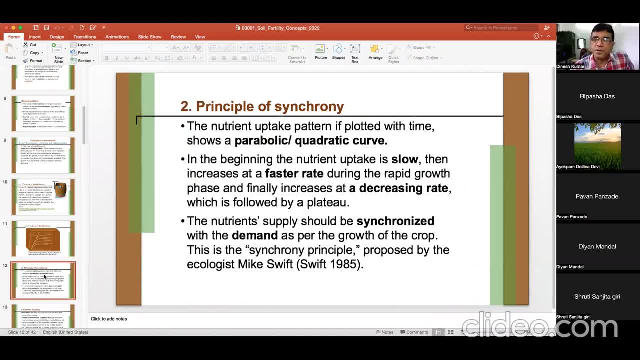 um ensure that supply of the nutrient is. um ensure that supply of the nutrient is according to the need of the plant. so according to the need of the plant, so according to the need of the plant. so this is also principle of, this is also principle of, this is also principle of sulfur. so the nutrient update pattern is: 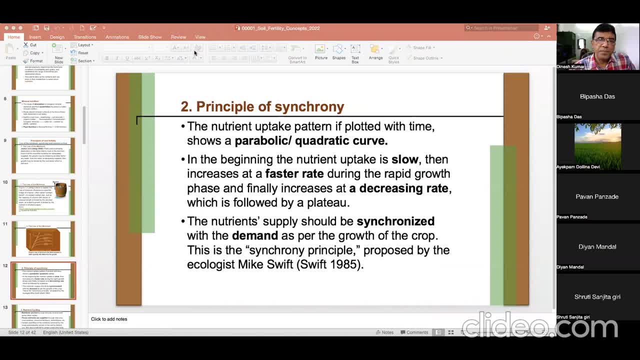 sulfur, so the nutrient update pattern is sulfur, so the nutrient update pattern is plotted with time, plotted with time, plotted with time. it, plotted with time, shows a parabolic quadratic term. parabolic shows a parabolic quadratic term. parabolic shows a parabolic quadratic term. parabolic quadratic companies. initially the 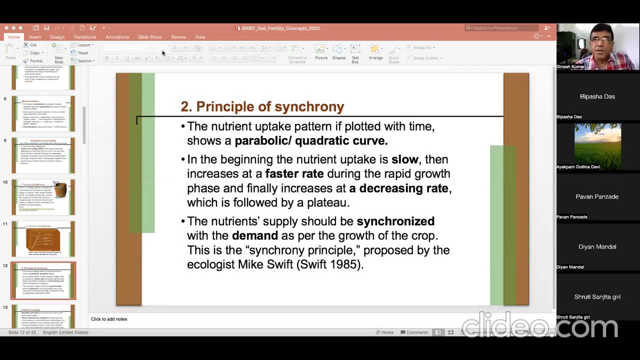 quadratic companies. initially the quadratic companies, initially the growth or requirement is low, and then at growth or requirement is low, and then at growth or requirement is low, and then at the rapid growth stage, the requirement, the rapid growth stage, the requirement, the rapid growth stage, the requirement is higher and in the end, the requirement. 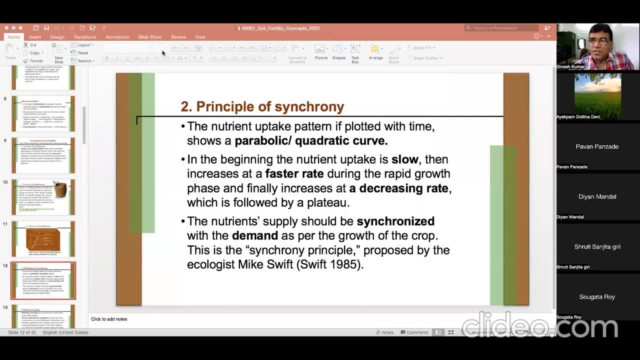 is higher and in the end, the requirement is higher and in the end, the requirement is low. i think you, if you remember, i is low. i think you, if you remember, i is low. i think you, if you remember, i discussed the parabolic relationship in, discussed the parabolic relationship in. 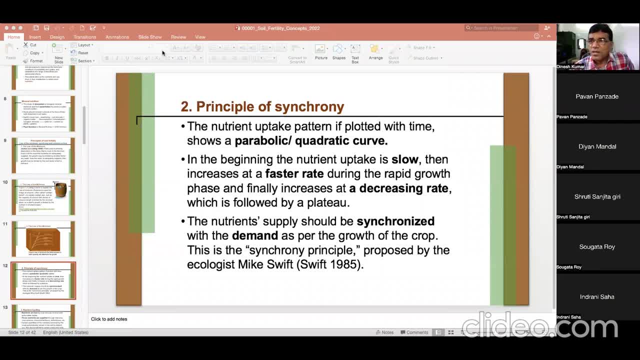 discussed the parabolic relationship in principles of pro production, at great principles of pro production, at great principles of pro production, at great length, quadratic curve at death. greatly length, quadratic curve at death. greatly length, quadratic curve at death, greatly so. it follows quadratic response, kind of. so it follows quadratic response, kind of. 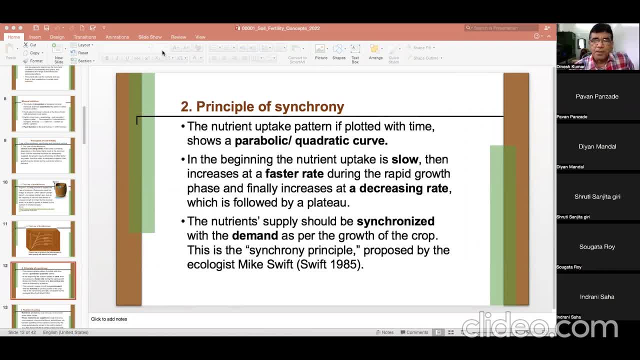 so it follows quadratic response. kind of thing means uptake of nutrient is thing means uptake of nutrient is thing means uptake of nutrient is related to, related to, related to the kind of growth plants, the kind of growth plants, the kind of growth plants during the rapid growth phase. and 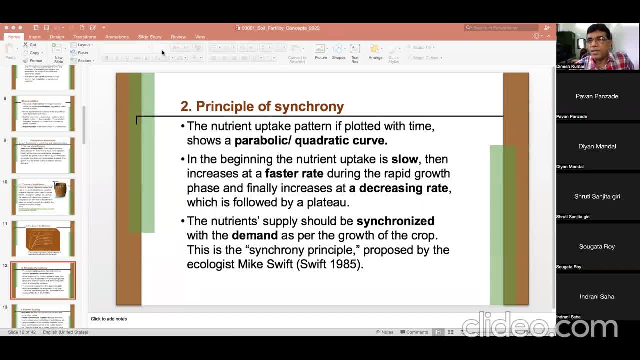 during the rapid growth phase and during the rapid growth phase. and finally, increases at a decreasing rate, finally increases at a decreasing rate, finally increases at a decreasing rate, which is followed by a plateau, which is followed by a plateau, which is followed by a plateau. the nutrient supply should be synchronized. 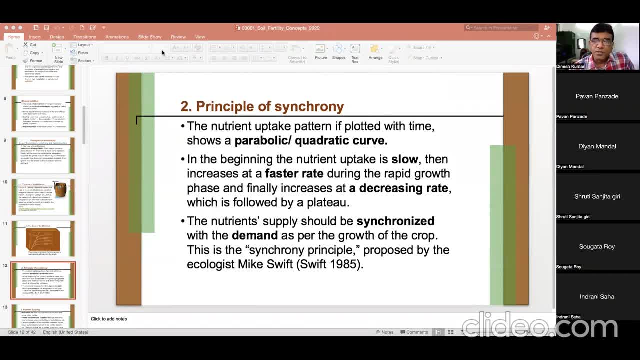 the nutrient supply should be synchronized. the nutrient supply should be synchronized with the demand as per growth of the, with the demand as per growth of the, with the demand as per growth of the crop. this is the synchronic principle crop. this is the synchronic principle crop. this is the synchronic principle proposed by the ecologist mike. 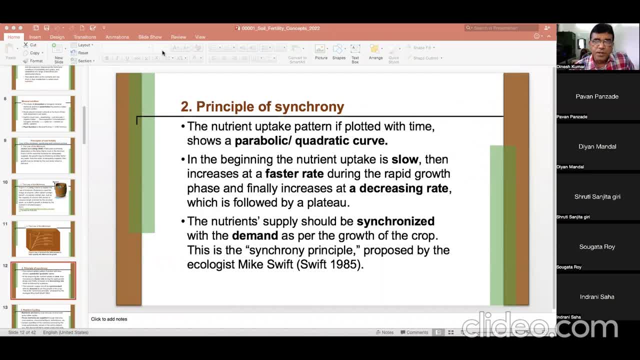 proposed by the ecologist mike. proposed by the ecologist mike mike. swift is the example. who proposed a mike? swift is the example. who proposed a mike swift is the example who proposed a principle of synchrony, principle of synchrony, principle of synchrony. and you can remember this name: swift. 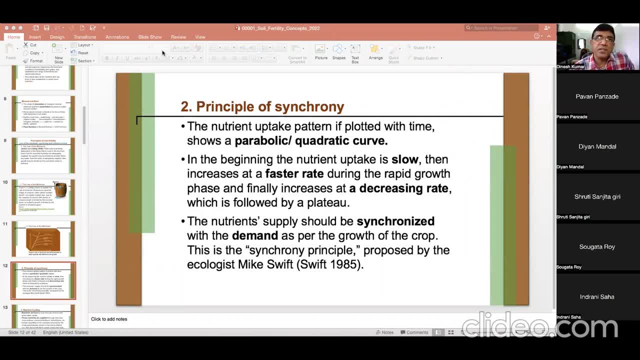 and you can remember this name: swift. and you can remember this name: swift 1985. 1985. 1985.. this question may come in some of the. this question may come in some of the. this question may come in some of the quizzes. 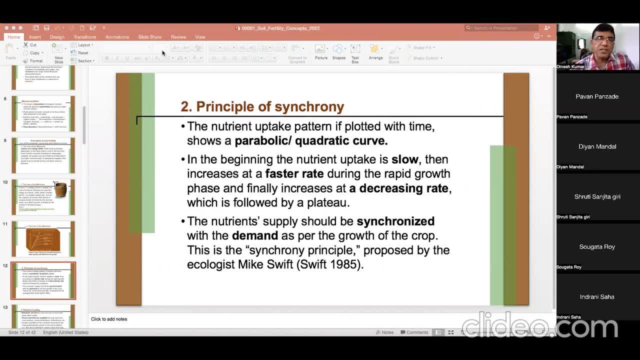 quizzes, quizzes: swift 1985.. swift 1985.. swift 1985.. so here you can see, i give you one. so here you can see, i give you one. so here you can see, i give you one example, example, example. example of rice. example of rice. 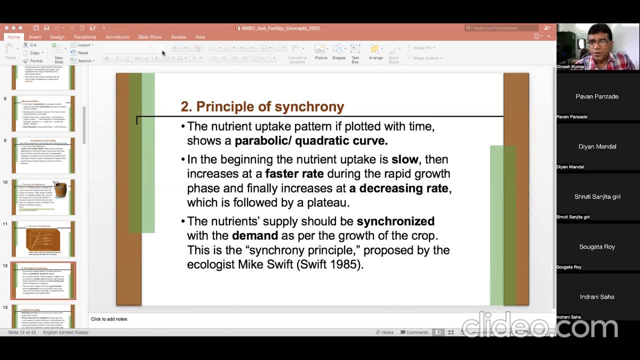 example of rice in rice nutrient management, in rice nutrient management, in rice nutrient management or any other growth or any other growth or any other growth. phosphorus and potashic fertilizer. phosphorus and potashic fertilizer. phosphorus and potashic fertilizer. zinc fertilizer. they are generally. 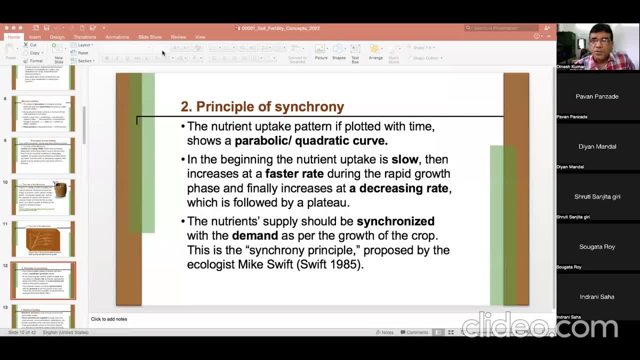 zinc fertilizer. they are generally zinc fertilizer. they are generally recommended at the time of recommended at the time of recommended at the time of sowing. sowing sowing part of nitrogenous fertilizer in rice, part of nitrogenous fertilizer in rice. part of nitrogenous fertilizer in rice is also recommended at transplanting of. 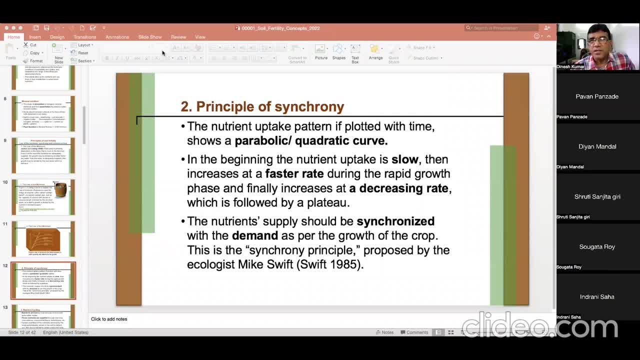 is also recommended at transplanting of. is also recommended at transplanting of soil, soil, soil. the recommendation of accurate is that. the recommendation of accurate is that. the recommendation of accurate is that you should apply half nut. you should apply half nut. you should apply half nut is half nitrogen at the time of planting. 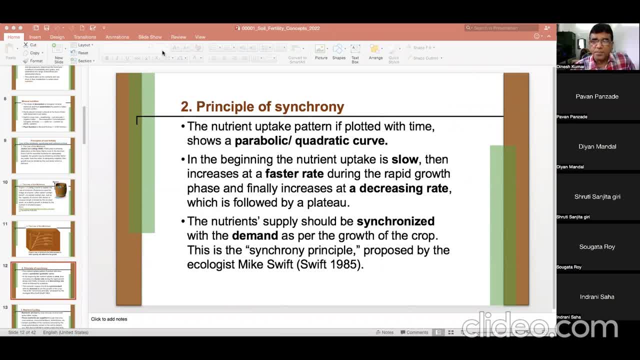 is half nitrogen at the time of planting, is half nitrogen at the time of planting and remaining half should be split into and remaining half should be split into and remaining half should be split into two parts. two parts, two parts. but if you see recommendation from ira, 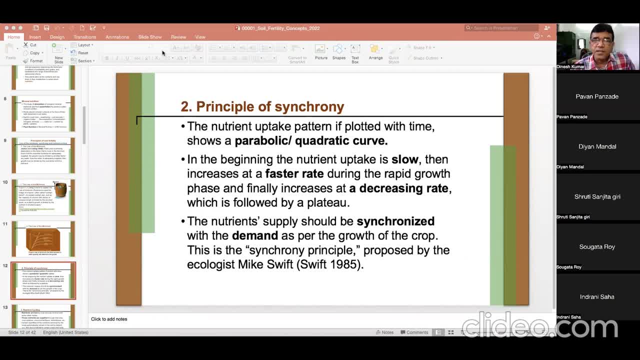 but if you see recommendation from ira, but if you see recommendation from ira, ira never recommended nitrogen application at the time of nitrogen application at the time of nitrogen application at the time of transplant, transplant, transplant. it recommends only three splits of. it recommends only three splits of. 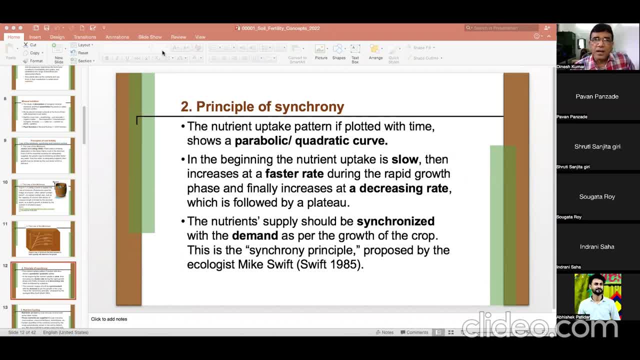 it recommends only three splits of running running running: one at 10 days after transplanting. one at 10 days after transplanting. one at 10 days after transplanting. another at 25 to 30 days after planting. another at 25 to 30 days after planting. another at 25 to 30 days after planting, and third one is at 55 to 60 days after, and third one is at 55 to 60 days after, and third one is at 55 to 60 days after transplanting. so these are the. 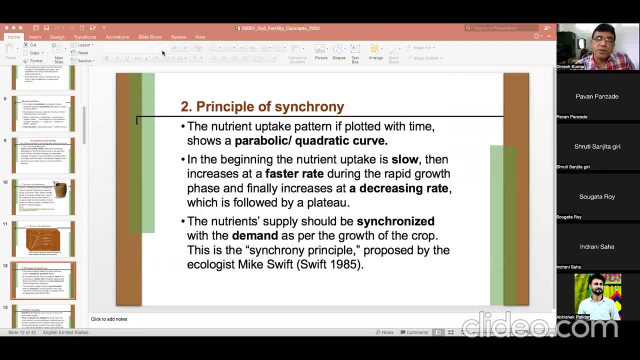 transplanting. so these are the transplanting, so these are the recommendation, why ira gave this recommendation, why ira gave this recommendation, why ira gave this recommendation, recommendation, recommendation of three splits. because in the building of three splits, because in the building of three splits, because in the building your seedlings are quite new, their your seedlings are quite new. their your seedlings are quite new. their requirement for nutrient is not that high. requirement for nutrient is not that high. requirement for nutrient is not that high. so so so whatever is required is already there. whatever is required is already there. whatever is required is already there. that much minimum. 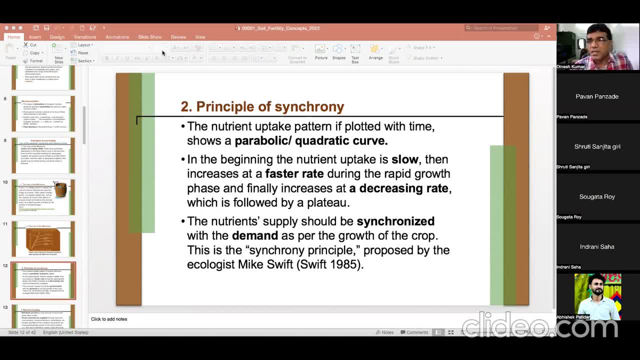 that much minimum. that much minimum. nitrogen is there in the soil, so nitrogen is there in the soil, so nitrogen is there in the soil. so, therefore, why to apply basal application? therefore, why to apply basal application? therefore, why to apply basal application in rice, in rice, in rice? why? why? because plant will not use much. 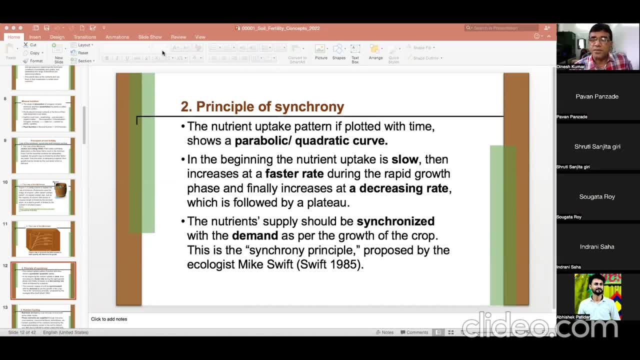 why? why? because plant will not use much. why why? because plant will not use much of the applied nitrogen for next 15 days of the applied nitrogen for next 15 days, of the applied nitrogen for next 15 days at least, at least, at least, so that nitrogen will be liable to be. 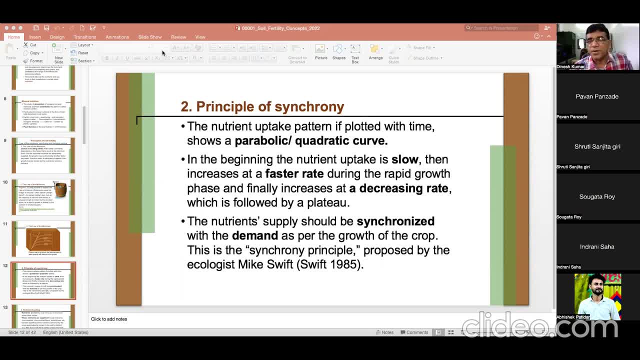 so that nitrogen will be liable to be, so that nitrogen will be liable to be lost. so unnecessarily we are recommending lost. so unnecessarily we are recommending lost. so unnecessarily we are recommending nitrogen in rice for nitrogen in rice for nitrogen in rice for at the time of transplanting, called this. 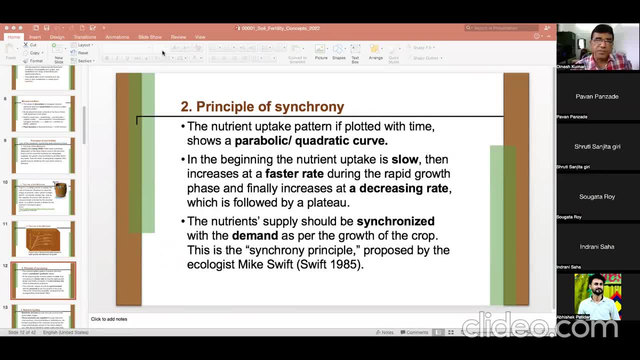 at the time of transplanting, called this, at the time of transplanting, called this. so that is just to meet the. so that is just to meet the. so that is just to meet the requirement of the chrome split requirement of the chrome split requirement of the chrome split application. 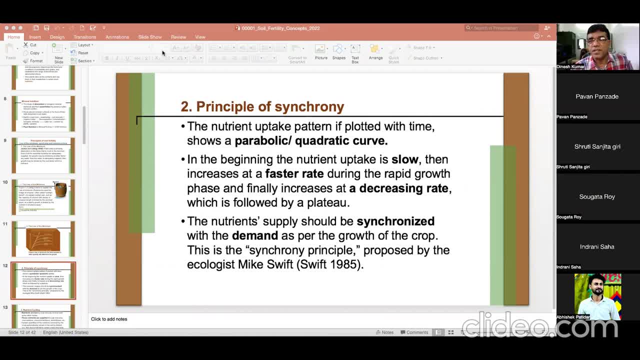 application, application, and then again after 55 or 60 days of, and then again after 55 or 60 days of, and then again after 55 or 60 days of transplanting, transplanting, transplanting. that time you will apply third dose and that time you will apply third dose. and. 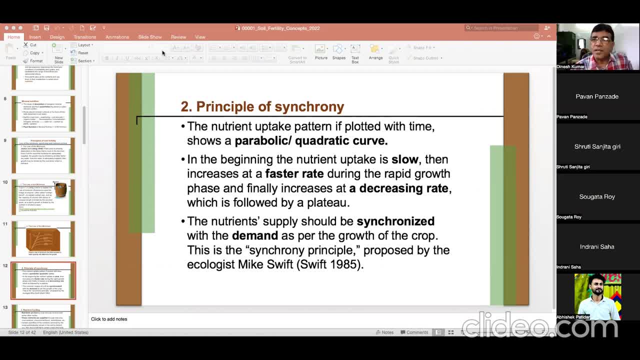 that time you will apply third dose, and after that you don't apply. because after that you don't apply, because after that you don't apply because the the, then the requirement will fall, the the, then the requirement will fall, the the, then the requirement will fall. requirement for nitrogen. 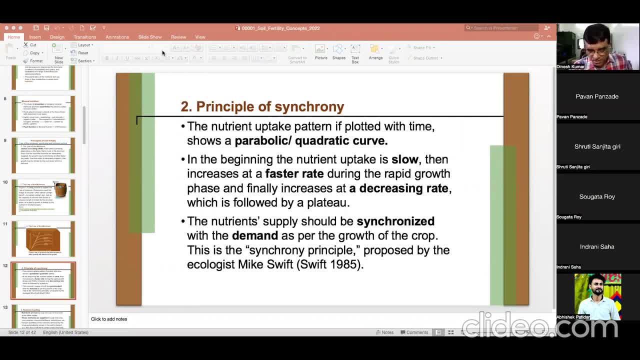 requirement for nitrogen. requirement for nitrogen will fall. so therefore, you are just will fall. so therefore, you are just will fall. so therefore, you are just matching the matching, the matching the supply and requirement, supply and requirement, supply and requirement. so this is your principle of simple. so, this is your principle of simple. 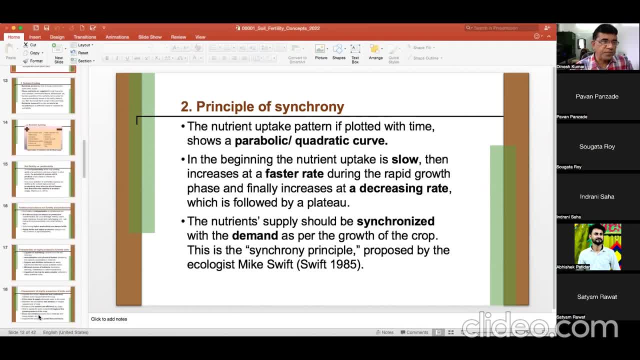 so this is your principle of simple, then third one is, then third one is, then third one is uh principle of cycling, uh principle of cycling, uh principle of cycling nutrients update pattern: if plotted nutrients update pattern. if plotted nutrients update pattern. if plotted with time. with time, with time shows it, this is over. so 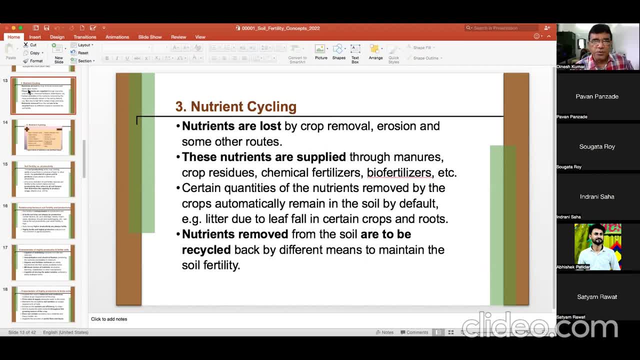 nutrient cycling. nutrient cycling, nutrient cycling. nutrients are lost by crop removal. nutrients are lost by crop removal. nutrients are lost by crop removal, erosion and some other roots, erosion and some other roots, erosion and some other roots. so you know that nutrients are removed, so you know that nutrients are removed. 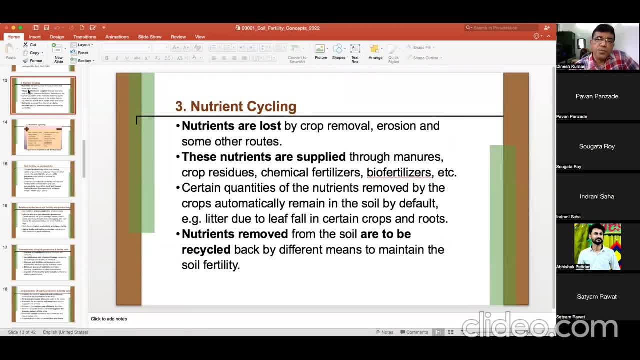 so you know that nutrients are removed from the soil. there is. there are input from the soil. there is. there are input from the soil. there is. there are input and out and out and out. so output are mainly crop removal erosion. so output are mainly crop removal erosion. 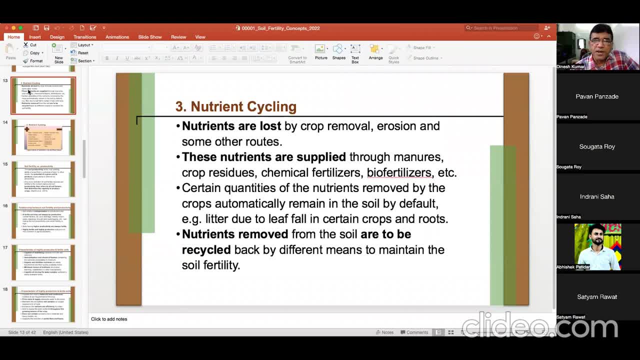 so output are mainly crop removal, erosion and some other roots like your and some other roots like your and some other roots like your: volatilization of nitrogen, volatilization of nitrogen, volatilization of nitrogen, leaching of sulfate, etc. leaching of sulfate, etc. 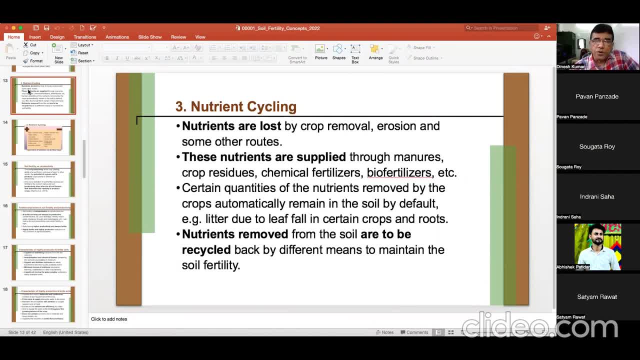 leaching of sulfate, etc. these nutrients are supplied through. these nutrients are supplied through. these nutrients are supplied through manuals, manuals, manuals, crop residues, chemical fertilizers and crop residues, chemical fertilizers and crop residues. chemical fertilizers and biofertilizer, biofertilizer, biofertilizer- so number of sources are used to supply. 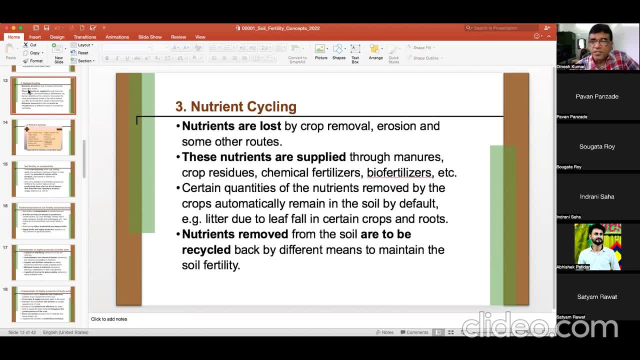 so number of sources are used to supply, so number of sources are used to supply these nutrients, certain quantities of these nutrients, certain quantities of these nutrients, certain quantities of these nutrients removed by the crops, these nutrients removed by the crops, these nutrients removed by the crops, automatically remain in the soil by 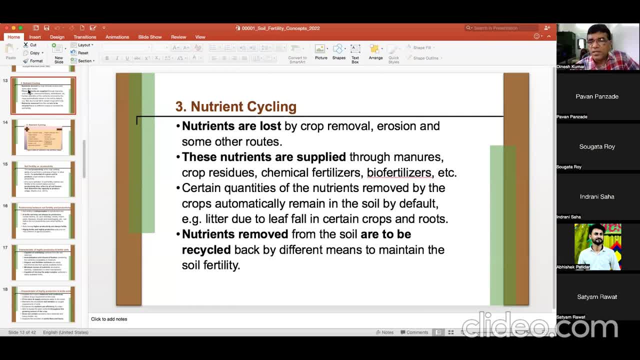 automatically remain in the soil. by automatically remain in the soil by default, for example, liter, due to default, for example, liter. due to default, for example, liter. due to default in certain groups and groups. so default in certain groups and groups. so default in certain groups and groups. so, whatever nutrients you apply, 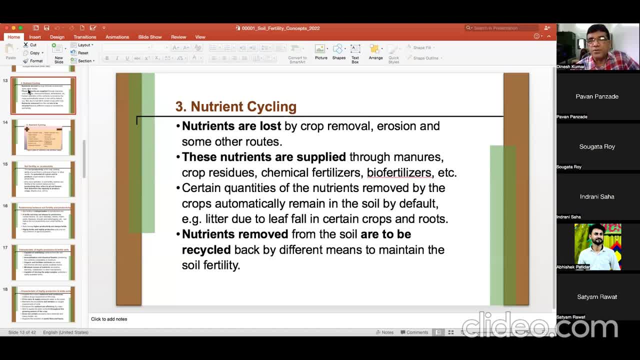 whatever nutrients you apply, whatever nutrients you apply, and whatever are there the total nutrient and whatever are there the total nutrient and whatever are there the total nutrient out of total nutrients available in out of total nutrients available in out of total nutrients available in the soil, the soil. 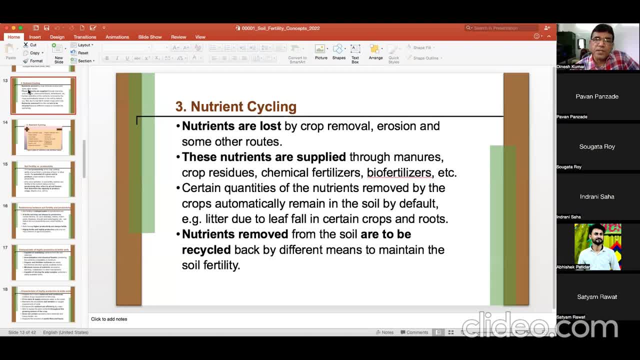 the soil. some will be lost by erosion or leaching. some will be lost by erosion or leaching. some will be lost by erosion or leaching or other other means, and some will be or other other means, and some will be or other other means and some will be removed by the 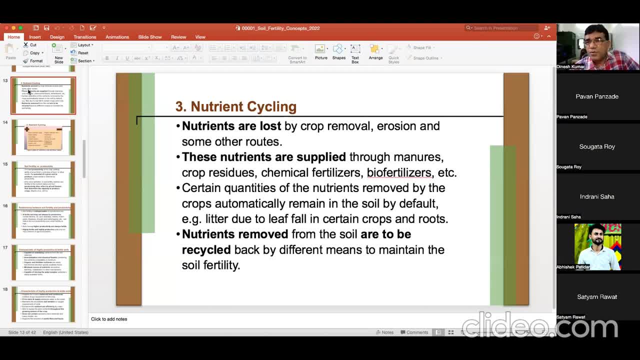 removed by the removed by the crop, but some or some of the nutrients crop, but some or some of the nutrients crop, but some or some of the nutrients which are removed by the crop, which are removed by the crop, which are removed by the crop, they will still remain in the soil in. 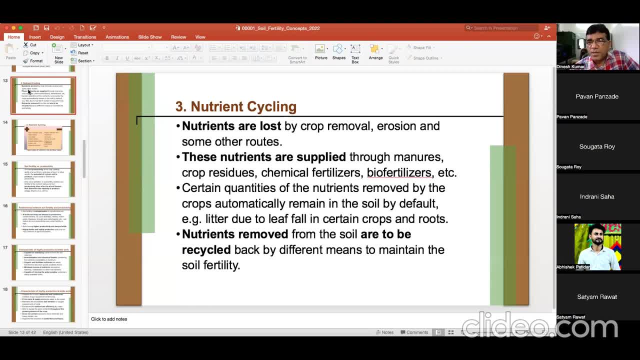 they will still remain in the soil in. they will still remain in the soil in the form of root, or in the form of the form of root, or in the form of the form of root, or in the form of anchored stubbles or maybe fallen leaves. anchored stubbles or maybe fallen leaves. 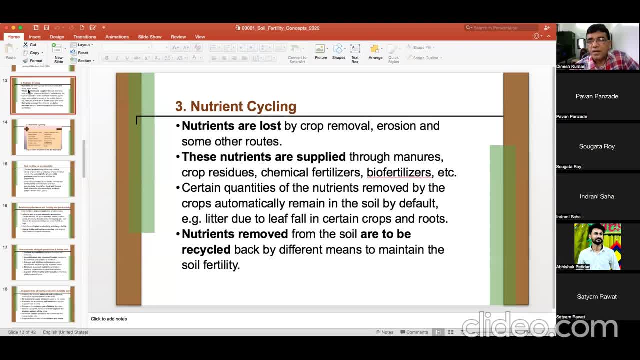 anchored stubbles or maybe fallen leaves, so they, they will be recycled naturally. so they. they will be recycled naturally. so they. they will be recycled naturally. they will be recycled automatically. they will be recycled automatically. they will be recycled automatically. but the nutrients which are removed in, but the nutrients which are removed in. 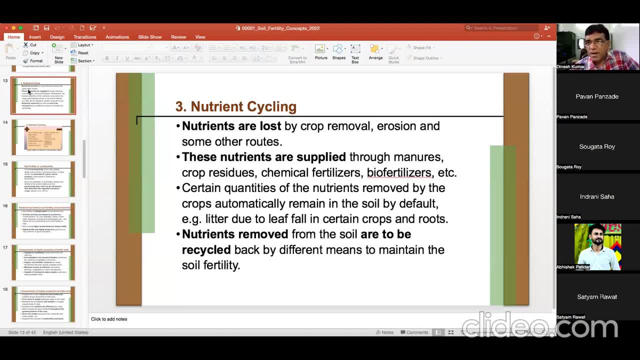 but the nutrients which are removed in the harvest, the harvest, the harvest. we should try to bring them back as much. we should try to bring them back as much. we should try to bring them back as much as possible, as possible, as possible. so nutrient cycling should be practice. 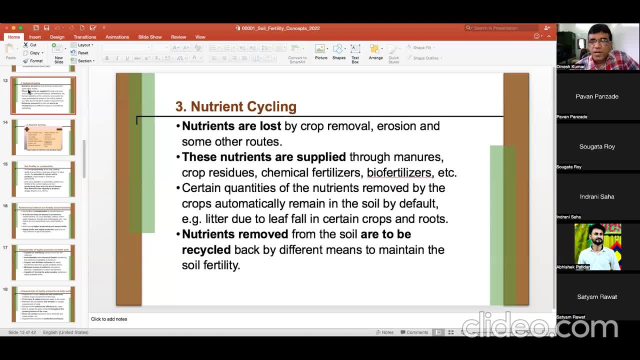 so nutrient cycling should be practice, so nutrient cycling should be practice. nutrients removed from the soil are to. nutrients removed from the soil are to. nutrients removed from the soil are to be recycled back, be recycled back, be recycled back by different means to maintain the soil, by different means to maintain the soil. 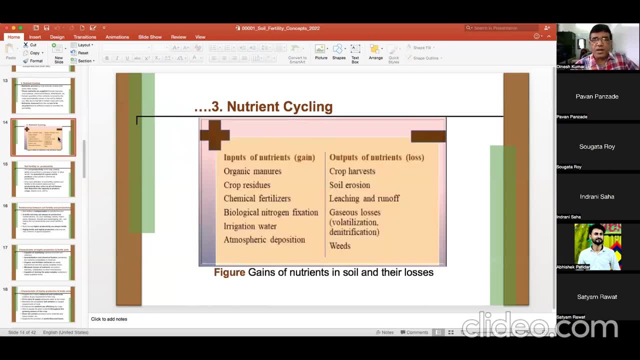 by different means to maintain the soil: fertility, fertility, fertility. so you can see the input and output of. so you can see the input and output of. so you can see the input and output of nutrients. inputs are your nutrients? inputs are your nutrients. inputs are your organic manuals supply nutrient? 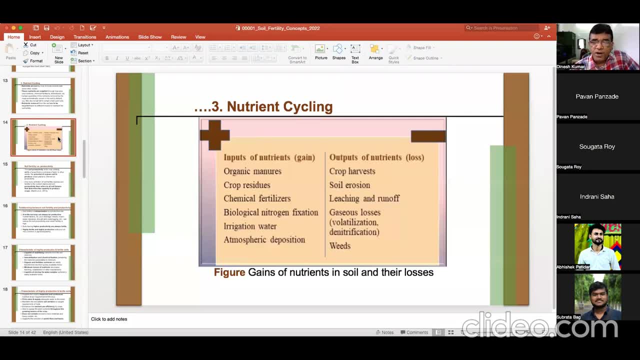 organic manuals: supply nutrient: organic manuals- supply nutrient: crop residues, fertilizers bnf. crop residues, fertilizers bnf. crop residues, fertilizers bnf. irrigation water also supplies some irrigation water also supplies some irrigation water also supplies some nutrients: atmospheric deposition nutrients- atmospheric deposition nutrients, atmospheric deposition. outputs may be grow. harvest erosion. 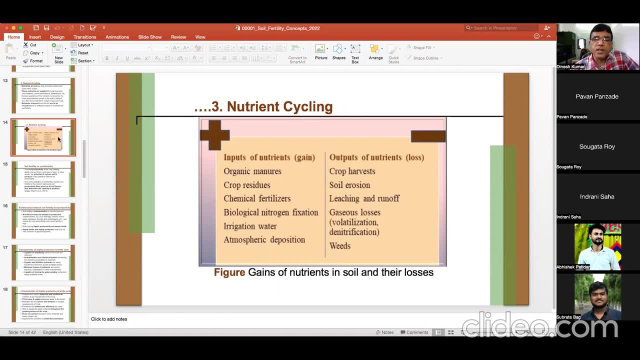 outputs may be grow. harvest erosion. outputs may be grow. harvest erosion. leaching runoff gaseous losses and leaching runoff gaseous losses and leaching runoff gaseous losses and fields. these are the inputs and outputs fields. these are the inputs and outputs fields. these are the inputs and outputs. we need to at least balance them. 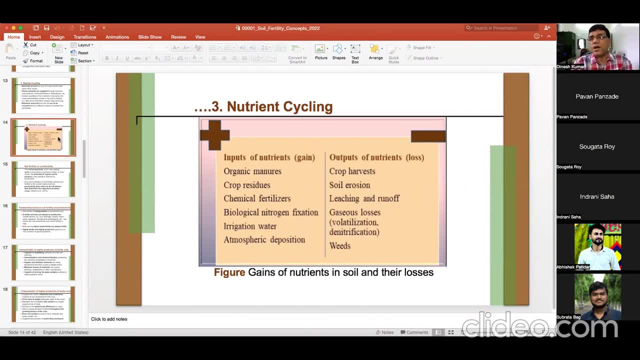 we need to at least balance them. we need to at least balance them. we need to balance them. if you have less, we need to balance them. if you have less, we need to balance them. if you have less input and more output, someday your input and more output someday your. 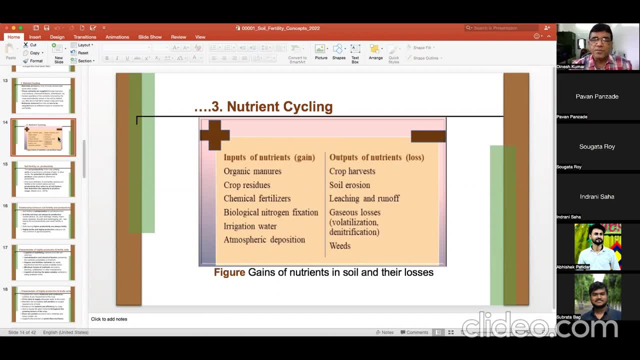 input and more output, someday, your fertility will become very, very poor and fertility will become very, very poor and fertility will become very, very poor and then it will not be able to sustain the, then it will not be able to sustain the, then it will not be able to sustain the productivity. so, therefore, at least a 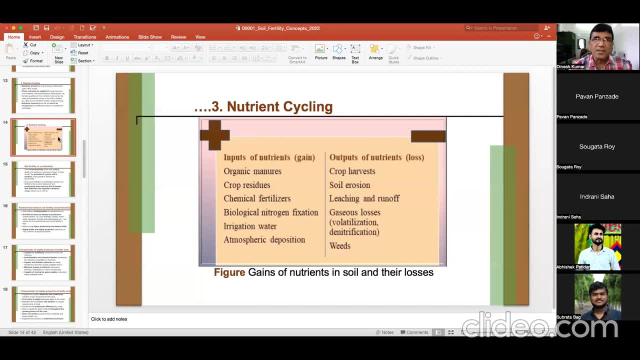 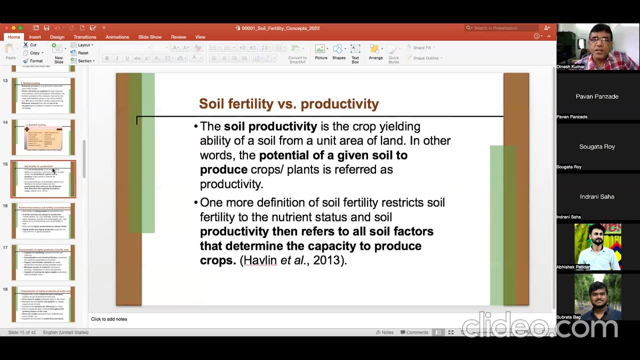 productivity. so therefore at least a productivity. so therefore at least a balance should be removed. whatever you balance should be removed, whatever you balance should be removed, whatever you take out, you must add it. add it into it then then then differences in fertility and productivity. differences in fertility and productivity. 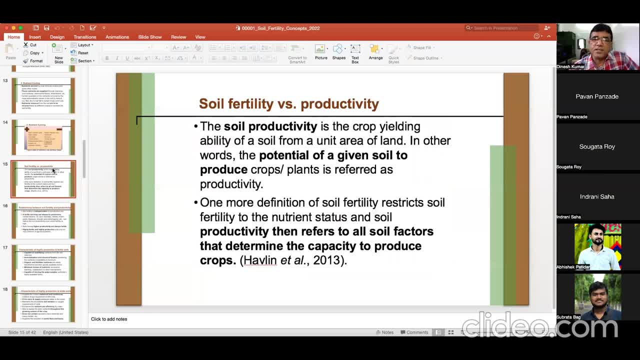 differences in fertility and productivity. so productivity is the crop yielding, so productivity is the crop yielding. so productivity is the crop yielding. somebody already discussed it. somebody already discussed it. somebody already discussed it: crop yielding ability of a soil from a crop. yielding ability of a soil from a. 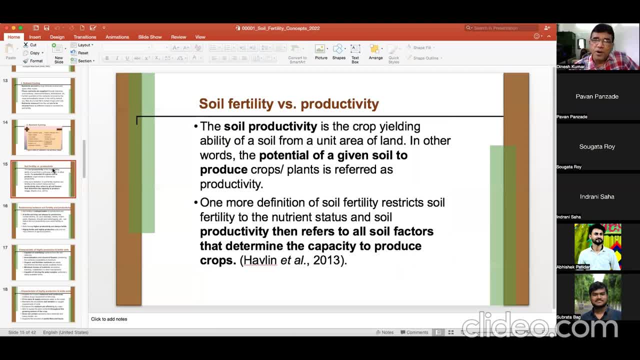 crop yielding ability of a soil from a unit area of land. unit area of land. unit area of land. means per unit area. how much is produced? means per unit area. how much is produced: means per unit area. how much is produced, in other words, potential of a given soil. 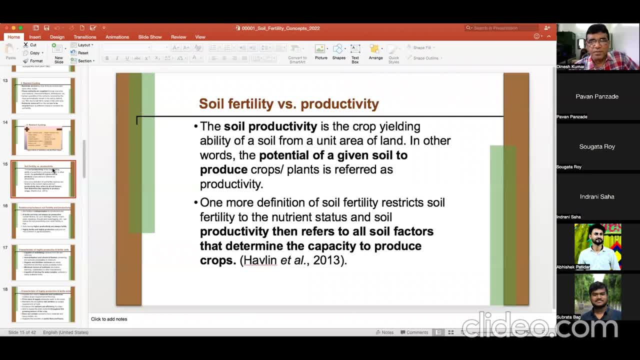 in other words, potential of a given soil. in other words, potential of a given soil to produce crops or plants is referred as to produce crops or plants. is referred as to produce crops or plants. is referred as productive, productive. productive statistics. soil fertility to the nutrient statistics. soil fertility to the nutrient. 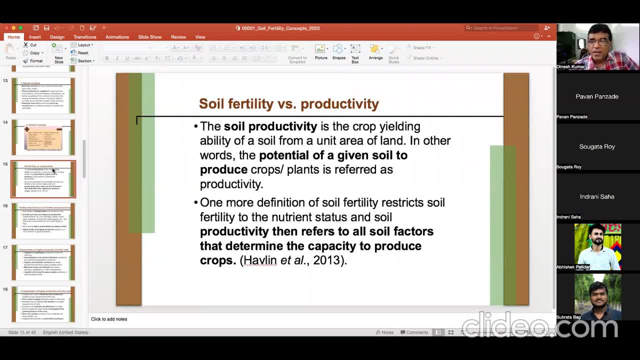 statistics: soil fertility to the nutrient status, status, status and soil productivity then refers to all and soil productivity then refers to all and soil productivity then refers to all. soil factors, soil factors, soil factors: that determines the capacity to produce, that determines the capacity to produce, that determines the capacity to produce crops. so here, 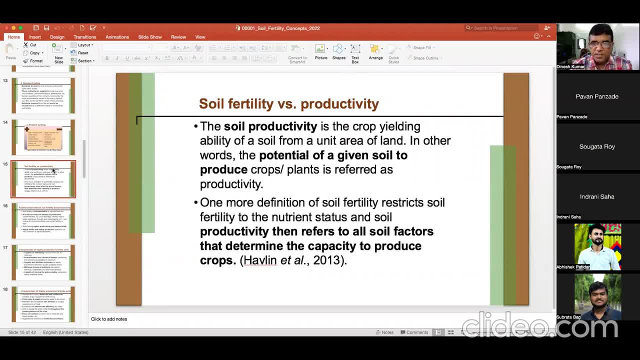 crops, so here. crops, so here one more definition. this is suggested by one more definition. this is suggested by one more definition. this is suggested by harvey, harvey, harvey. it is dale book, i think you already have. it is dale book, i think you already have. 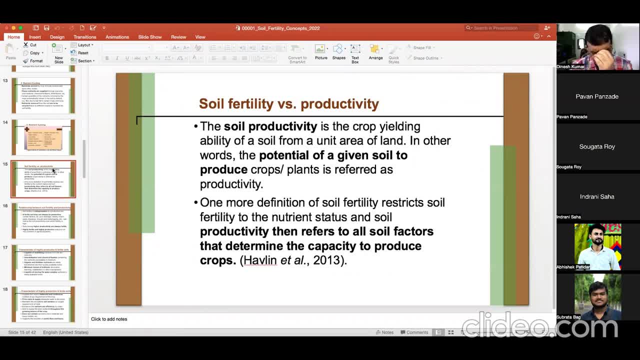 it is dale book. i think you already have this. no, no, sorry. this is this, no, no, sorry. this is this, no, no, sorry. this is probably. yeah, it is one more definition of soil fertility. one more definition of soil fertility. one more definition of soil fertility restricts soil fertility to the 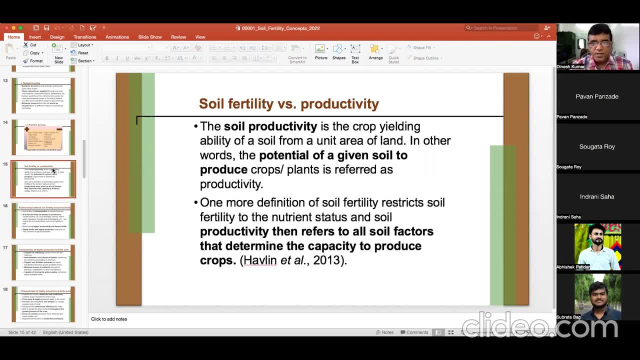 restricts soil fertility to the restricts soil fertility to the nutrient status. nutrient status, nutrient status and soil productivity then refers to and soil productivity then refers to, and soil productivity then refers to all soil factors that determine the all soil factors that determine the all soil factors that determine the capacity to produce problems howling in. 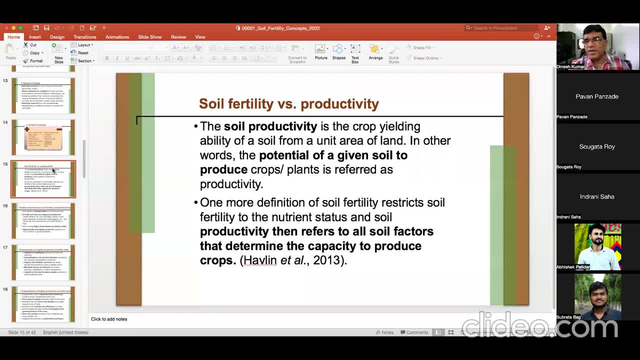 capacity to produce problems howling in capacity to produce problems howling in general. do not recognize general. do not recognize general. do not recognize differences in soil fertility and differences in soil fertility and differences in soil fertility and productivity, productivity, productivity. there are many more scientists who do not. 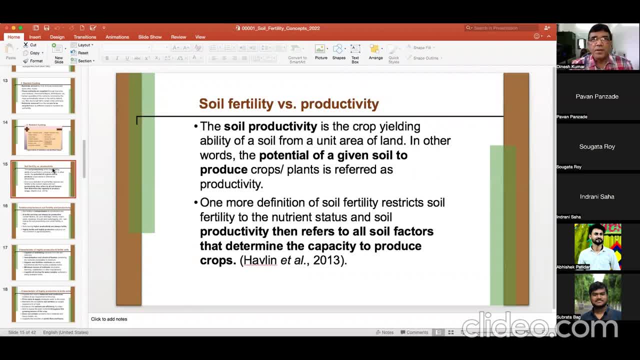 there are many more scientists who do not. there are many more scientists who do not make a difference in make a difference in make a difference in soil fertility and productivity. it is soil, fertility and productivity. it is soil fertility and productivity. it is mostly in india, mostly in india. 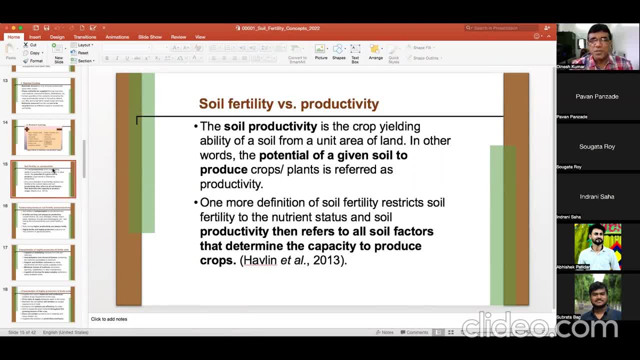 mostly in india- that people are very much worried about that. people are very much worried about that. people are very much worried about these two things. whenever you are in these two things, whenever you are in these two things, whenever you are in interview, interview, interview students are in interview. they 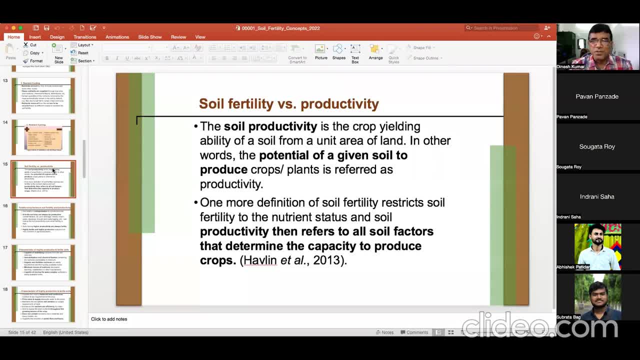 students are in interview. they students are in interview. they repeatedly ask this repeatedly, ask this repeatedly, ask this unwanted question: soil fertility- unwanted question. soil fertility- unwanted question. soil fertility, productivity, productivity, productivity- normally to be very frank and very normally to be very frank and very normally to be very frank and very clear. there is hardly any difference in 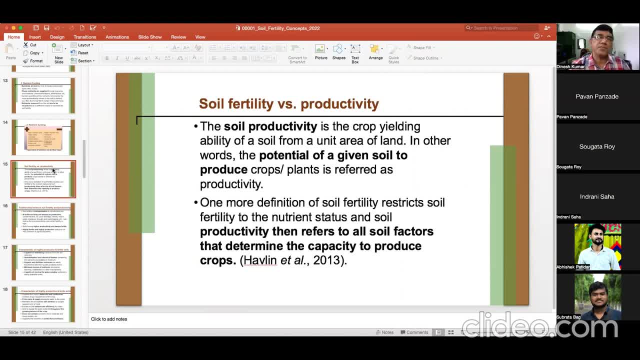 clear. there is hardly any difference in clear. there is hardly any difference in soil fertility and productivity, soil fertility and productivity. soil fertility and productivity. we have made some differences artificial. we have made some differences artificial. we have made some differences, artificial differences, differences, differences in soil fertility and productivity, if you try. 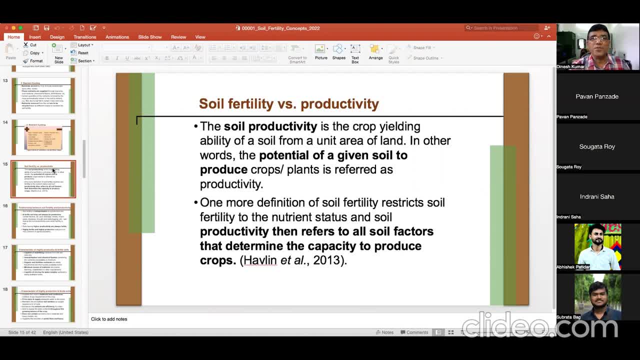 in soil fertility and productivity. if you try in soil fertility and productivity, if you try to get more knowledge, deep knowledge in to get more knowledge, deep knowledge in to get more knowledge, deep knowledge in this subject, then you will find this subject, then you will find this subject. then you will find very little, or rather no difference in. 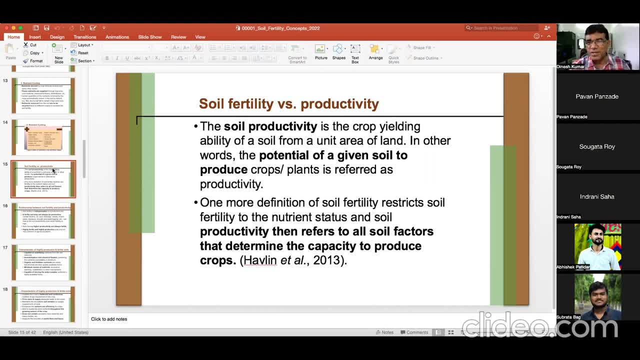 very little, or rather no difference in very little, or rather no difference in soil fertility and productivity, soil fertility and productivity. soil fertility and productivity. i don't want to prove it here, but i don't want to prove it here, but i don't want to prove it here. but you, you can remember. but to satisfy, 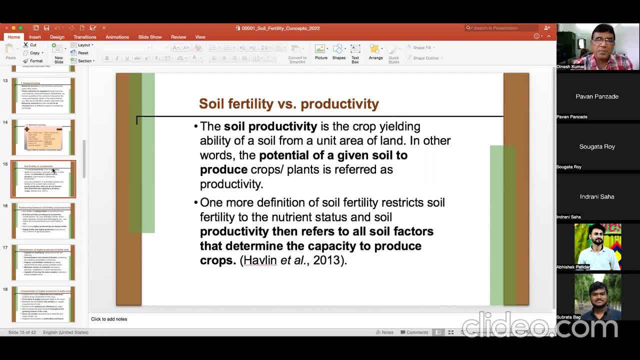 you, you can remember. but to satisfy you, you can remember. but to satisfy the people who ask a question, you need the people who ask a question. you need the people who ask a question. you need to say yes, sir, to say yes, sir, to say yes, sir, there is difference in soil fertility and 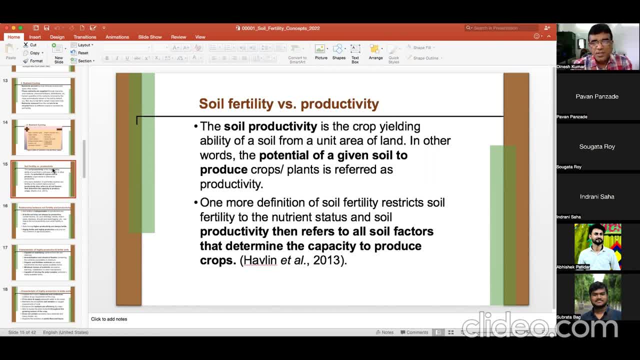 there is difference in soil fertility and there is difference in soil fertility and productivity, and there are two different productivity and there are two different productivity and there are two different things, things, things. so therefore, this thing is written here. so therefore, this thing is written here. so therefore, this thing is written here by harvey. 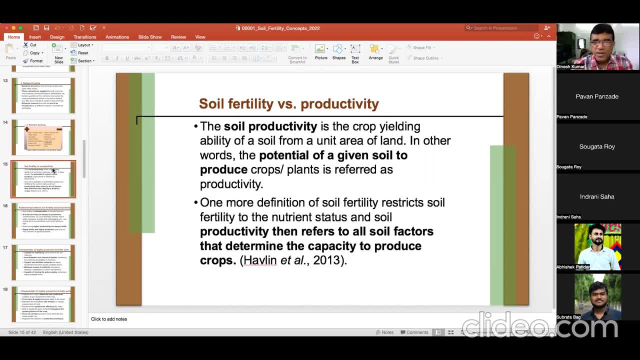 by harvey by harvey. one more definition of soil fertility. one more definition of soil fertility. one more definition of soil fertility. restricts soil fertility to the nuclear. restricts soil fertility to the nuclear. restricts soil fertility to the nuclear status. and soil productivity status and soil productivity. 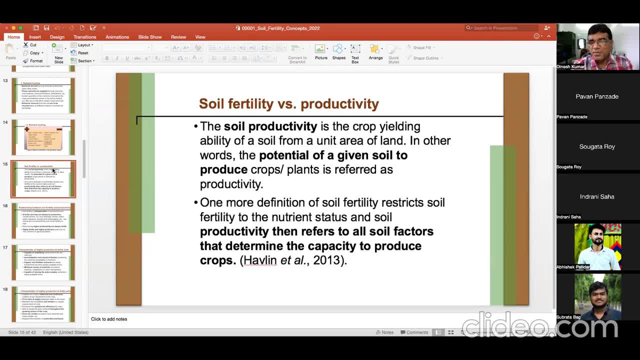 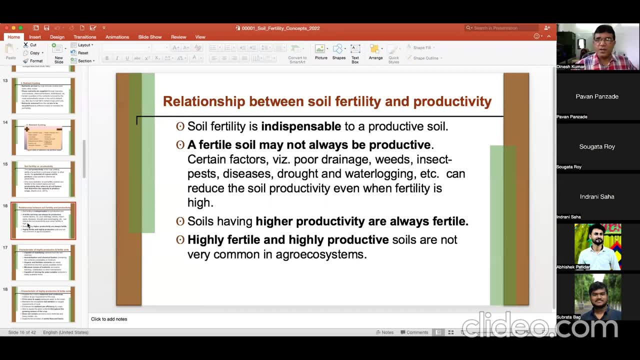 status and soil productivity. then refers to all soil factors. that then refers to all soil factors. that then refers to all soil factors that determine the capacity to produce. so, relationship between so. relationship between so. relationship between soil fertility and productivity, so as a. soil fertility and productivity, so as a. 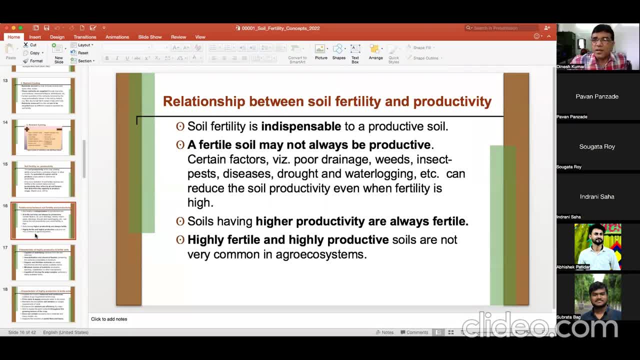 soil, fertility and productivity, so as a fertility and productivity, both are fertility and productivity. both are fertility and productivity. both are different and there are differences different and there are differences different and there are differences. already you know the differences in there. already you know the differences in there. 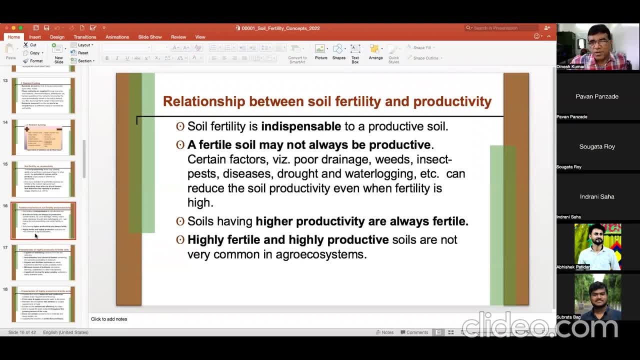 already. you know the differences in there. so soil: fertility is indispensable to a so soil. fertility is indispensable to a so soil. fertility is indispensable to a productive soil. productive soil, productive soil. if you want highly productive soil, then if you want highly productive soil, then if you want highly productive soil, then you should have highly fertilized. 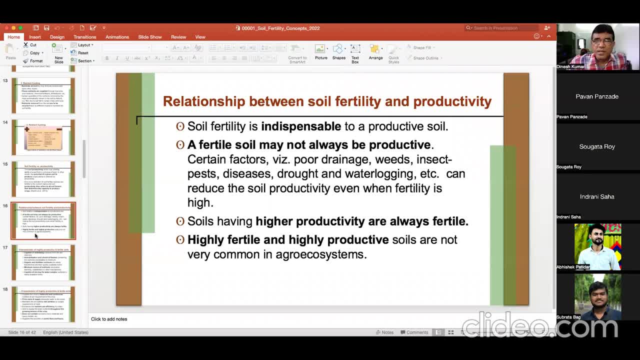 you should have highly fertilized. you should have highly fertilized. a fertile soil may not always be productive. a fertile soil may not always be productive. a fertile soil may not always be productive. that is another point. okay, your soil is. that is another point. okay, your soil is. 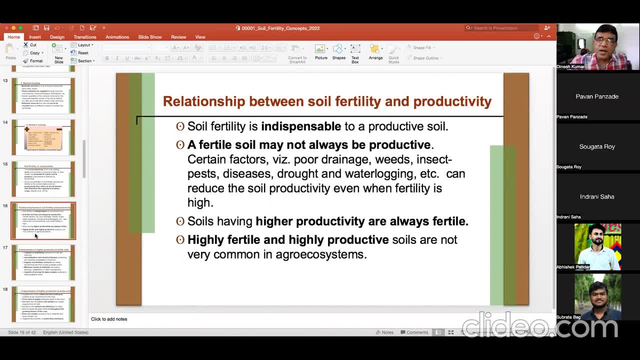 that is another point. okay, your soil is hard, highly fertile, but many times it hard. highly fertile, but many times it hard. highly fertile, but many times it may not be highly productive. a fertile may not be highly productive. a fertile may not be highly productive. a fertile soil may not be necessarily. 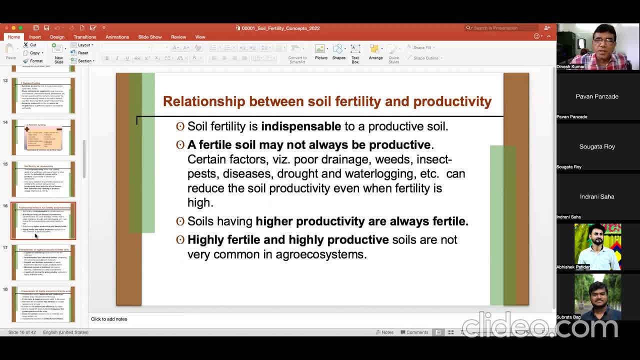 soil may not be necessarily. soil may not be necessarily productive. one productive, one productive one. how it can become fertile soil can become. how it can become fertile soil can become. how it can become fertile soil can become unproductive, less productive due to unproductive. less productive due to. 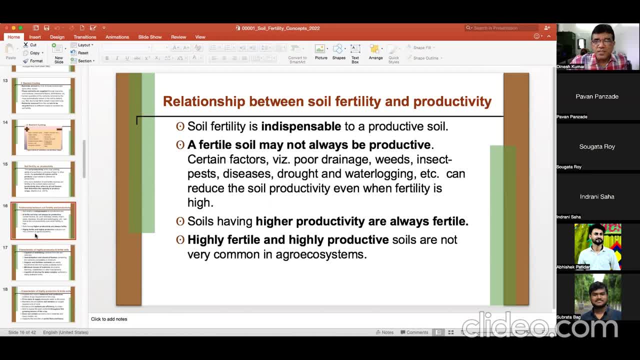 unproductive, less productive due to poor damage, poor damage. poor damage, weeds, insect pests, diseases, drought and weeds, insect pests, diseases, drought and weeds, insect pests, diseases, drought and water logging, water logging, water logging, etc. can reduce the soil productivity. these etc can reduce the soil productivity. these etc can reduce the soil productivity. these other factors, factors other than soil. 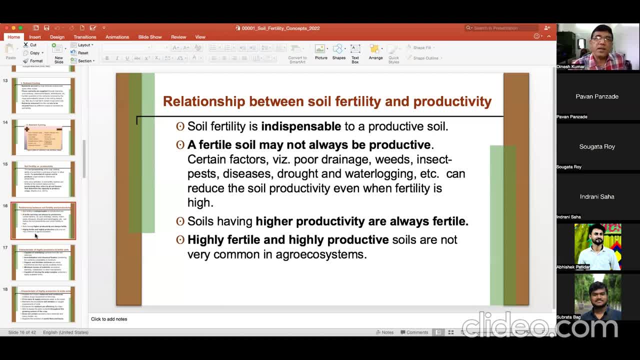 other factors. factors other than soil. other factors, factors other than soil: fertility, fertility: fertility will reduce the productivity will. can will reduce the productivity. will can will reduce the productivity will can can limit the productivity. can limit the productivity, can limit the productivity so as having higher productivity are. 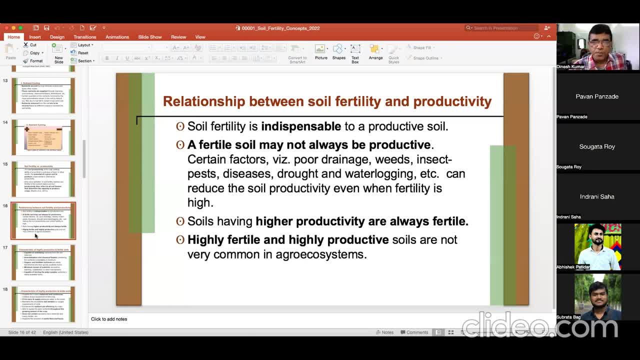 so as having higher productivity are so as having higher productivity are always fertile, always fertile, always fertile- this is true, this is true. highly fertile- this is true. this is true, this is true. highly fertile- this is true, this is true. highly fertile and highly productive soils are not very 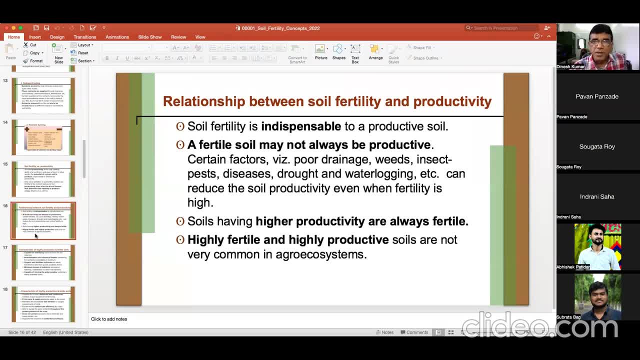 and highly productive soils are not very and highly productive soils are not very common, common, common in agro ecosystem. so you need to remember in agro ecosystem. so you need to remember in agro ecosystem. so you need to remember all these four points tomorrow, if you. 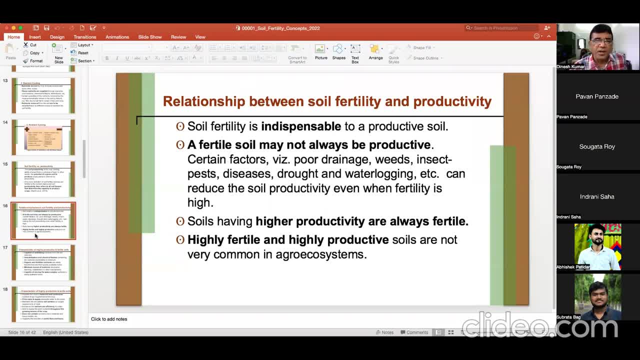 all these four points tomorrow, if you, all these four points tomorrow, if you are sitting in any interview, any exam, are sitting in any interview, any exam, are sitting in any interview, any exam. if you are not able to answer, you cannot. if you are not able to answer, you cannot. 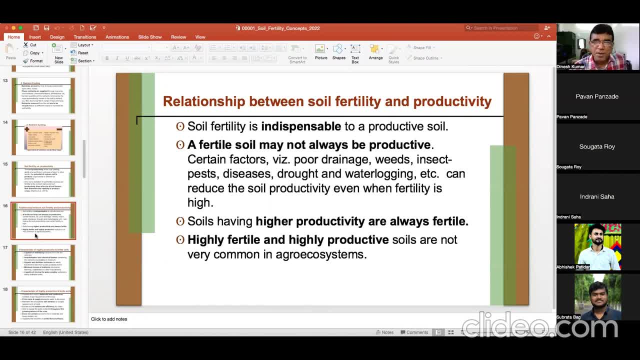 if you are not able to answer, you cannot question the teacher. that we were not question the teacher, that we were not question the teacher, that we were not taught, taught, taught. so please do remember these four points. so please do remember these four points. so please do remember these four points. a lot of people still discuss this. 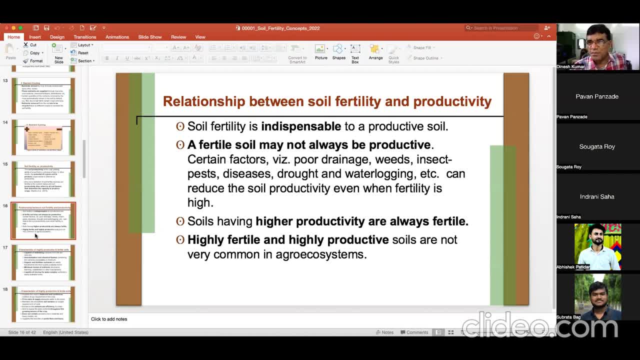 a lot of people still discuss this. a lot of people still discuss this irrelevant issue. irrelevant issue, irrelevant issue. so you need to prepare yourself to answer. so you need to prepare yourself to answer. so you need to prepare yourself to answer this very irrelevant issue, this very irrelevant issue. 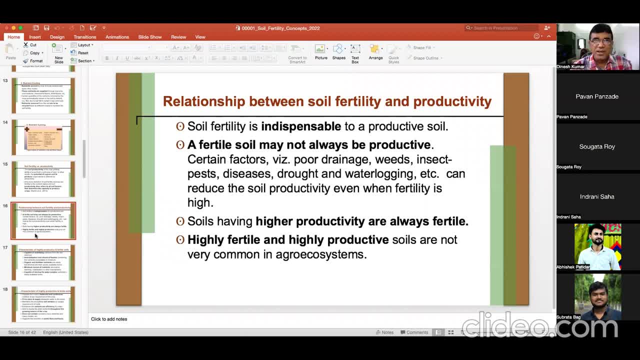 this very irrelevant issue. anyway, this is, in my view, irrelevant, but anyway, this is in my view, irrelevant. but anyway, this is in my view irrelevant, but maybe very relevant to people who ask, maybe very relevant to people who ask, maybe very relevant to people who ask that question because it is the simplest. 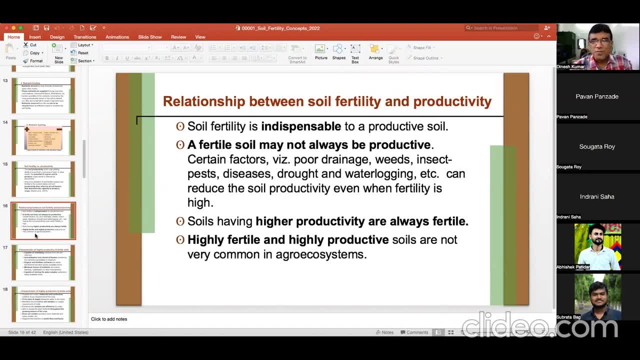 that question because it is the simplest, that question, because it is the simplest question. anybody can ask question. anybody can ask question, anybody can ask. so you see, first thing is so. you see, first thing is so. you see, first thing is that soil fertility is in this, that soil fertility is in this. 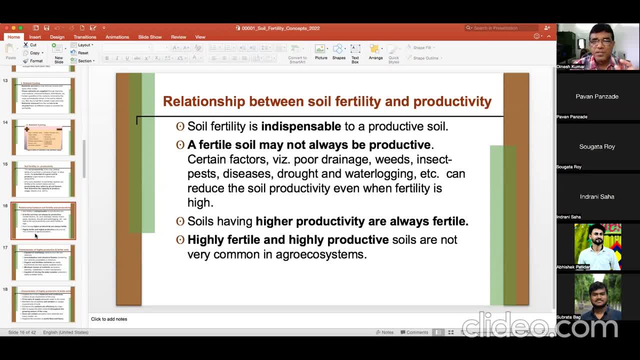 that soil fertility is, in this, indispensable to a productive soil, indispensable to a productive soil, indispensable to a productive soil. indispensable means, it is a must. indispensable means, it is a must. indispensable means, it is a must, it is a must. soil fertility is must, it is a must. soil fertility is must. 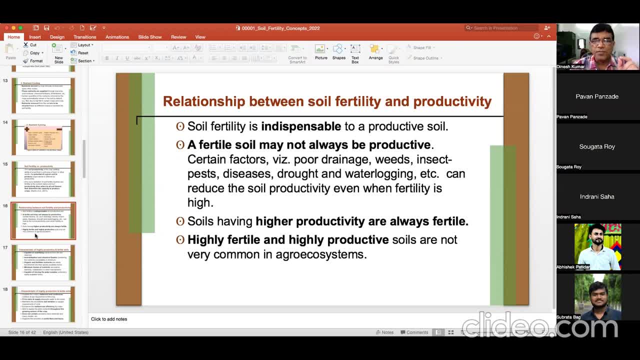 it is a must, soil fertility is must to have a productive soil, to have a productive soil, to have a productive soil. so, therefore, a fertile soil may not, so, therefore, a fertile soil may not. so, therefore, a fertile soil may not always, always, always. another point is: a fertile soil may. 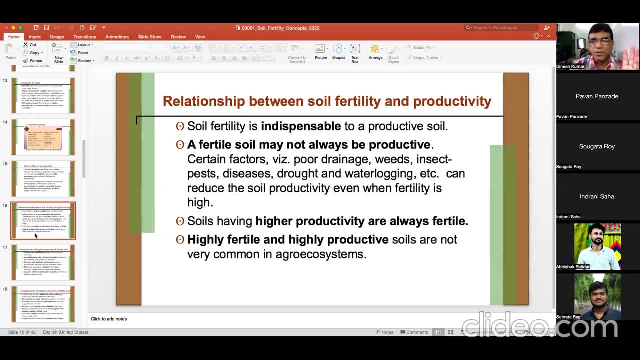 another point is: a fertile soil may not be always productive. soil is having not be always productive. soil is having not be always productive. soil is having good status of nutrients, but still it is good status of nutrients but still it is good status of nutrients, but still it is not producing good crops. maybe because 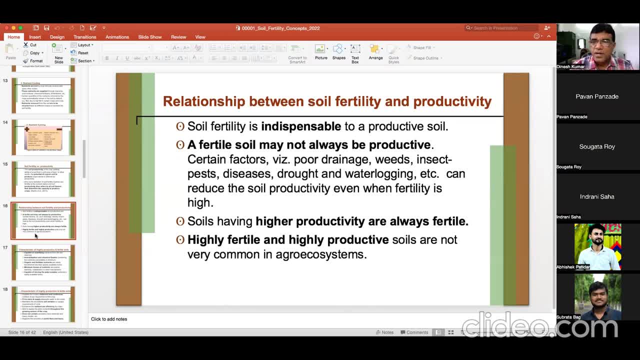 not producing good crops. maybe because not producing good crops, maybe because of limitation of other factors, of limitation of other factors, of limitation of other factors like poor drainage, weeds insect-based, like poor drainage weeds insect-based, like poor drainage, weeds, insect-based, disease etc. disease etc, disease etc. third point is soils having high. 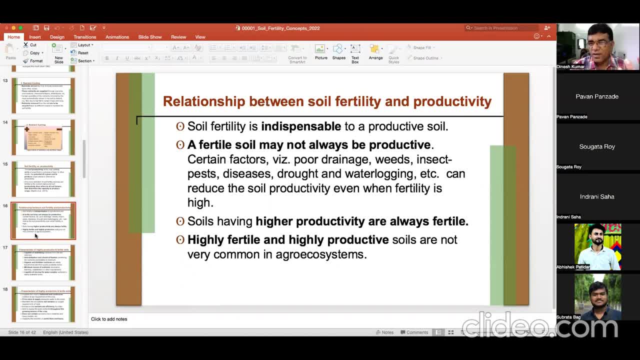 third point is soils having high. third point is soils having high productivity. must are always highly productivity. must are always highly productivity, must are always highly fertile, fertile. fertile are fertile because you cannot have higher. are fertile because you cannot have higher are fertile because you cannot have higher productivity. first condition is that soil 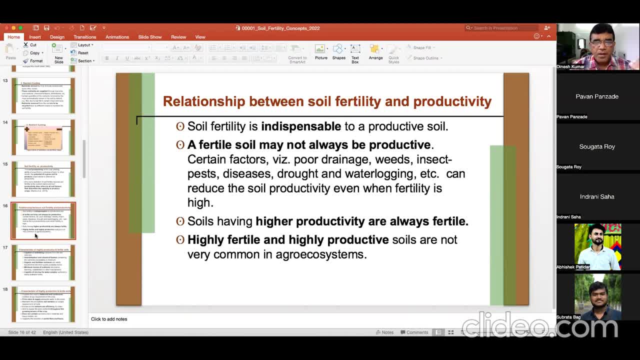 productivity first condition is that soil productivity first condition is that soil should be fertile, then comes the other. should be fertile, then comes the other should be fertile, then comes the other factors, factors, factors: highly fertile and highly productive: highly fertile and highly productive, highly fertile and highly productive soils are 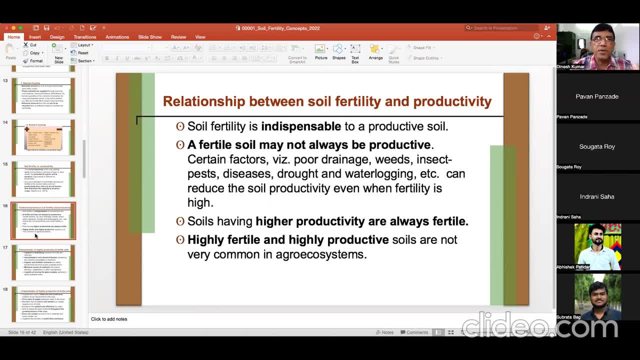 soils are. soils are not very common in agricultural systems, not very common in agricultural systems, not very common in agricultural systems. they are not common that you can have. they are not common that you can have. they are not common that you can have very high fertility soil, which is highly 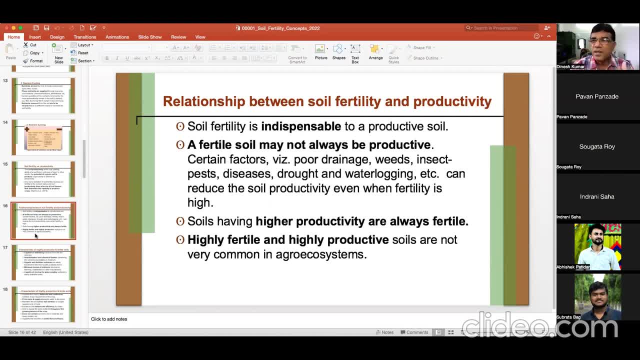 very high fertility soil which is highly very high fertility soil, which is highly productive. so it is there, but very productive. so it is there, but very productive. so it is there, but very limited area. we have such kind of soil. limited area, we have such kind of soil. 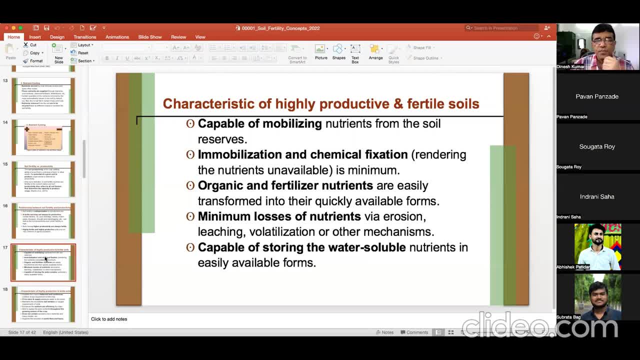 limited area. we have such kind of soil which are highly fertile and highly, which are highly fertile and highly, which are highly fertile and highly productive, productive productive now. characteristics of highly productive now. characteristics of highly productive, now characteristics of highly productive and fertile. just now we have seen 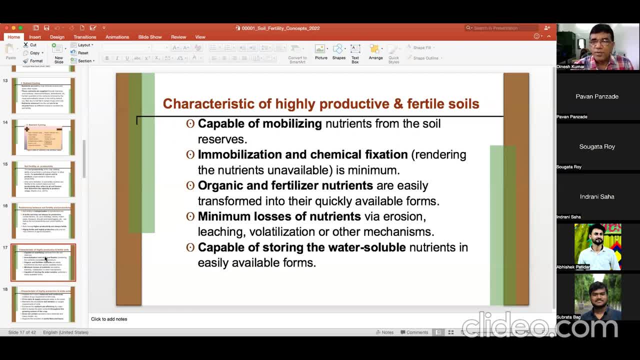 and fertile. just now we have seen- and fertile. just now we have seen- that the soil which is highly productive, that the soil which is highly productive, that the soil which is highly productive and highly and highly and highly fertile may not be found in agricultural. fertile may not be found in agricultural. 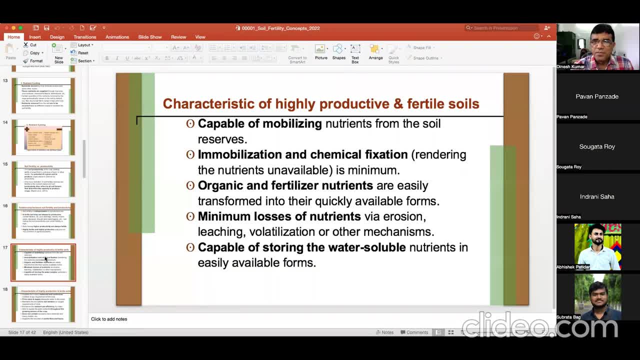 fertile may not be found in agricultural system system. system means our artificial system. it is rare to means our artificial system. it is rare to means our artificial system. it is rare to find, find, find, but if you found. if you found, then what? but if you found. if you found, then what? 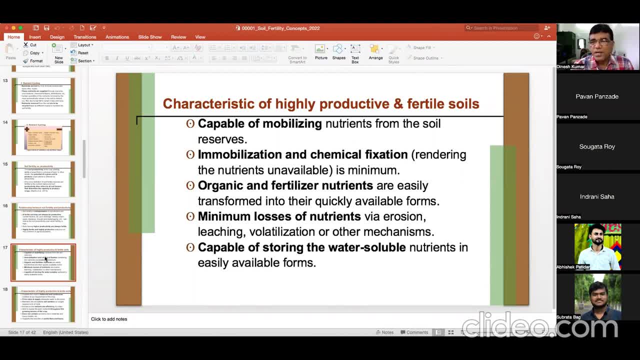 but if you found, if you found, then what should be the characteristics of, should be the characteristics of, should be the characteristics of highly productive and highly fertile. highly productive and highly fertile, number one: it is capable of mobilizing. number one: it is capable of mobilizing number one: it is capable of mobilizing nutrients from the soil reserves. 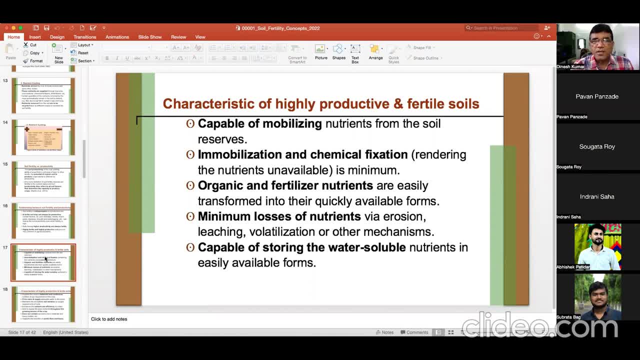 nutrients from the soil reserves. nutrients from the soil reserves. the soil reserves can be a cook and the soil reserves can be a cook and the soil reserves can be a cook, and inorganic and organic. so you should have inorganic and organic. so you should have inorganic and organic, so you should have capacity to get the nutrients released. 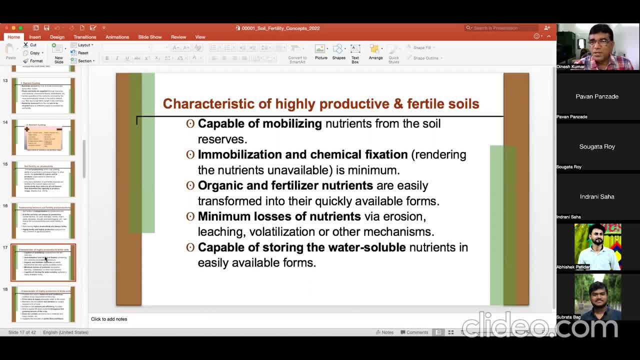 capacity to get the nutrients released, capacity to get the nutrients released from the results, from the results, from the results. it should not get more fixation of the. it should not get more fixation of the. it should not get more fixation of the nutrients, nutrients, nutrients. it should supply the nutrients as per. 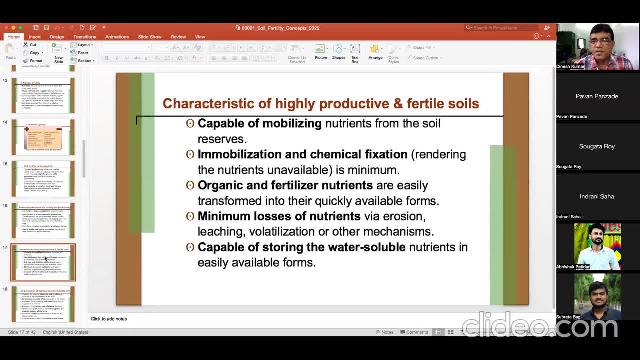 it should supply the nutrients as per. it should supply the nutrients as per demand. demand, demand, immobilization and chemical fixation. immobilization and chemical fixation. immobilization and chemical fixation. it renders the nutrients unavailable. it it renders the nutrients unavailable. it it renders the nutrients unavailable. it should be minimal. there should not be. 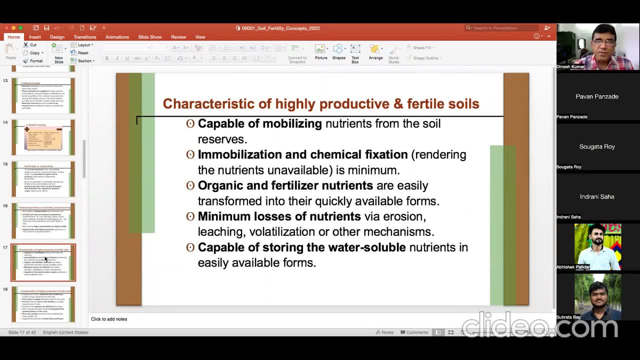 should be minimal. there should not be, should be minimal. there should not be too much of immobilization so that too much of immobilization, so that too much of immobilization so that nutrients become unavailable, or there nutrients become unavailable, or there nutrients become unavailable, or there should not be chemical fixation, then 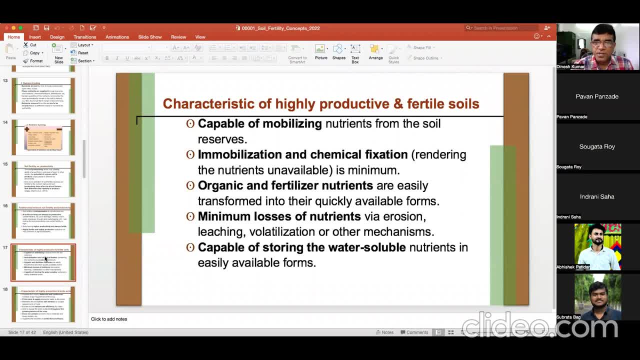 should not be chemical fixation, then should not be chemical fixation, then only you can have, only you can have, only you can have a higher status of available nutrients. a higher status of available nutrients, a higher status of available nutrients. organic and fertilizer nutrients are organic and fertilizer nutrients are. 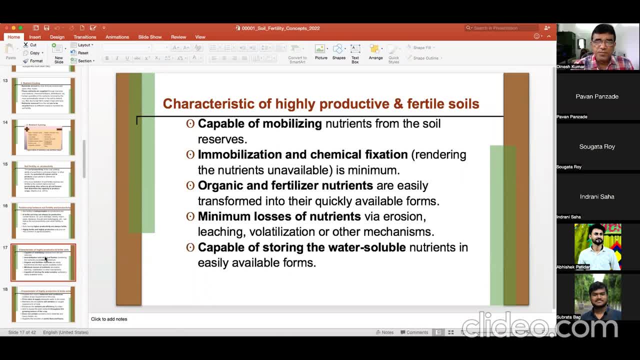 organic and fertilizer nutrients are easily transformed quickly into available. easily transformed quickly into available. easily transformed quickly into available nutrients. if you apply fertilizers or nutrients, if you apply fertilizers or nutrients, if you apply fertilizers or manure, they should be converted into manure. they should be converted into. 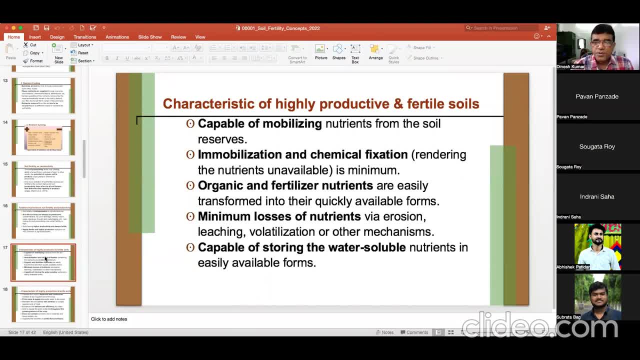 manure. they should be converted into easily available forms. easily available forms. easily available forms. minimum losses of nutrients. a soil which minimum losses of nutrients, a soil which minimum losses of nutrients. a soil which is productive and fertile. they should is productive and fertile. they should is productive and fertile. they should have minimum losses of nutrients. if you 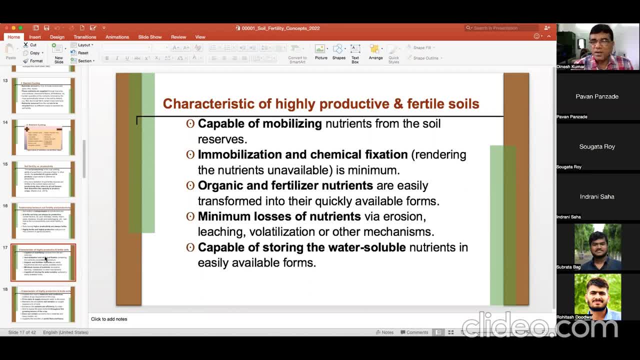 have minimum losses of nutrients. if you have minimum losses of nutrients, if you have high losses of nutrients, it will not have high losses of nutrients. it will not have high losses of nutrients. it will not remain highly fertile, remain highly fertile. remain highly fertile, capable of restoring the water soluble. 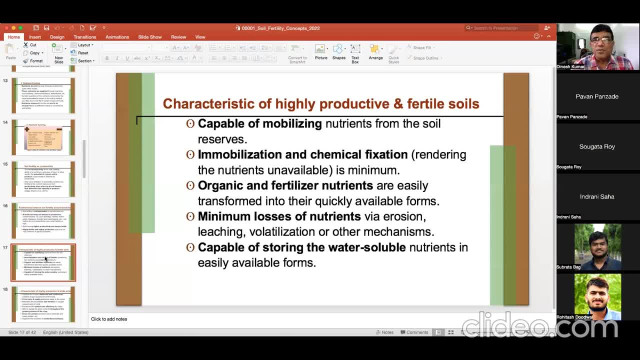 capable of restoring the water soluble, capable of restoring the water soluble nutrients. soil should not soil should be nutrients. soil should not. soil should be nutrients. soil should not. soil should be such which allows minimum losses of the, such which allows minimum losses of the, such which allows minimum losses of the nutrients from, from the, from it. 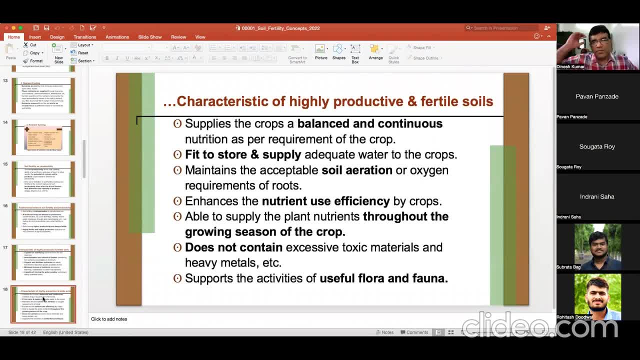 nutrients from from the from it, nutrients from from the from it. so so, so you can have some more characteristics of, you can have some more characteristics of, you can have some more characteristics of highly productive and fertile soil. it highly productive and fertile soil. it highly productive and fertile soil. it supplies the crops a balanced and 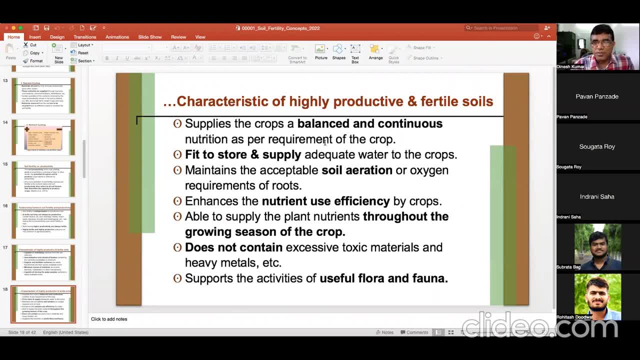 supplies the crops a balanced and supplies the crops a balanced and continuous nutrition, as per requirement of continuous nutrition, as per requirement of continuous nutrition, as per requirement of the crops, the crops, the crops fit to store and supply adequate water, fit to store and supply adequate water, fit to store and supply adequate water to the crops. this is also important- fit. 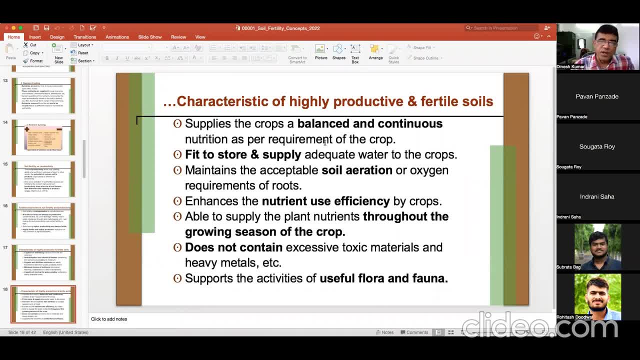 to the crops. this is also important. fit to the crops. this is also important. fit to store. it should have capacity to to store. it should have capacity to to store. it should have capacity to store water and supply adequate water to store water and supply adequate water to. 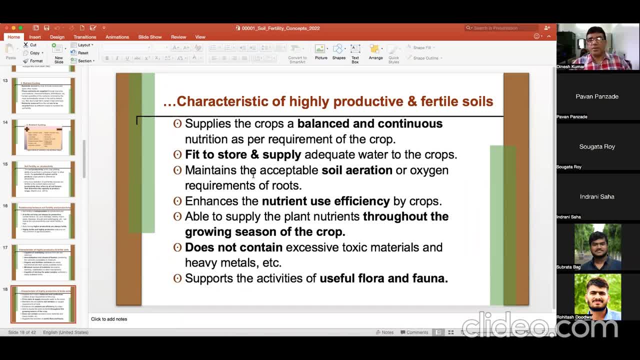 store water and supply adequate water to the crops, the crops, the crops- maintains the acceptable soil erasure or maintains the acceptable soil erasure, or maintains the acceptable soil erasure or oxygen requirement of foods. so aeration. oxygen requirement of foods, so aeration. oxygen requirement of foods, so aeration is needed for making nutrients available. 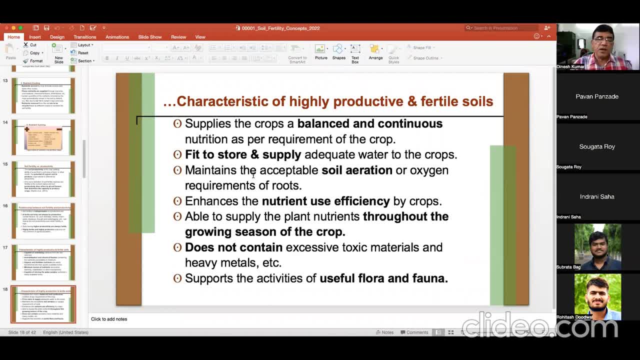 is needed for making nutrients available, is needed for making nutrients available, as well as for microbial activity and as well as for microbial activity and as well as for microbial activity and other activities also for plant foods. you other activities also for plant foods, you other activities also for plant foods. you need oxygen. 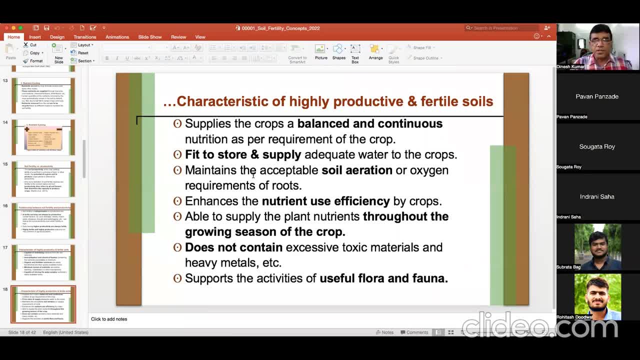 need oxygen. need oxygen. announces the nutrient use absentee by. announces the nutrient use absentee by. announces the nutrient use absentee by crops able to supply the plant nutrients. crops able to supply the plant nutrients. crops able to supply the plant nutrients. throughout the growing season of the. throughout the growing season of the. 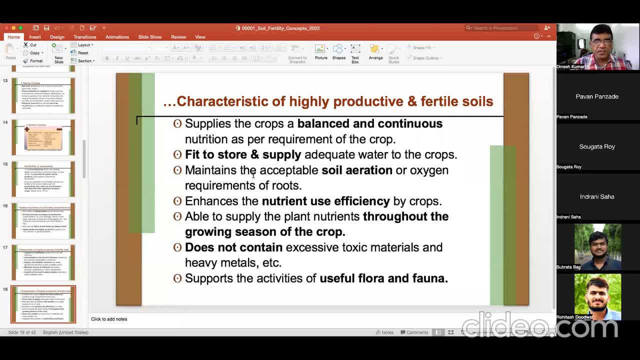 throughout the growing season of the crop. does not contain excessive toxic crop. does not contain excessive toxic crop. does not contain excessive toxic materials and heavy metals. supports the materials and heavy metals. supports the materials and heavy metals. supports the activities of useful flora and fauna. activities of useful flora and fauna. 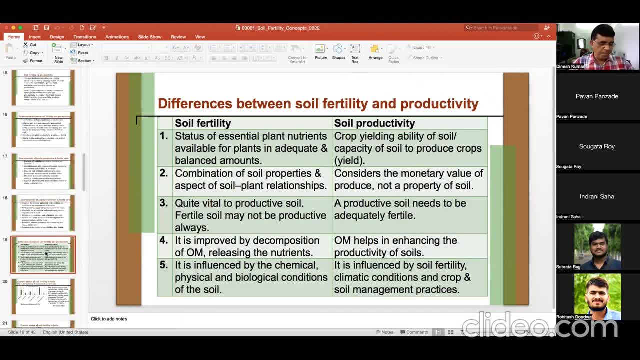 activities of useful flora and fauna. so these are some of the characteristics. so these are some of the characteristics. so these are some of the characteristics. uh, uh, uh. now, the last slide for today is now the last slide for today is now. the last slide for today is differences between soil fertility and 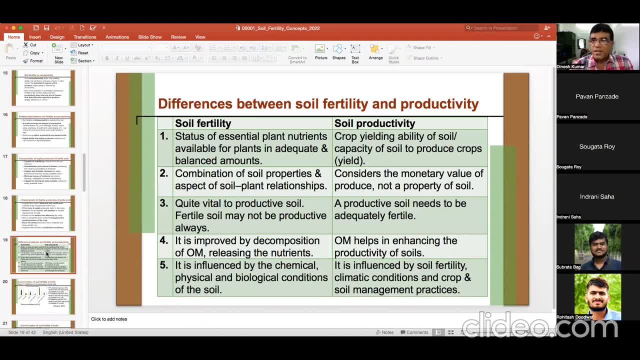 differences between soil fertility and differences between soil fertility and productivity: productivity, productivity, so soil fertility, these are very uh. so soil fertility, these are very uh. so soil fertility. these are very uh, man-made, man-made, man-made differences, differences, differences, uh. however, they are not genuinely the uh. however, they are not genuinely the. 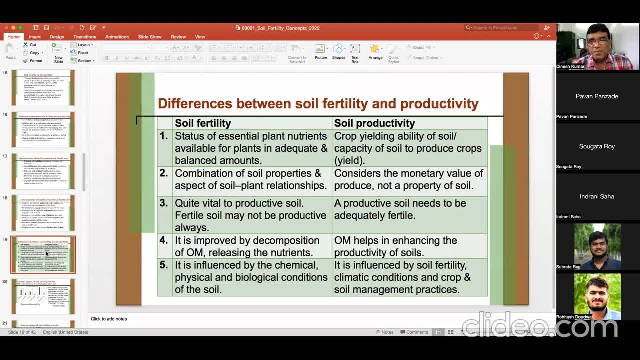 uh, however, they are not genuinely the differences anyway. differences, anyway, differences anyway. if because in your exam it can come any, if because in your exam it can come any, if because in your exam it can come any. exam in your life in soil fertility, exam in your life in soil, fertility. 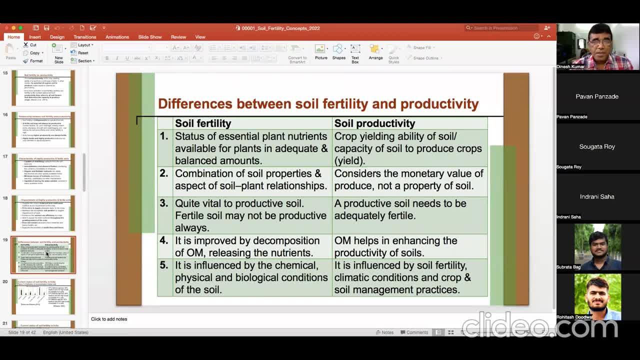 exam in your life in soil fertility. such questions can come, however they are. such questions can come, however they are. such questions can come. however, they are irrelevant. irrelevant relevant. soil fertility and soil productivity. soil fertility and soil productivity. soil fertility and soil productivity: difference, difference, difference. the status of essential plant nutrients. 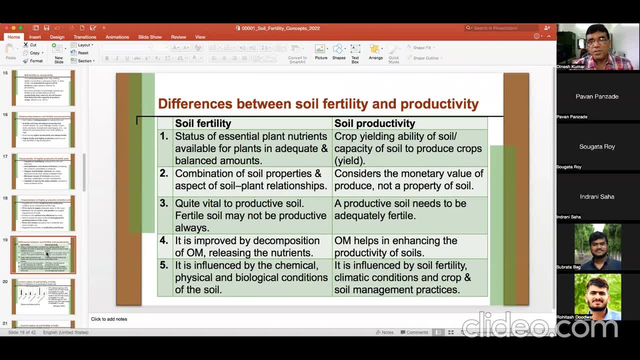 the status of essential plant nutrients, the status of essential plant nutrients available for plants in adequate and available for plants in adequate and available for plants in adequate and balanced amount. so this is the definition: balanced amount. so this is the definition, balanced amount. so this is the definition of soil fertility. you can write any. 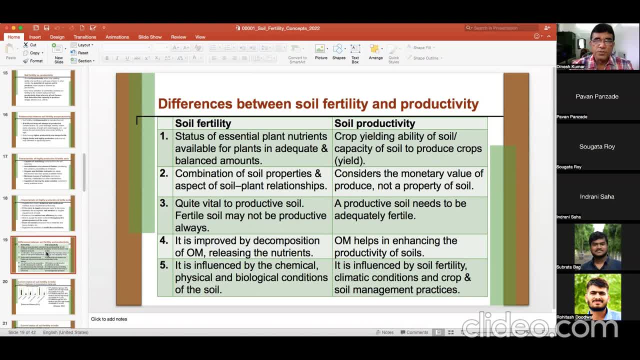 of soil fertility. you can write any of soil fertility. you can write any definition of soil fertility here. definition of soil fertility: here. definition of soil fertility here. on the right side, it is soil productivity. on the right side it is soil productivity. on the right side it is soil productivity. this is pro yielding ability of soil. or. 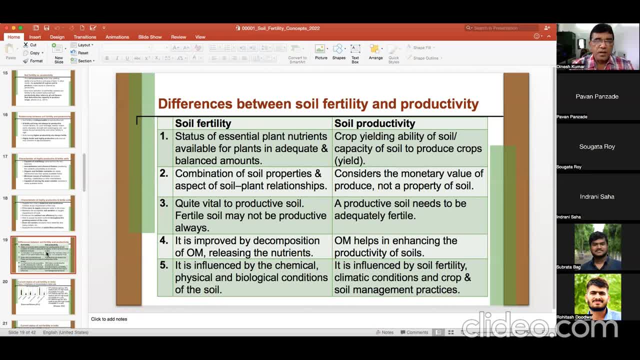 this is pro yielding ability of soil or this is pro yielding ability of soil or capacity of soil to produce crops. capacity of soil to produce crops. capacity of soil to produce crops- uh combination of soil properties and uh combination of soil properties and uh combination of soil properties. and aspect of soil plant relationship- soil- 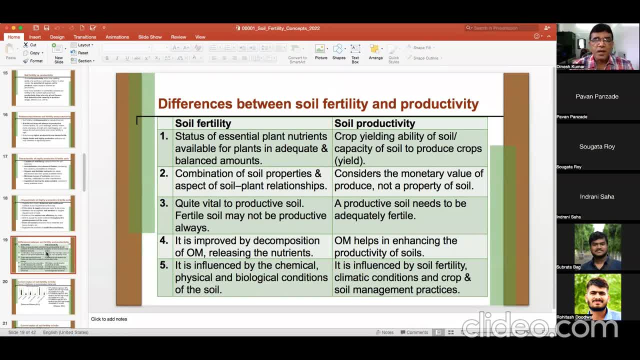 aspect of soil plant relationship. soil aspect of soil plant relationship. soil fertility: combination of mostly soil fertility, combination of mostly soil fertility, combination of mostly soil properties. properties: properties govern the soil for trade. however, here govern the soil for trade. however, here govern the soil for trade. however, here there are number of. 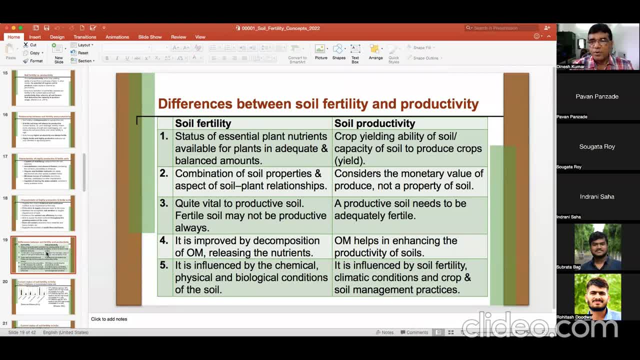 there are number of, there are number of uh factors. consider the monetary value. uh factors consider the monetary value. uh factors consider the monetary value of produce, of produce, of produce not a property of the sun. it is not a not a property of the sun. it is not a. 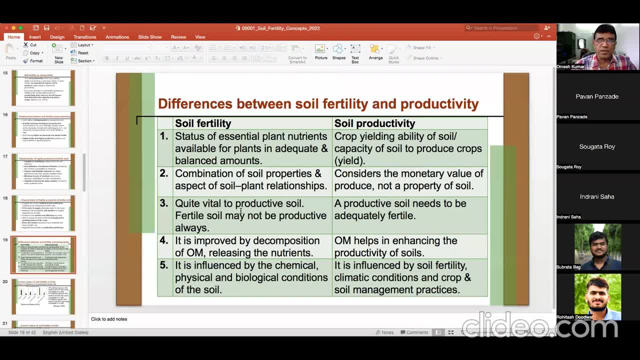 not a property of the sun, it is not a property of the soil, property of the soil, property of the soil, quite wider to productive soils, fertile, quite wider to productive soils fertile, quite wider to productive soils. fertile soil may not be productive. a productive soil may not be productive. 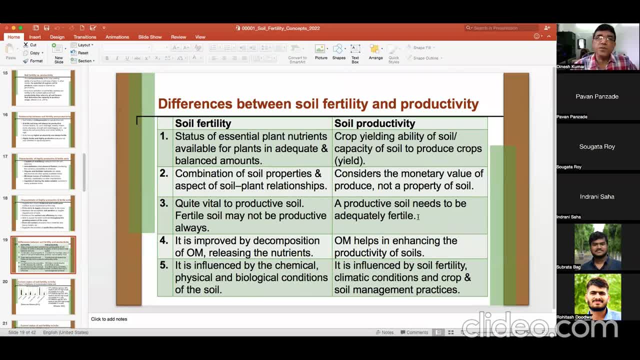 a productive soil may not be productive. a productive soil needs to be adequately. a productive soil needs to be adequately. a productive soil needs to be adequately fertile or need to be fertile- this fertile or need to be fertile, this fertile or need to be fertile. this, these two lines you must remember. 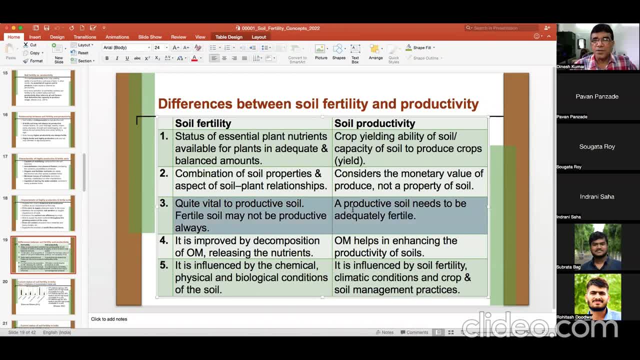 these two lines. you must remember these two lines. you must remember tomorrow, if any confusion is there, and tomorrow, if any confusion is there, and tomorrow if any confusion is there and you are not able to answer this question, you are not able to answer this question, you are not able to answer this question, then i i may not be blamed for it. that 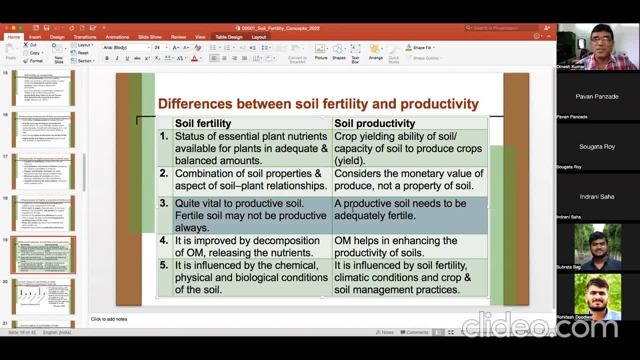 then i, i may not be blamed for it. that then i, i may not be blamed for it- that you were not taught, you were not taught, you were not taught. so they are very simple points. remember so they are very simple points. remember. so they are very simple points. remember, i have seen. 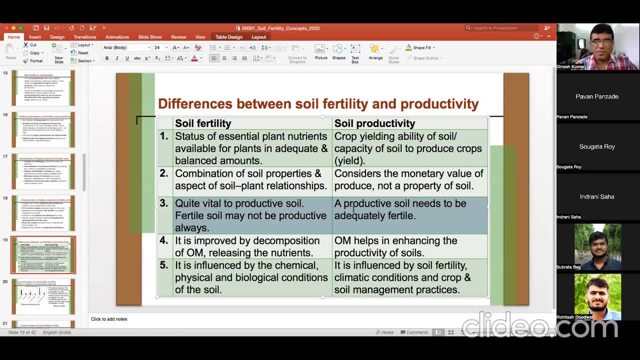 i have seen. i have seen very few strength can answer this. very few strength can answer this. very few strength can answer this simplest question. anyway, it is improved by decomposition of. anyway, it is improved by decomposition of. anyway, it is improved by decomposition of organic matter, releasing the nutrients. 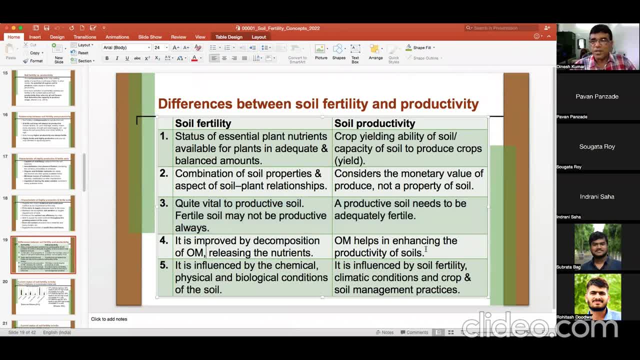 organic matter releasing the nutrients. organic matter releasing the nutrients: this one fertility. organic matter helps this one fertility. organic matter helps this one fertility. organic matter helps in enhancing the productivity of soils, in enhancing the productivity of soils, in enhancing the productivity of soils. it is influenced by the chemical. 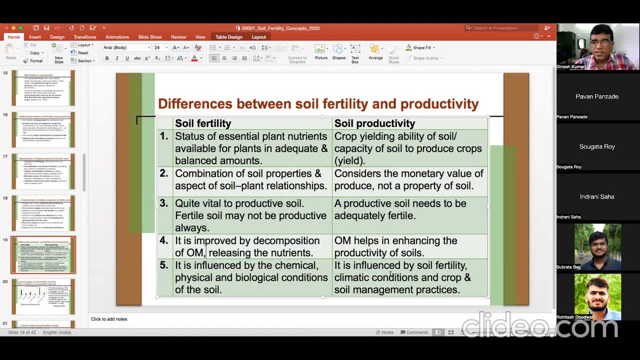 it is influenced by the chemical. it is influenced by the chemical physical biological properties of the physical biological properties, of the physical biological properties of the soil. productivity is influenced by soil. soil productivity is influenced by soil. soil productivity is influenced by soil fertility, plus all other fertility, plus all other.